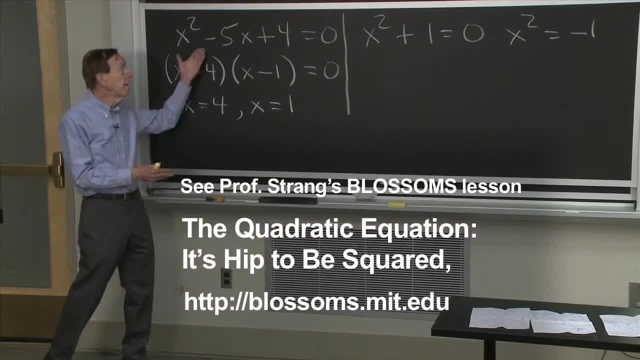 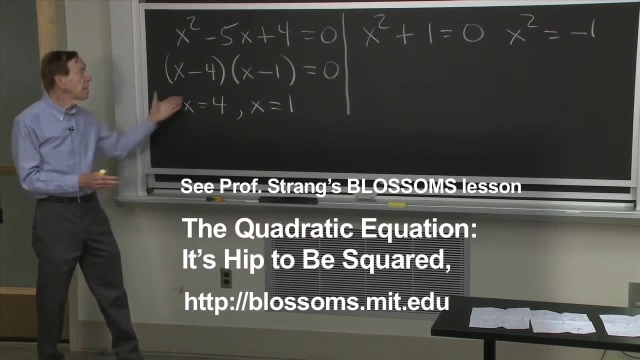 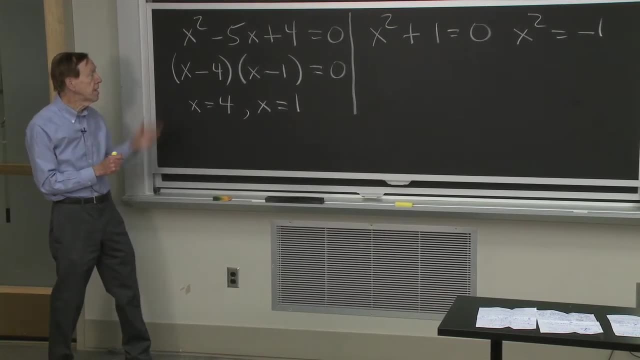 like that before quadratic equation And the nice way to solve it is to factor that into two pieces And then you can see: to make this piece 0, x equal 4 gives an answer. To make this piece 0, x equal 1 gives an answer. 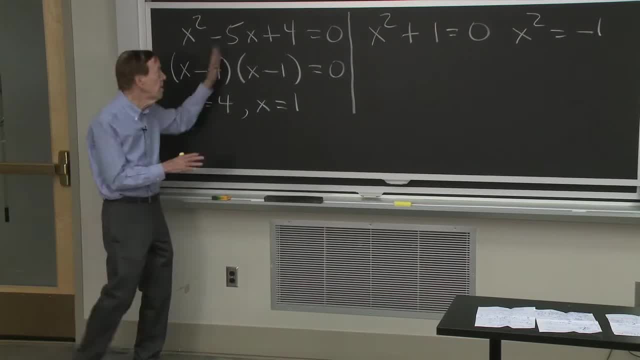 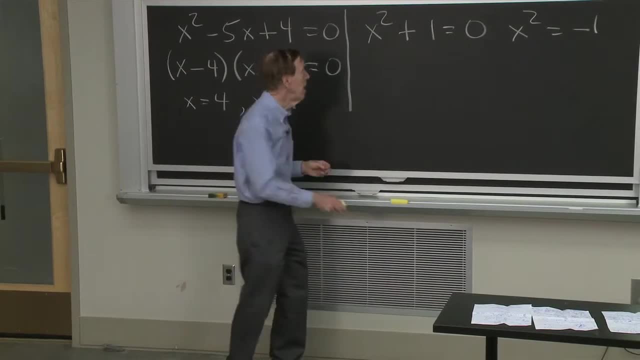 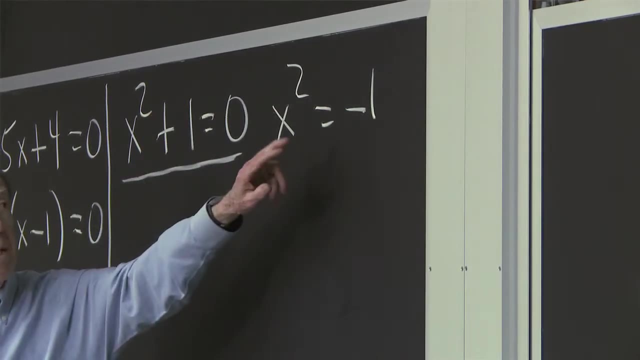 And we have the two solutions Straightforward, because that didn't involve complex numbers. Now let's get to an imaginary number. Suppose this was our equation: x squared plus 1 equals 0.. Or if I put the 1 on the other side, x squared equal minus 1.. 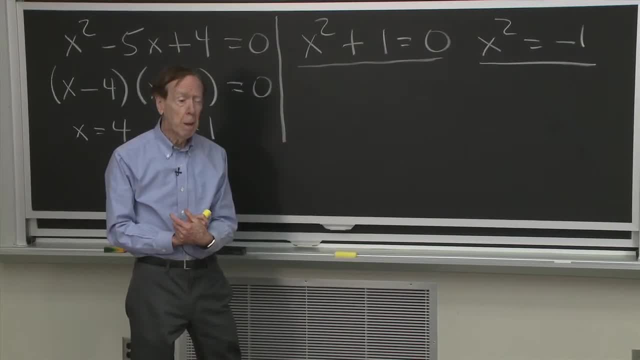 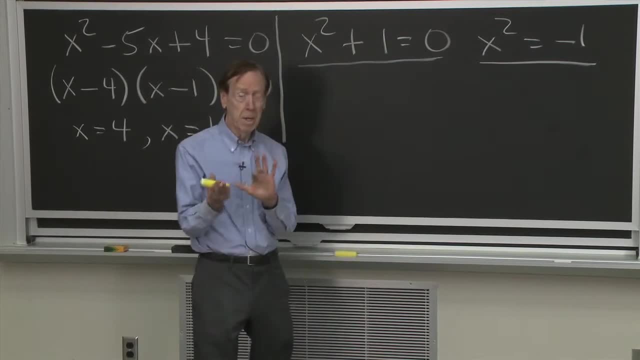 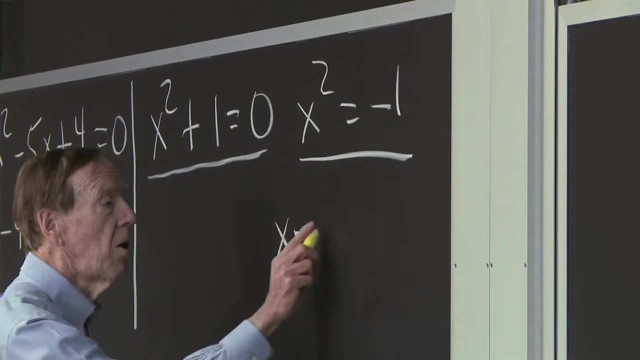 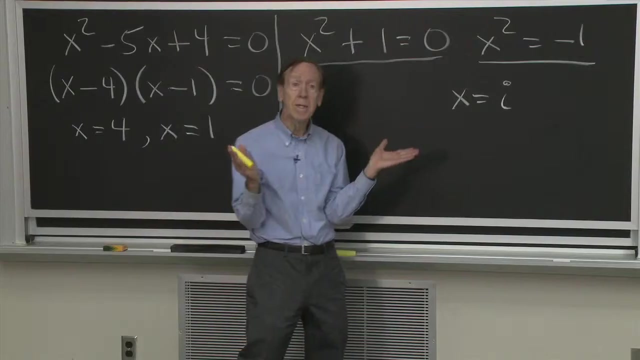 Well, no real solutions for that. So you can either stop, which is what people did for thousands of years, or invent an imaginary number that solves that equation. So that number is called i- i for imaginary, I guess. So i is just defined to be a number whose square is minus 1.. 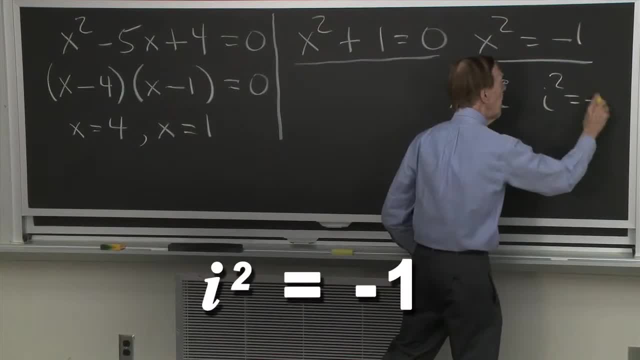 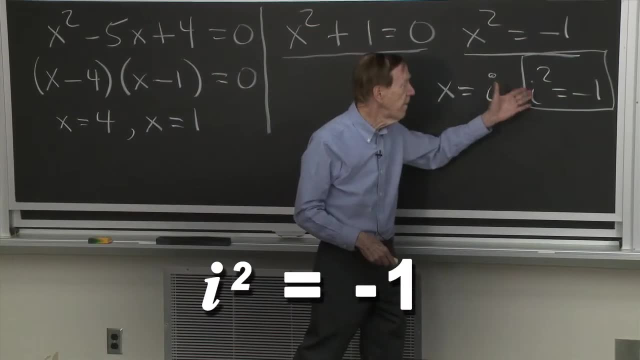 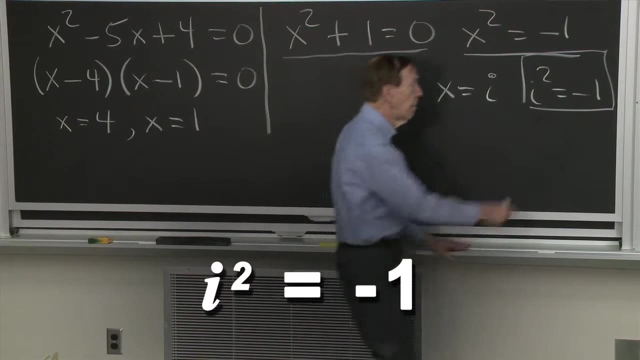 So x equal i. i squared equals minus 1.. That's the key to everything. All about complex numbers will flow out of that condition that, And any time we see i squared, we can replace it by the real number minus 1.. 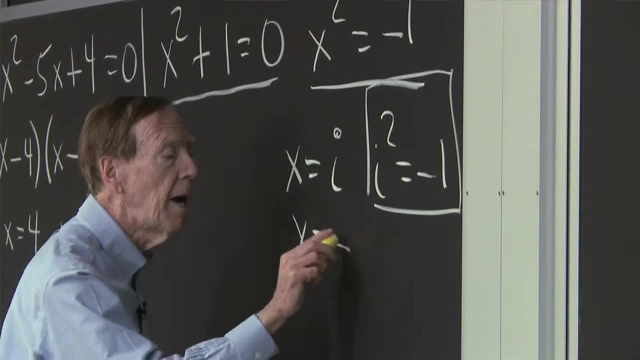 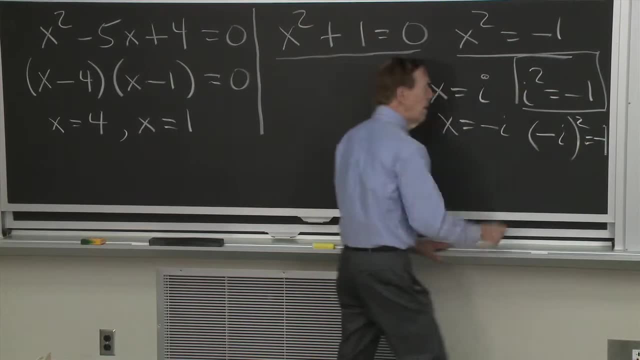 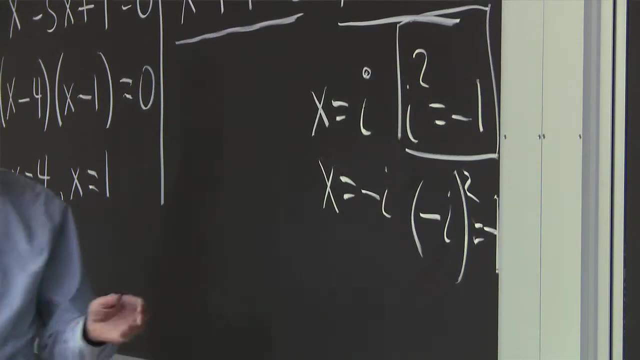 And this will also have another root: x equal minus i, Because of course minus i squared is also minus 1.. Because minus times minus gives plus. That leaves i squared, which gives us the minus 1. And this thing then would factor into x minus i. 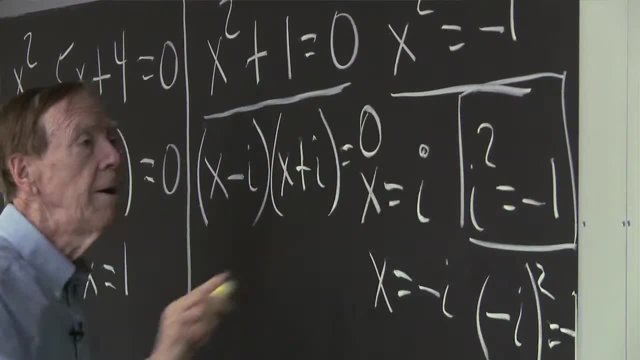 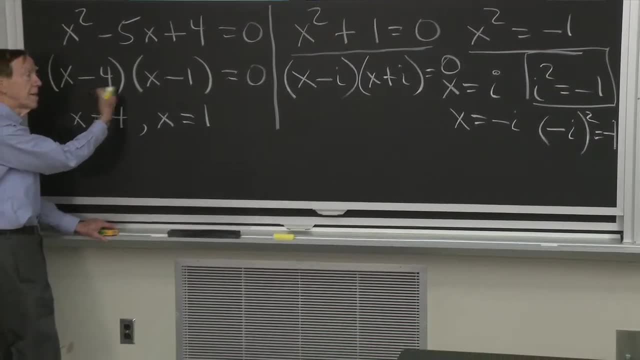 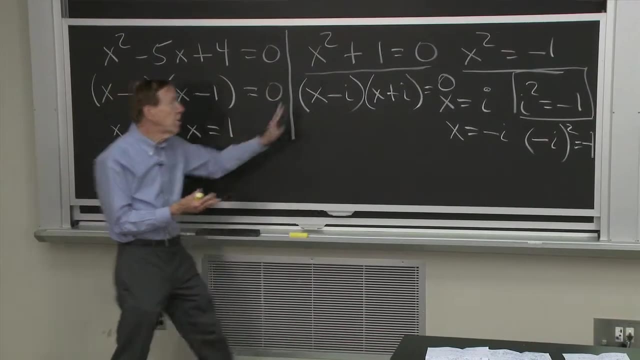 and x plus i equals 0.. What I want to say is: all polynomials can be factored, Maybe not so simply and easily as this one, But if we allow imaginary and complex numbers, we can still do it OK. So this is the starting point. 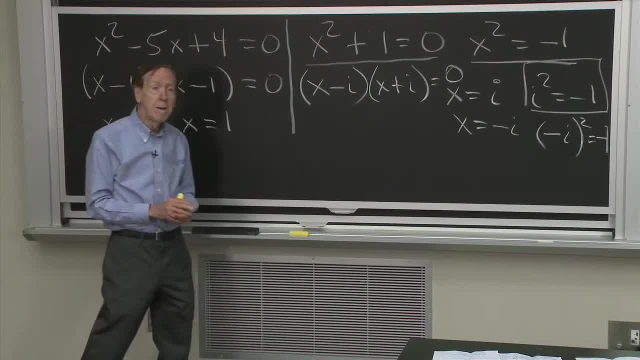 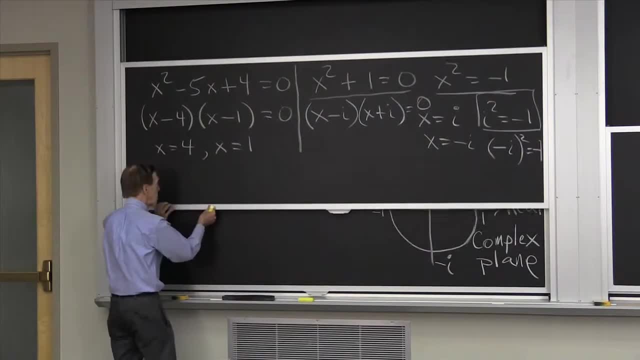 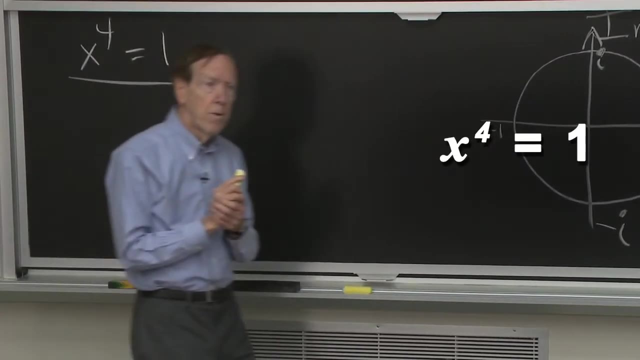 But I want to take a more interesting, more exciting equation. Let me get up to fourth power, So can I take, Let's go next to x to the fourth equal: 1.. OK, Degree 4.. I'm expecting four solutions to that equation. 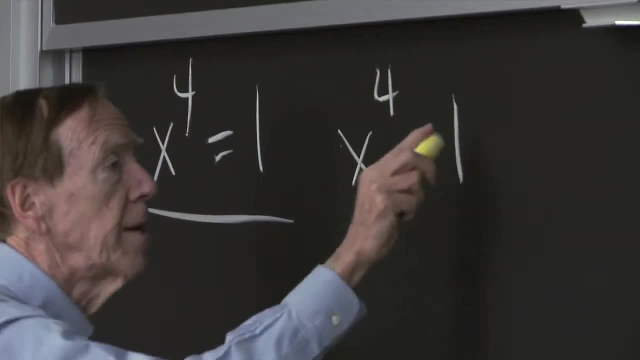 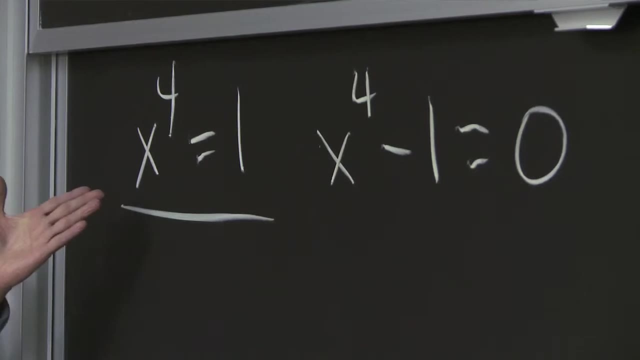 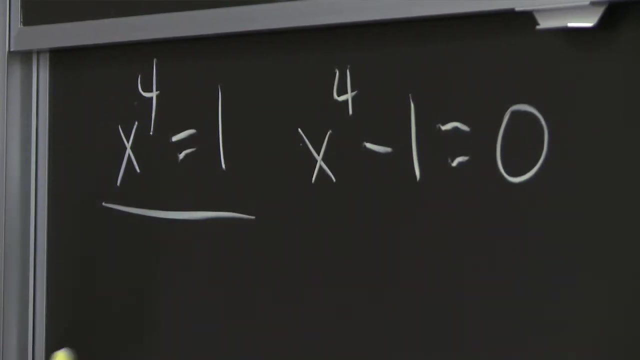 And of course I can write that equation as: x to the fourth minus 1 equals 0. Now, what are those four solutions? I'm taking four solutions because I see it's a degree 4 equation. OK, This I see. I could factor that without going imaginary. 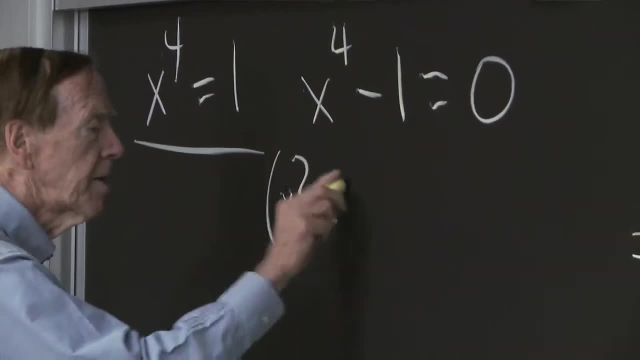 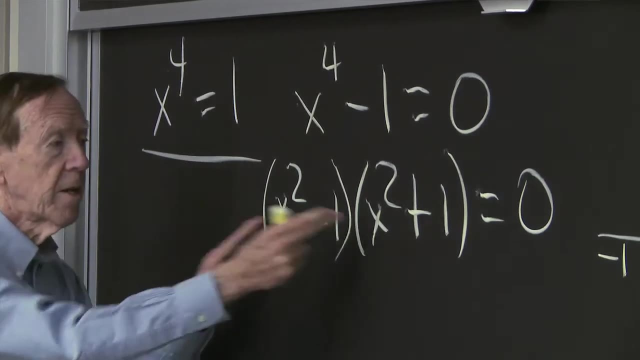 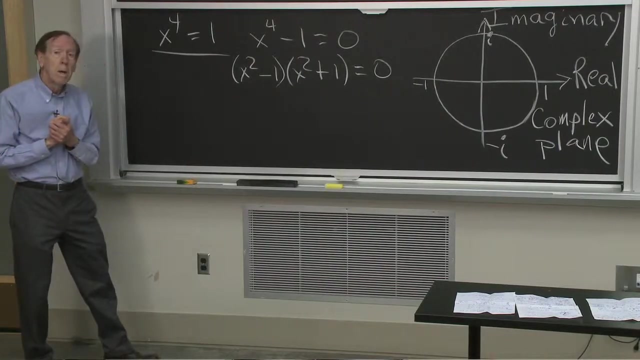 right away into: x squared minus 1 times x squared plus 1 equals 0.. OK, Because that gives me x to the fourth minus x squared plus x squared minus 1, is there? OK, Now get down to the solutions. So, if this is 0.. 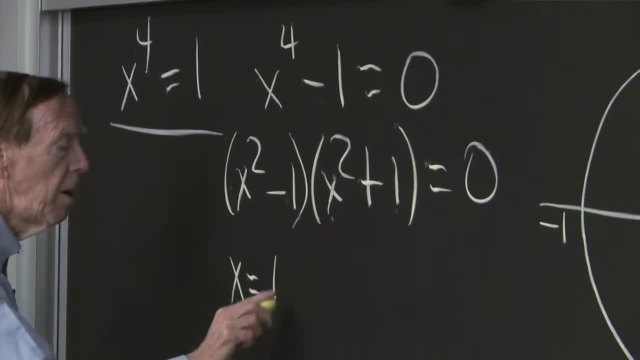 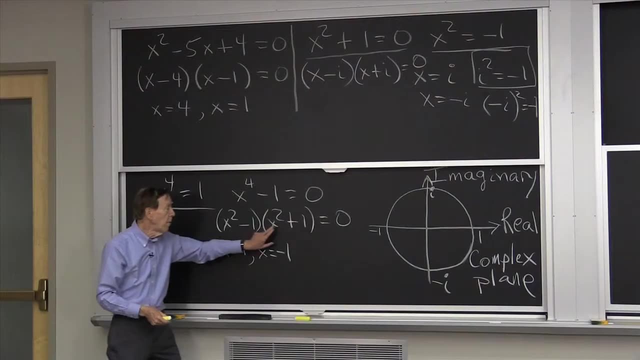 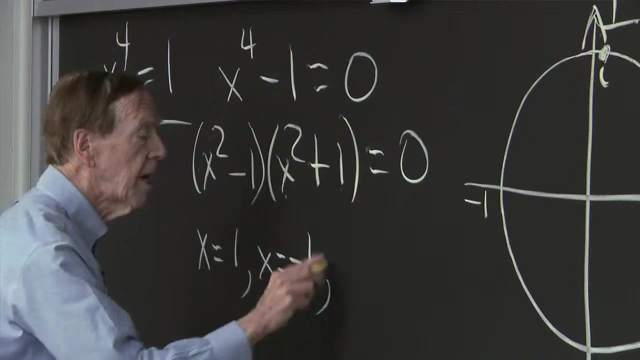 I have a solution: x equal 1 or x equal minus 1.. That gives me two solutions, because this is degree 2.. And what about this one? When can that factor be 0?? Well, that's the one we did. That's the one that gave us x equal i and x equal minus i. 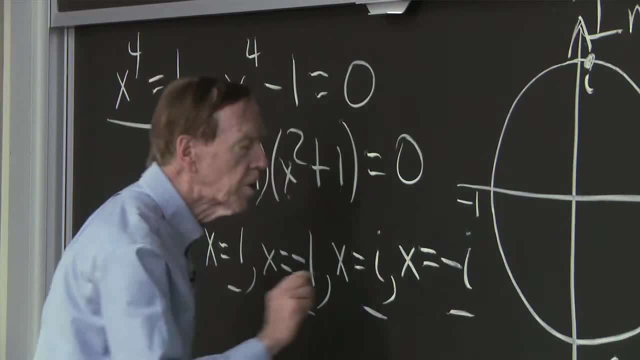 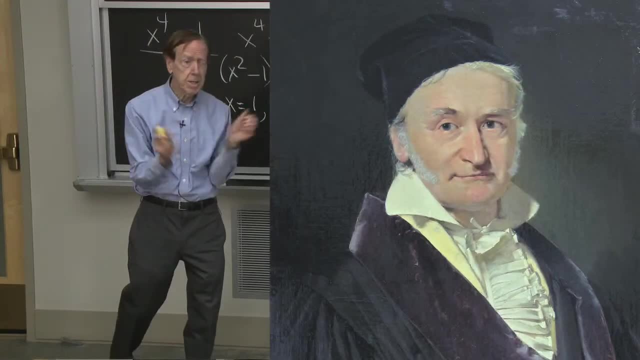 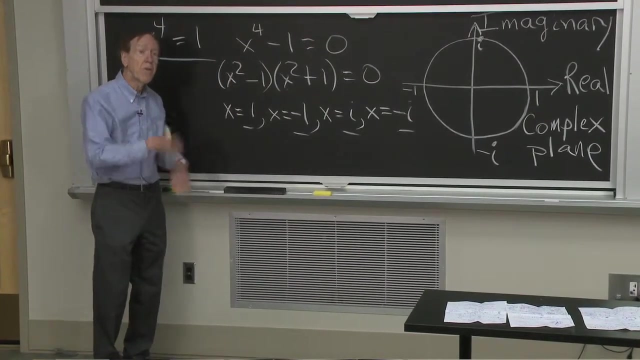 Those are the four- 1,, 2,, 3, 4- solutions to this fourth degree equation. That's what we expect. That's what Gauss, the greatest mathematician of all time, proved: That every fourth degree equation has four solutions. 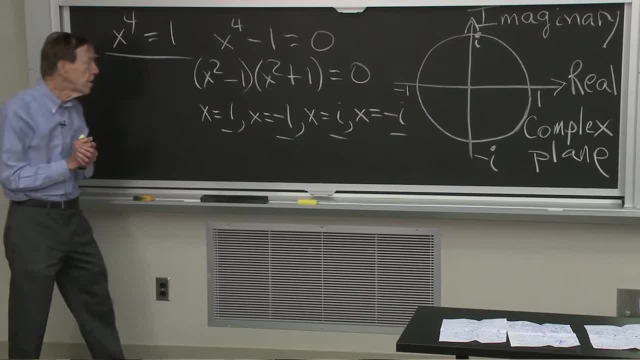 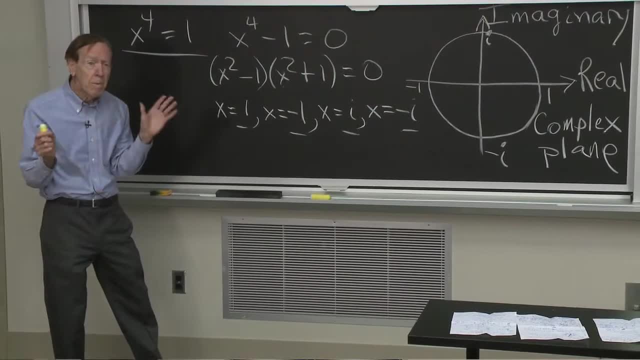 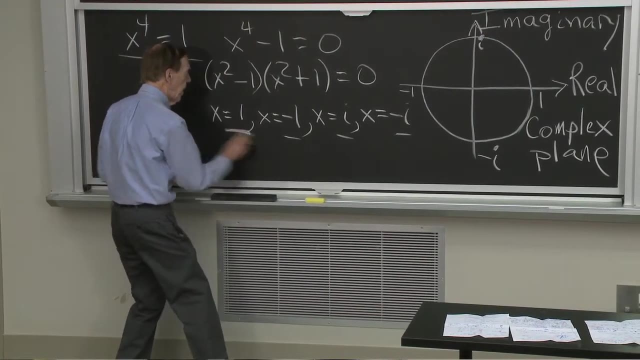 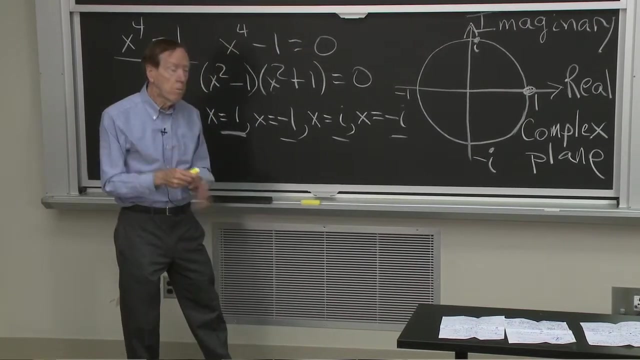 Every nth degree equation has n solutions. These four are nice because nice to draw. So I want to draw the complex plane. The complex plane has, Here's a real number: x equal 1.. That's setting along the real line, the real axis at 1.. 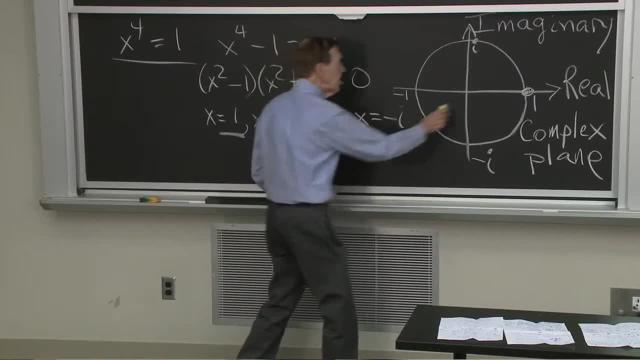 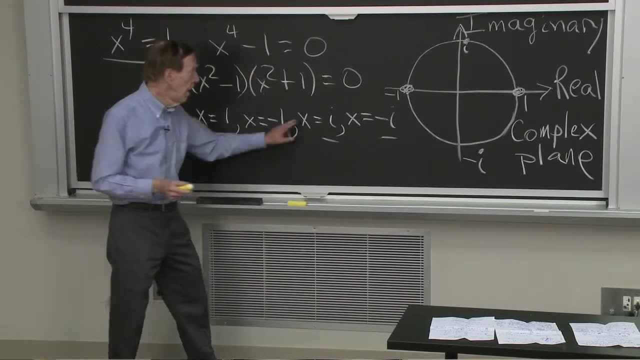 The second solution- x equal minus 1, is also real. It's at minus 1.. It's here. And the other two, x equal i, is up the imaginary axis. That's the point. We can have real numbers. 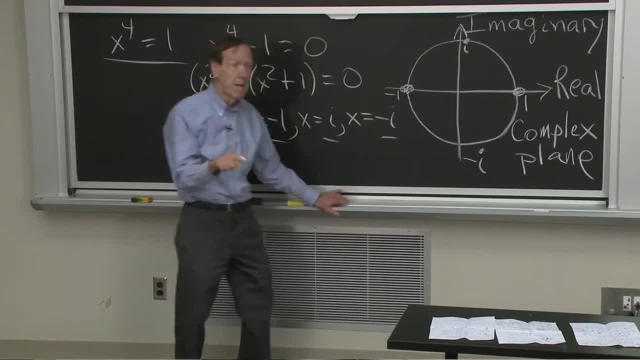 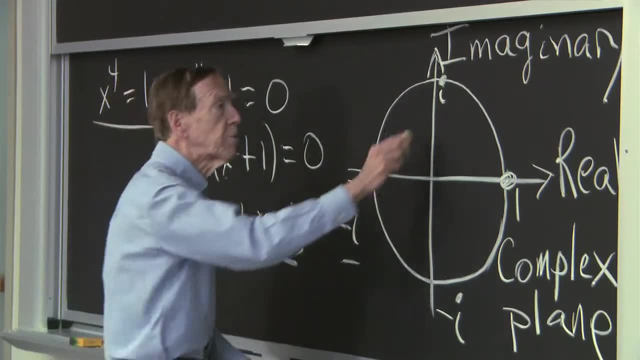 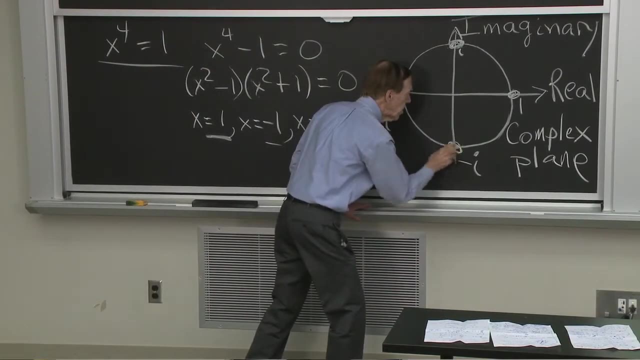 We can have imaginary numbers And in a minute, In a minute or in four minutes we're going to have complex numbers. But where is this imaginary number? It's right there, Right at the top of the circle, And minus i is at the bottom of the circle. 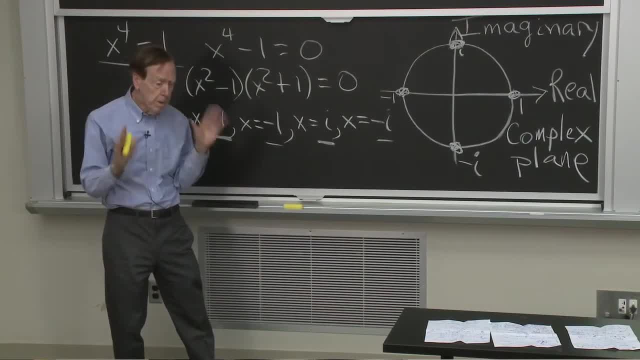 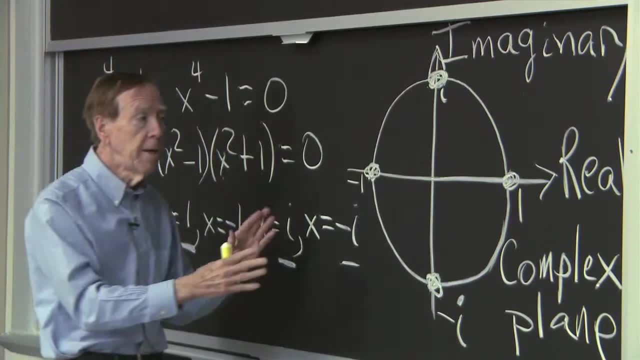 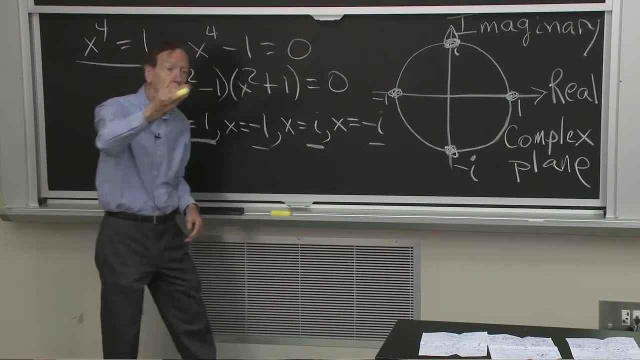 I put in that circle because it's very important. It gives you a sort of good picture of the complex plane. The plane has 0 in it, Has small numbers And has larger numbers And that unit circle where the numbers are somehow of size 1,. 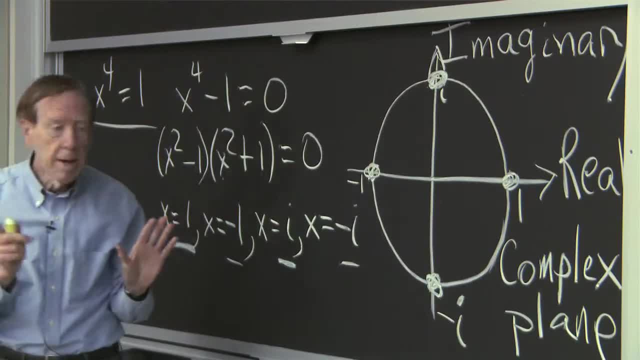 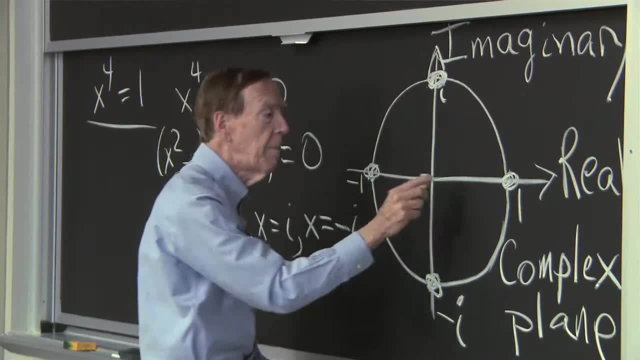 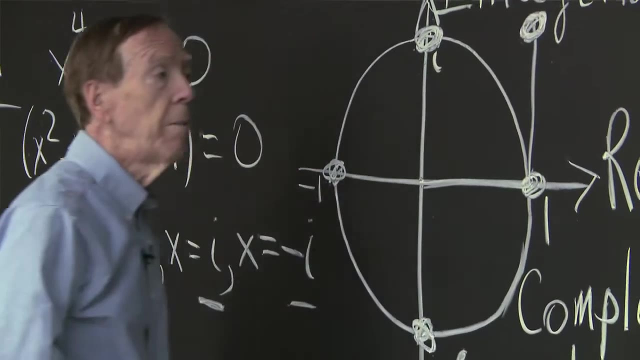 is the great thing to see. I'll tell you what a complex number is. It has a real part And it has an imaginary part. Let me take the real part, 1, and the imaginary part, i. There is 1 plus i. 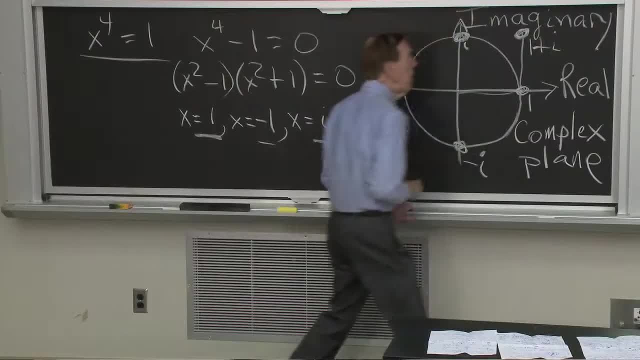 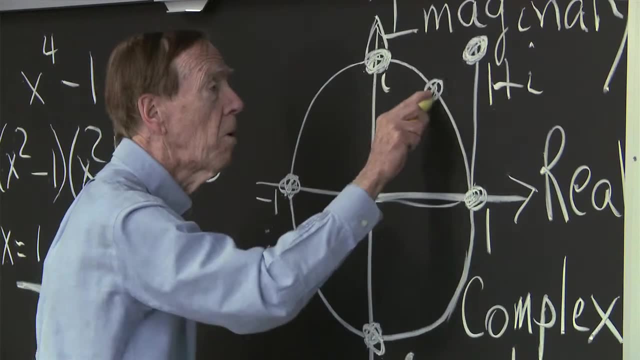 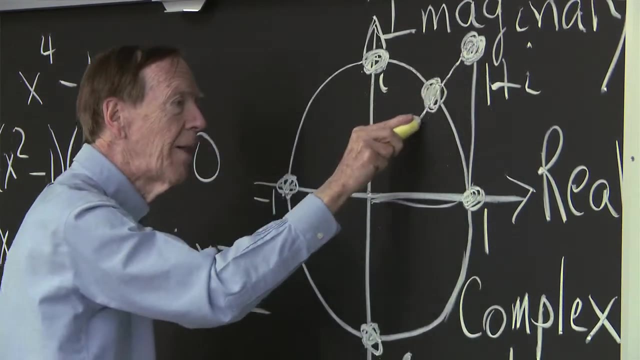 That's 1 plus i. 1 plus i, That's bigger than 1.. You notice it's outside the circle. If I want to bring that into the circle, or maybe onto the circle, would be nice, Let me draw that line because it's. 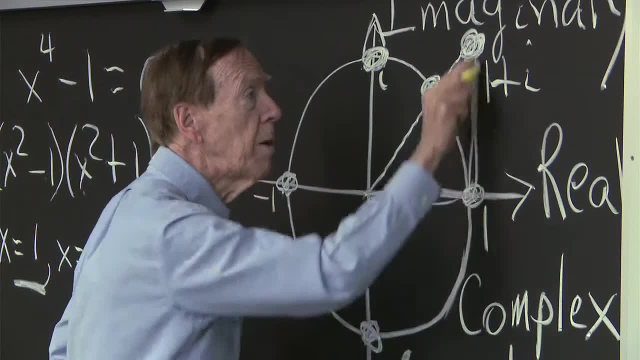 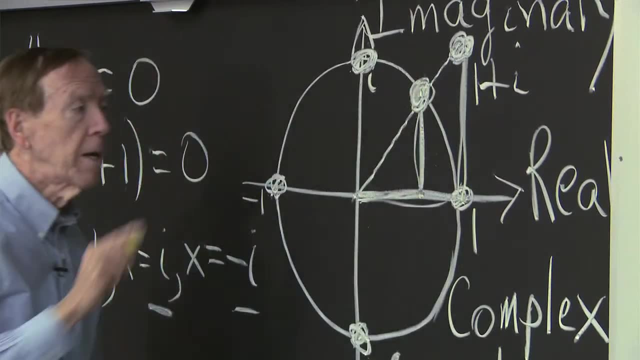 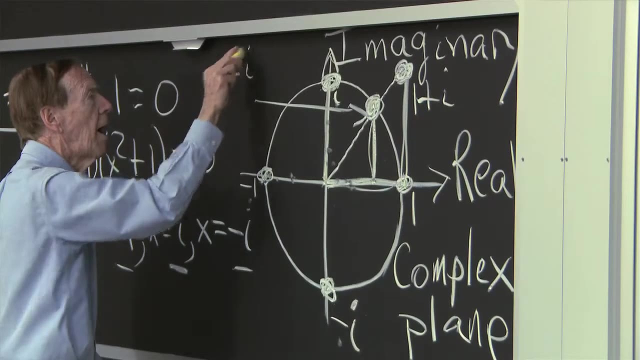 sort of part of the picture. So this one was 1 plus i. This is going to be some smaller number plus some smaller number times i, that point. So let me tell you what that number is. That's 1 plus i, divided by the square root of 2.. 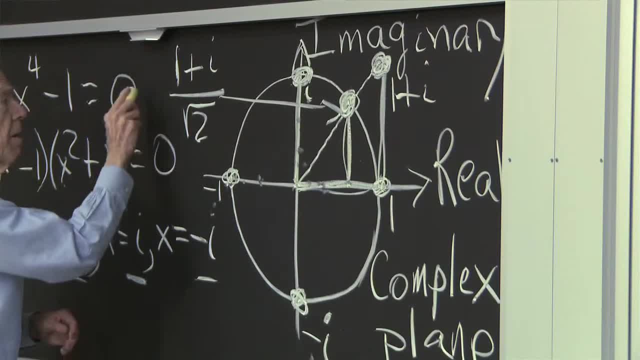 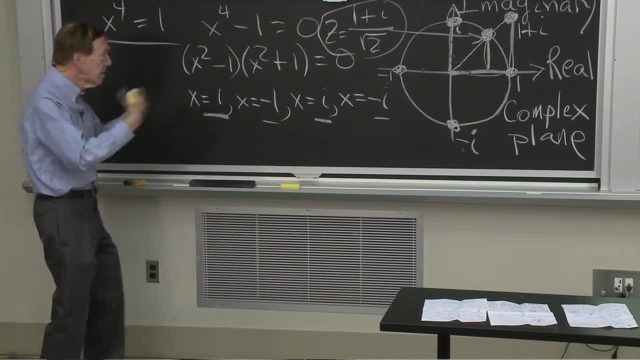 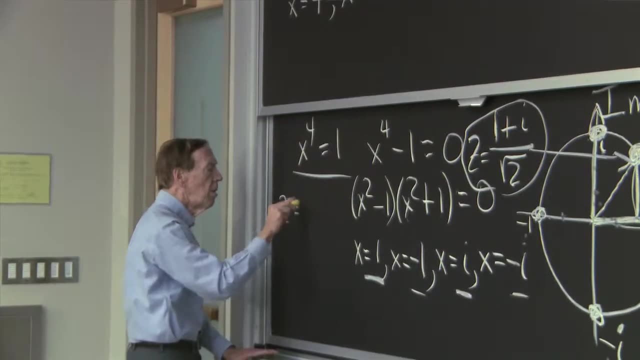 I have to bring it back. That's a special number. Let me call that z. OK, here's a challenge. During the next pause, let me write again that number z is 1 plus i over the square root of 2.. 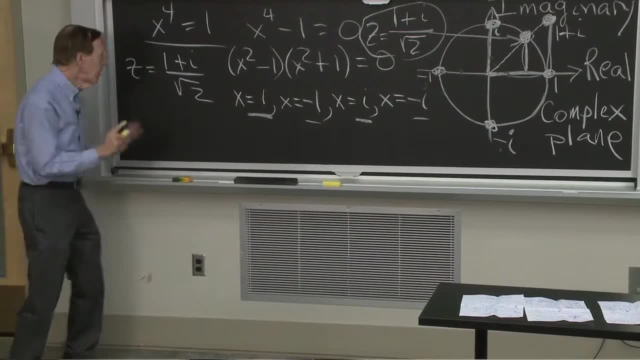 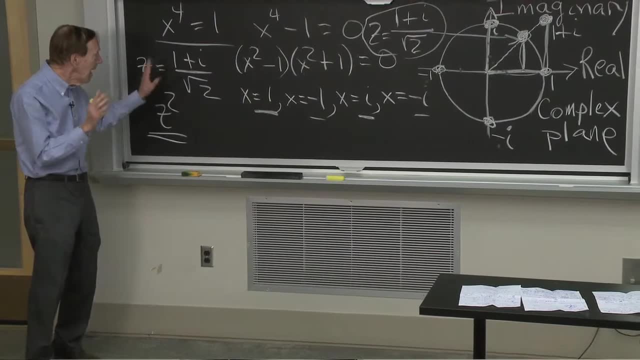 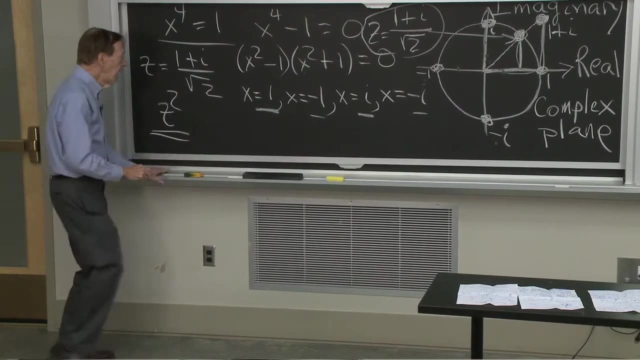 What I want you to do is Figure out what is z squared. Think you can do that. Figure out how could I multiply that by itself, See what I'd get, And then if you can think about the equation z. 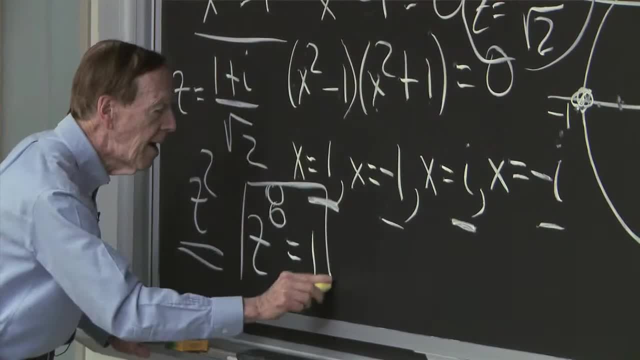 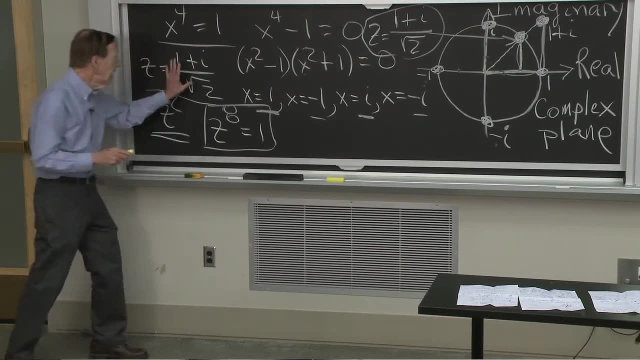 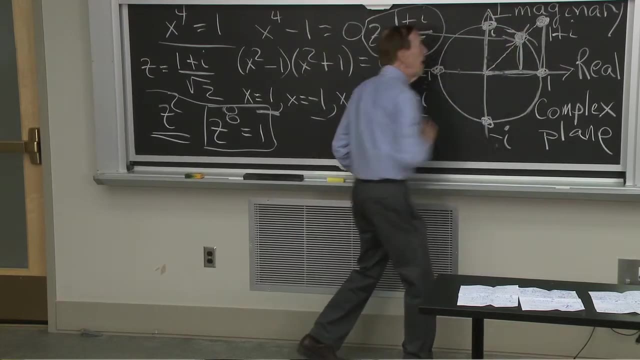 to the eighth equal 1.. Can you in fact this z, this wonderful z, it's eighth power will be 1.. So that will be, this will be this number. right, here is a solution to the equation z to the eighth equal 1.. 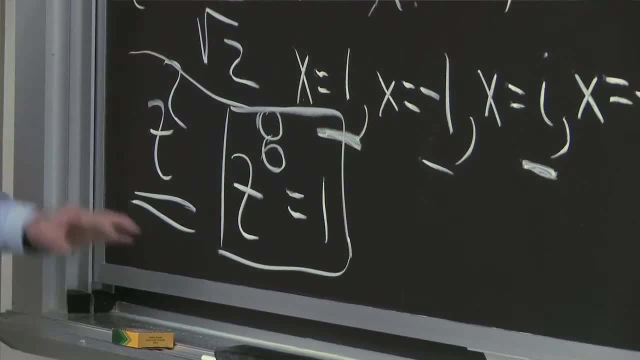 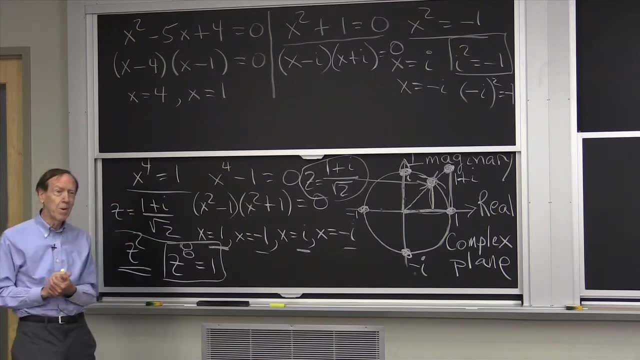 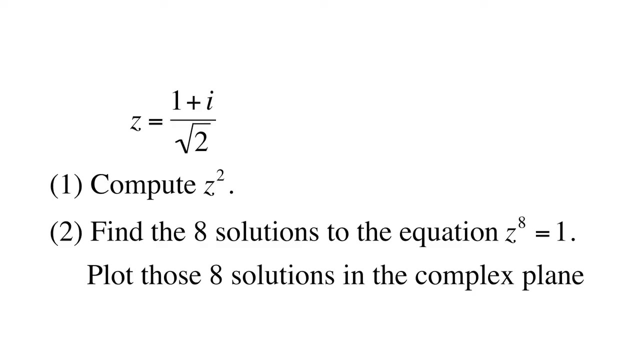 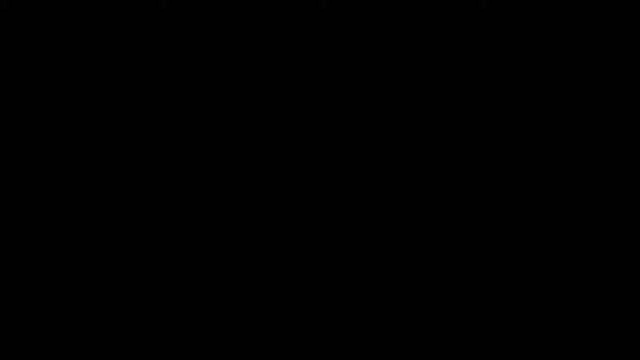 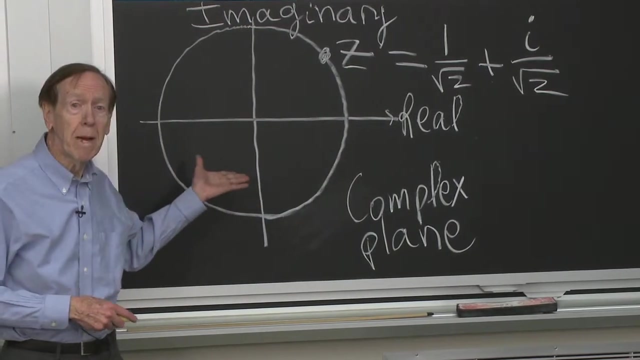 And we know how many more solutions do we expect? Seven more to make eight all together. Can you find them? OK? that gives you more than enough to do, Thanks, OK, let me pick up by drawing this complex plane again. 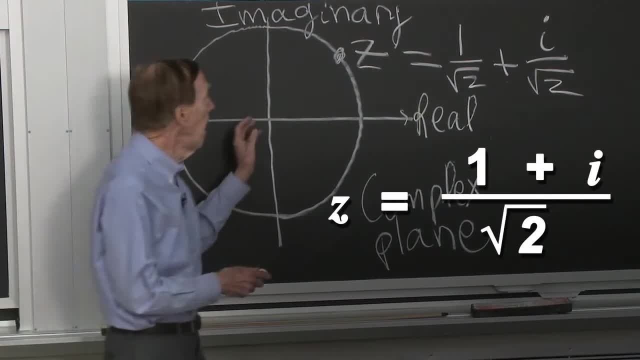 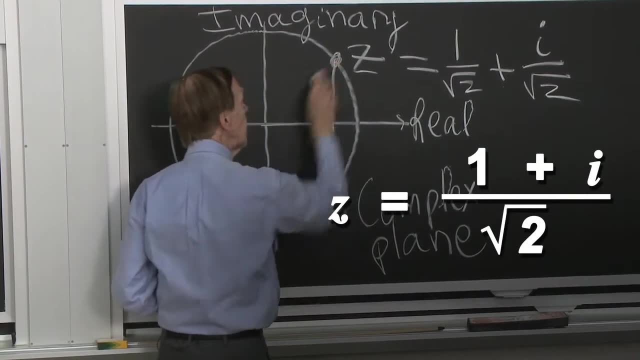 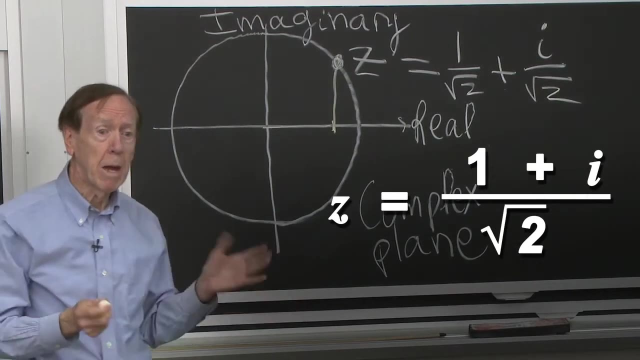 And that point z, the particular point that goes along the real distance 1 over square root of 2, up the imaginary distance and produces that number z. So that's a typical point in the complex plane. I'll draw other points too. 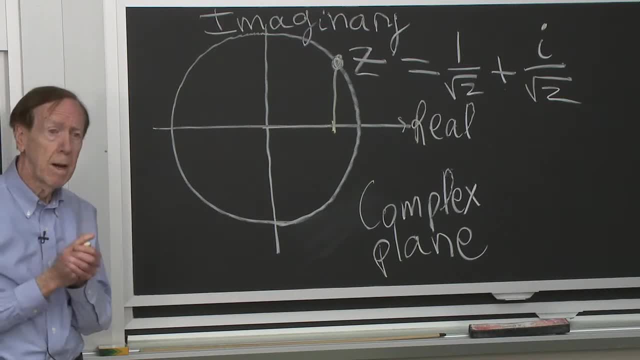 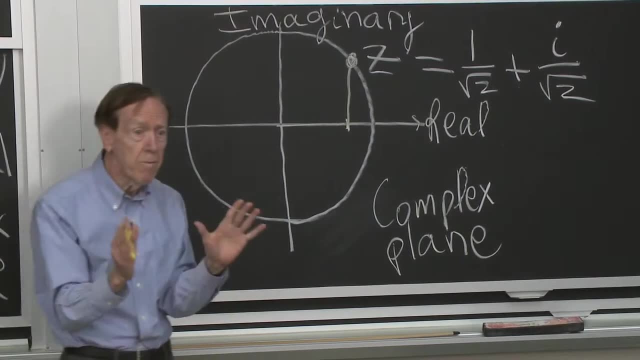 What do I want to do with these complex numbers? I want to be able to add them And I want to be able to multiply them. So that's what that's our first job is: How do I add complex numbers? Let me pick an interesting complex number. 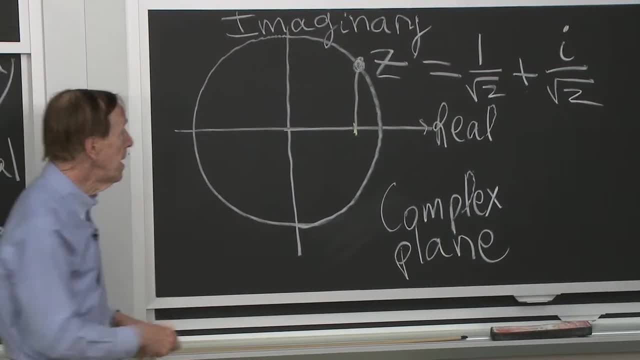 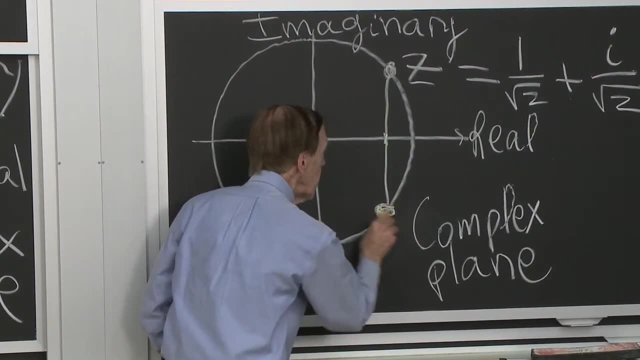 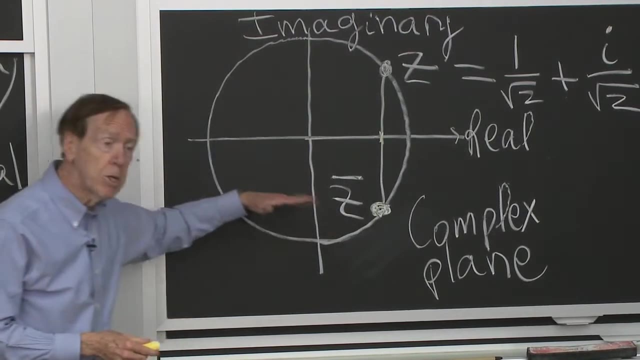 This number that goes with that one. it's down here. It's sort of the mirror image of that one. It's. so let me call that one z bar. That bar tells me it's the mirror image in the real axis. So what is z bar? 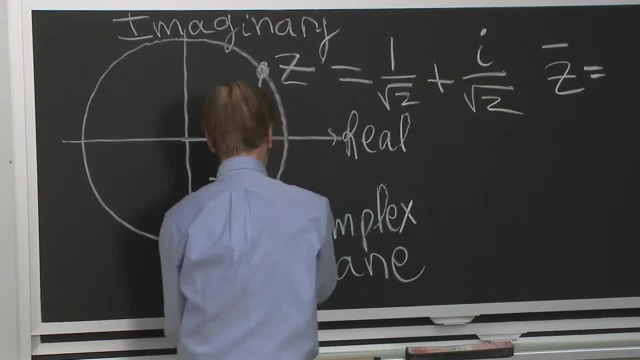 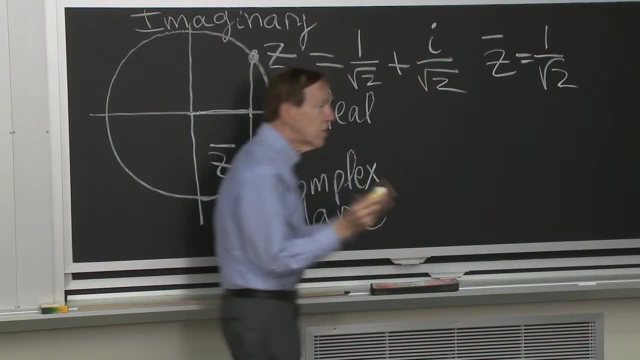 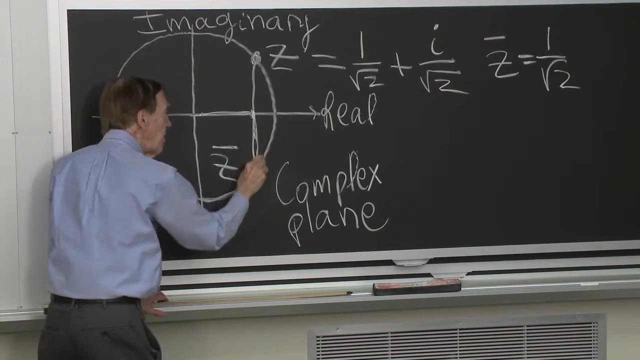 z bar. that point has the same real part, the same 1 over square root of 2.. And do you see what happens to the imaginary part? I change the sign. Instead of going up to z, I come down to z bar. 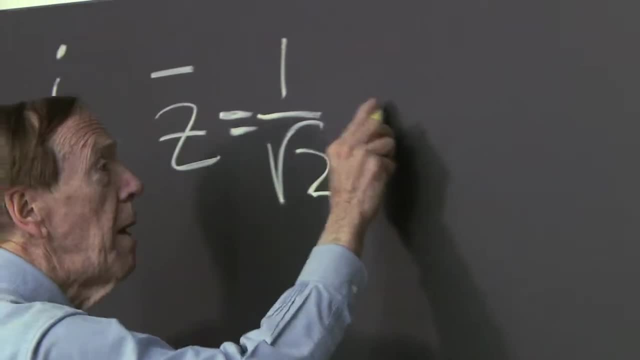 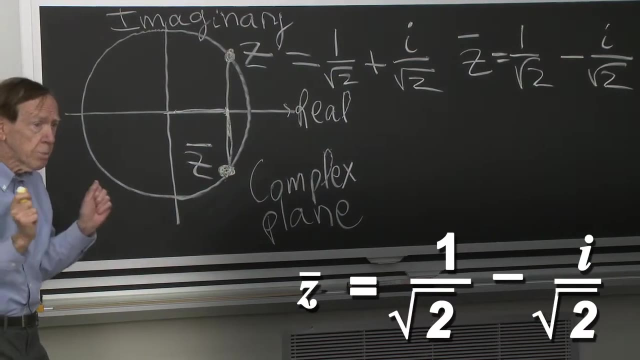 So instead of i over the square root of 2, I have minus i over the square root of 2.. So those are two complex numbers, rather special ones. That one is the conjugate. let me write that word conjugate. 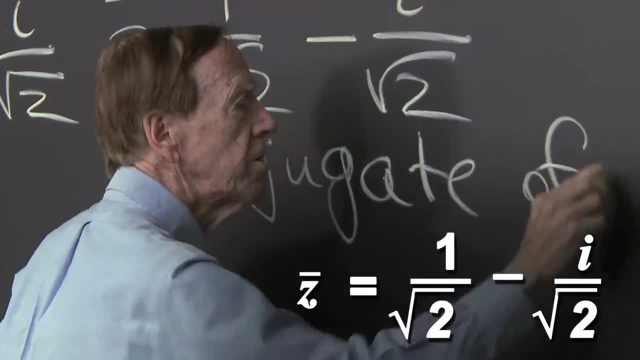 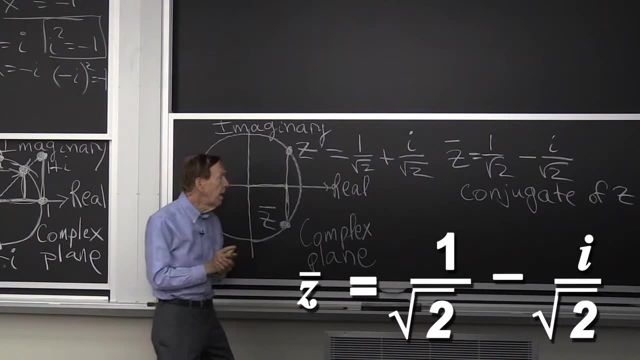 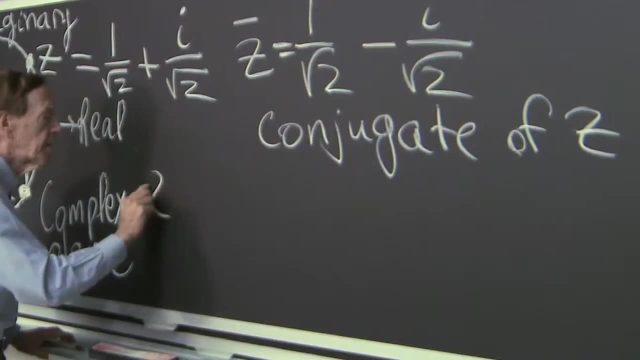 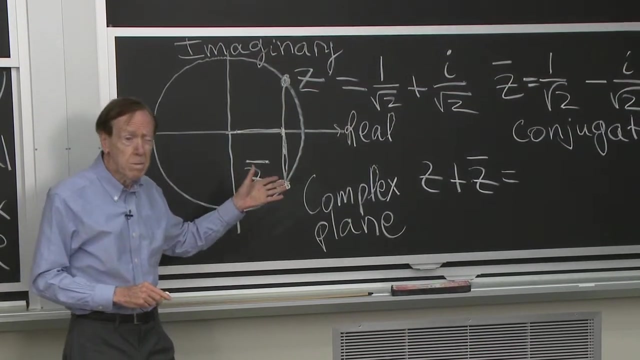 Or the complex conjugate Of z. You just change i to minus, i everywhere, you see. OK, so those are two candidates to add and to multiply. Let me do add first. What is if I add complex numbers and they happen to be conjugates in this example? 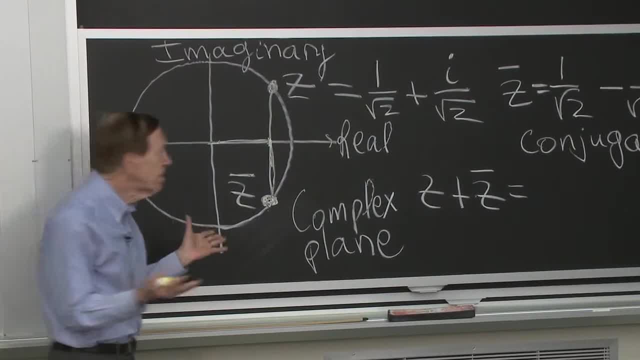 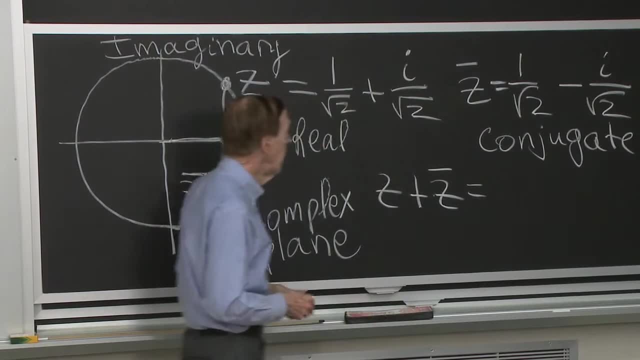 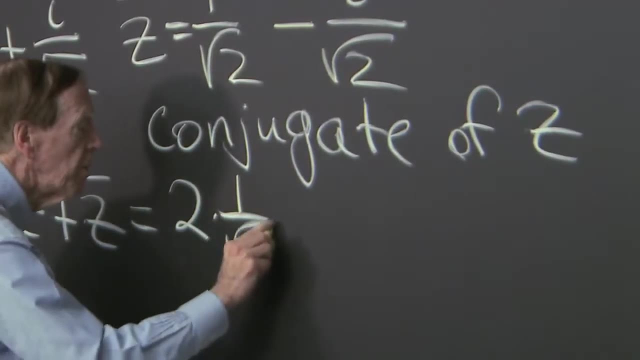 how do I add complex numbers? Just what you have to do: you add, you add the real parts, So I add that real part to that real part. So I'll have 2 times 1 over square root of 2.. 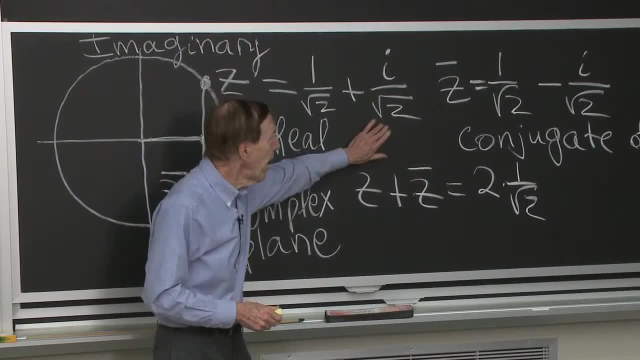 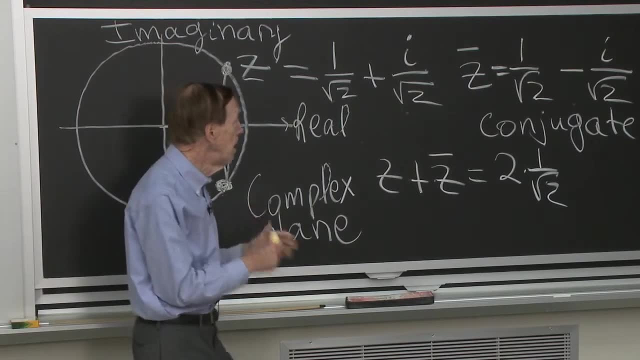 And I add the imaginary parts, I add that part to that part, And what do I get for that? Those happen to cancel. That's the idea of conjugates. So that number plus its conjugate is a real number, And I could write this as square root. 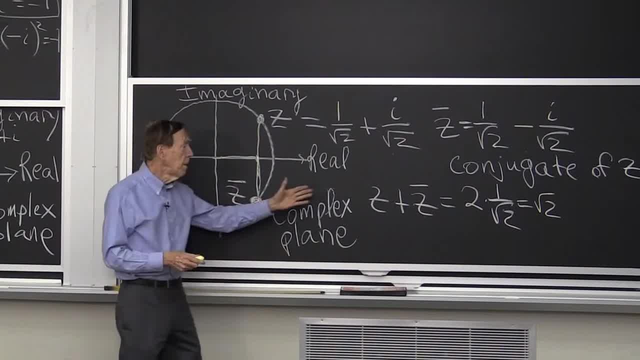 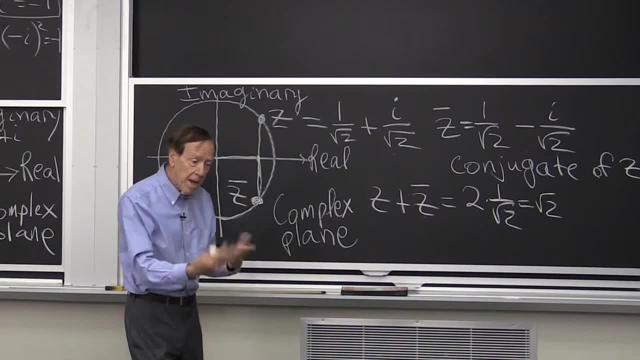 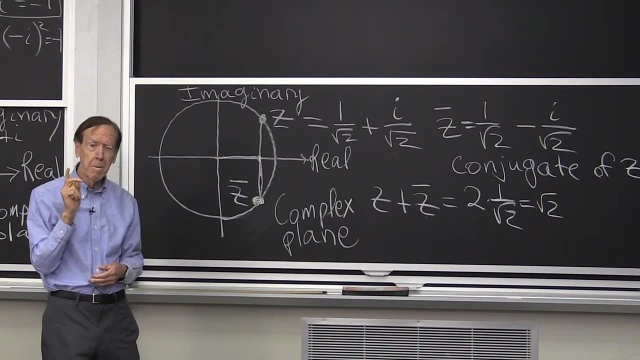 of 2. It's the real number, So that's the rule for addition. Just do what you have to do: Add the real parts, add the imaginary parts and you've got it. Multiplication is really the most interesting operation on the complex plane. 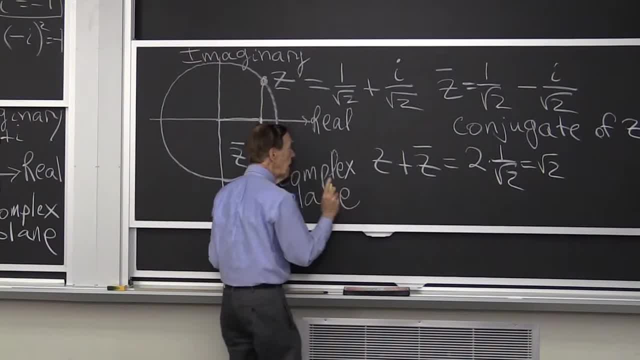 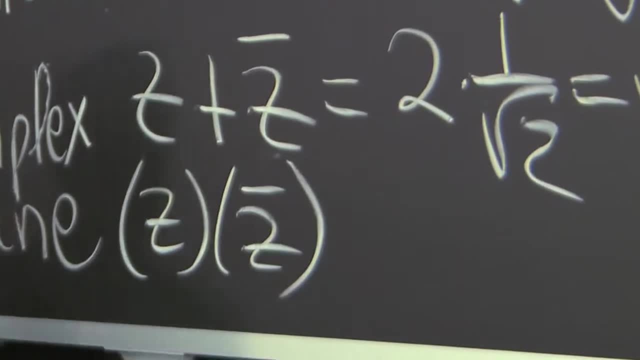 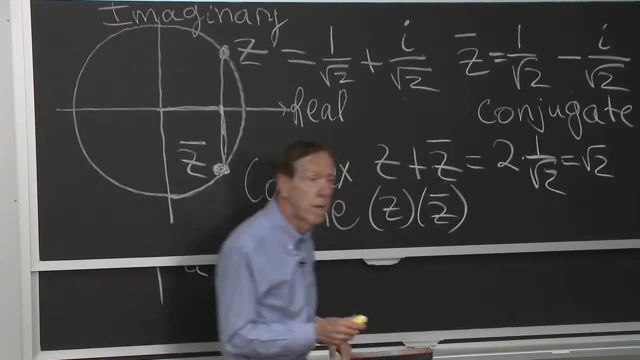 So let me do a multiplication. Let me multiply these two numbers. That's rather special too: z times z bar. How are you going to do that multiplication? You're multiplying that which has two pieces times that which has two pieces. 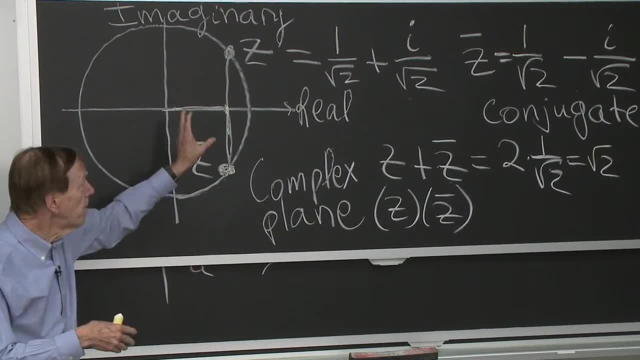 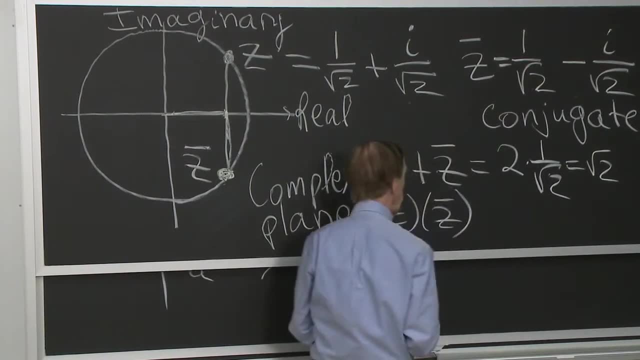 But all you do is multiply every piece on the left by every piece on the right. Put them together So I'll multiply 1 over square root of 2 times 1 over square root of 2.. That'll give me a half. 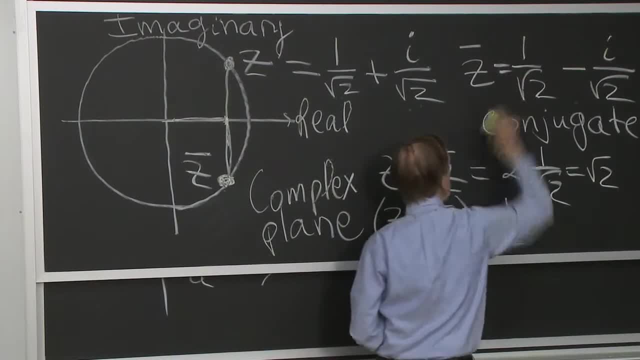 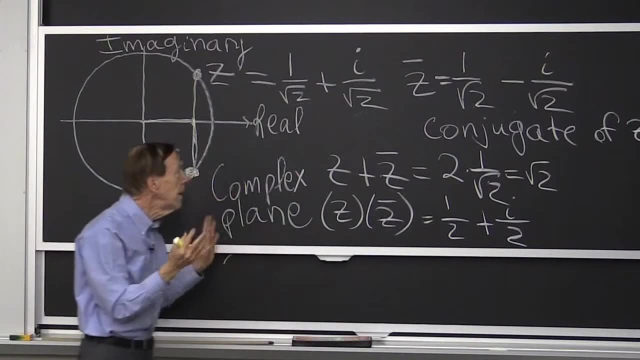 And then I'll multiply i over the square root of 2 times 1 over the square root of 2.. That'll give me a plus: i over the square root of 2.. i over 2, I think That times that will be an imaginary part. 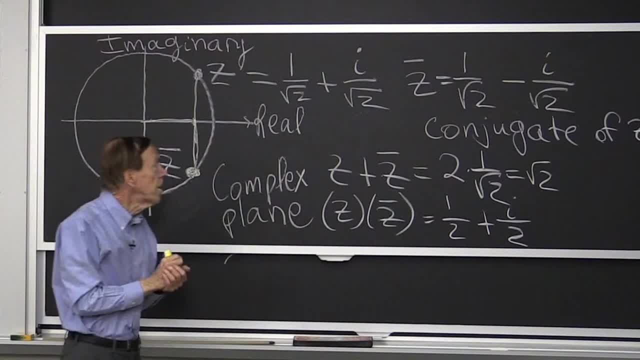 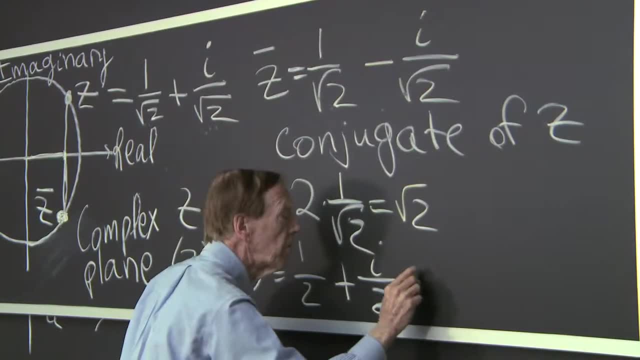 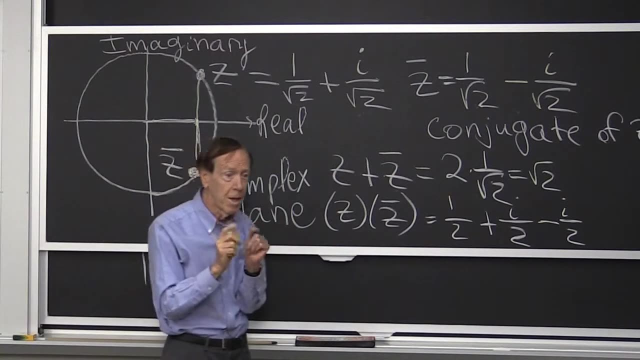 This times this will be also an imaginary part. Oh, it's got the minus sign now, So it will be a minus i over 2.. And then finally- and this is I'm getting finally to the importance of i When I multiply that part by that part. 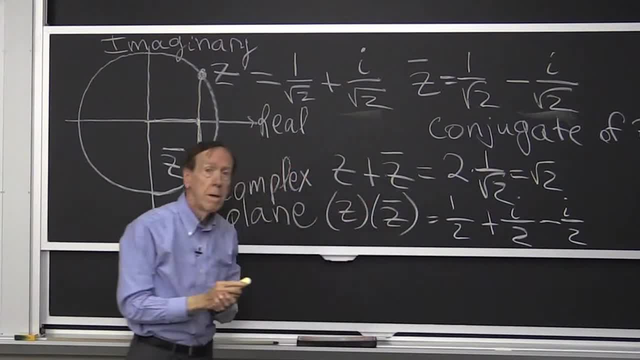 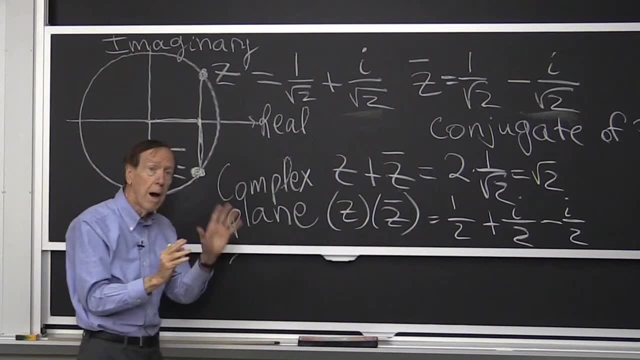 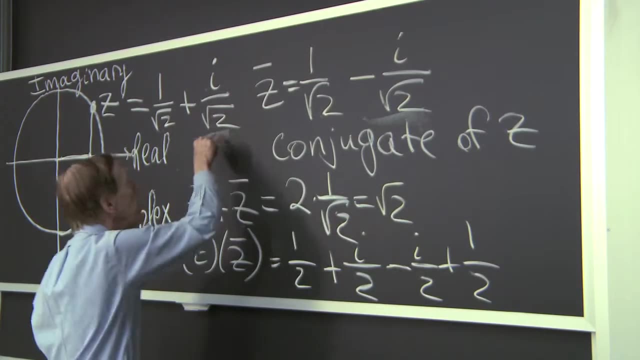 I have i times, I times i, which is minus 1.. And then there's the minus sign, so I'm plus 1.. So I'm real. The i times i produces this real number which is, I think, a half again. 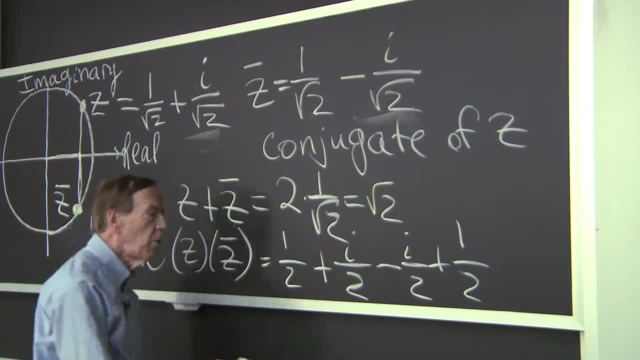 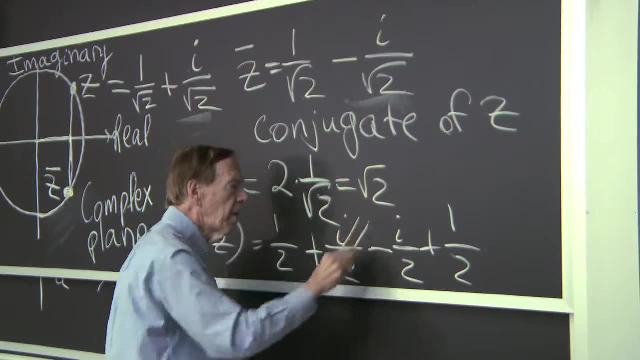 The square root of 2 times the square root of 2, giving me the 2.. Here's the point: With conjugate numbers, z times z, bar the imaginary parts cancel. I just have these two parts, giving in this case 1.. 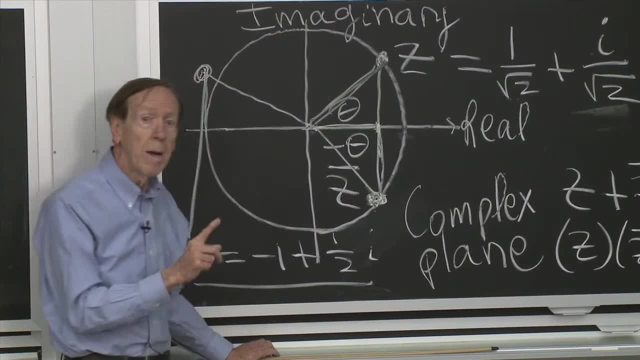 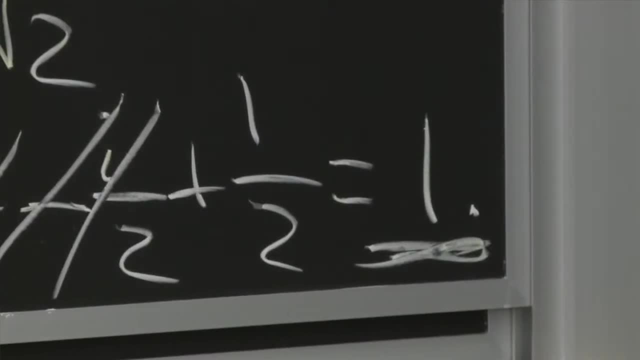 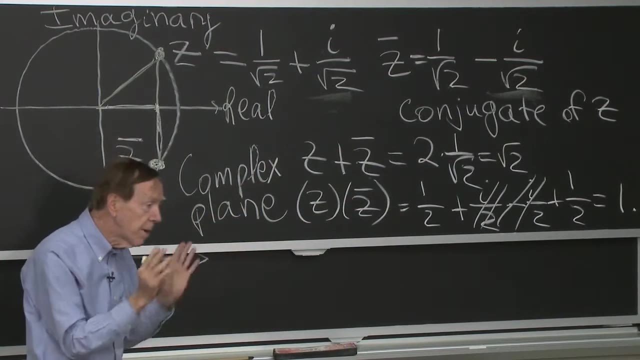 So in multiplying that distance is 1.. That distance is 1.. And when I multiply I got the answer 1.. That's the idea of complex conjugates, And it shows you how to add and how to multiply. But now I better take any two numbers. 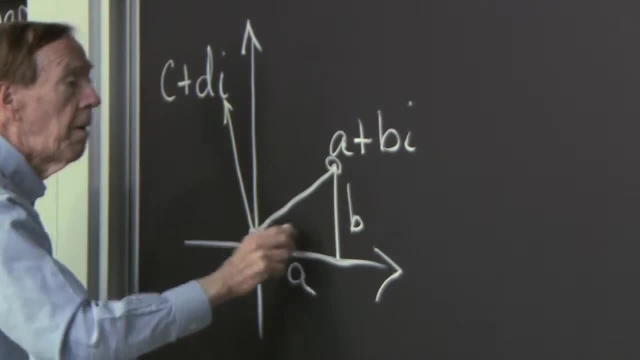 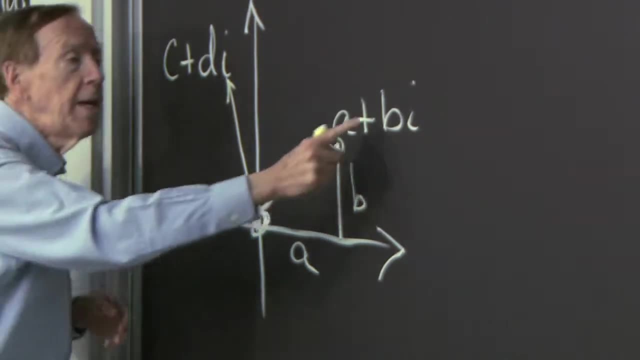 and just do the same thing. So here's one of my numbers: a plus b, b, i, any a or any b. a is the real part, b is the imaginary part. And here's another complex number. If I add them, what do I get? 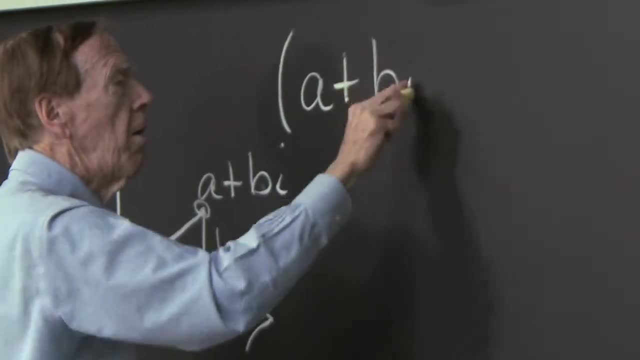 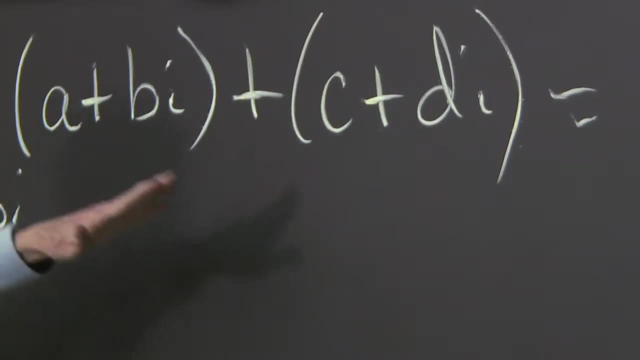 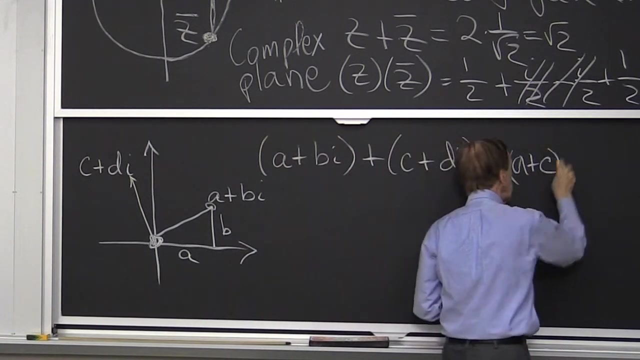 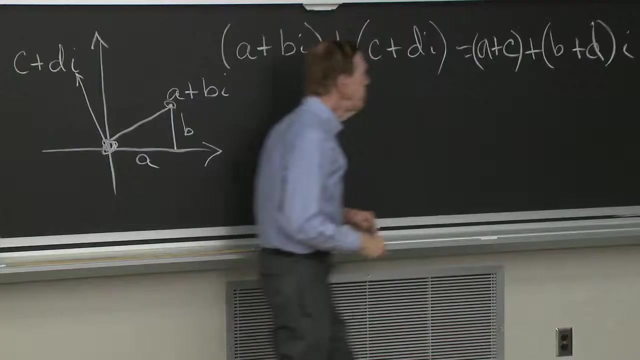 So if I add a plus b? i to c plus d i, what could it be but a plus c and b? i plus d i? So I have a plus c- c is the real part- And b? i plus d? i, Of course. 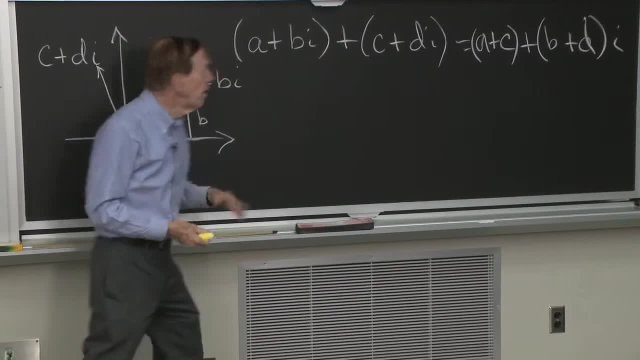 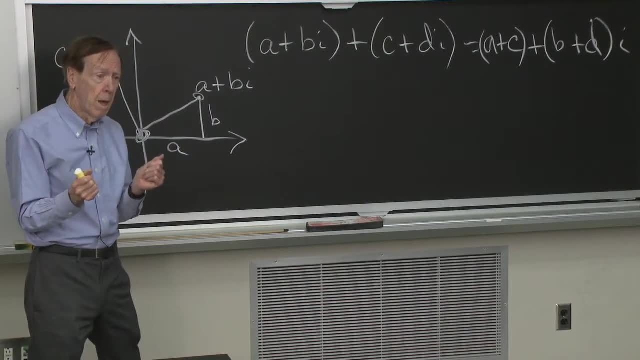 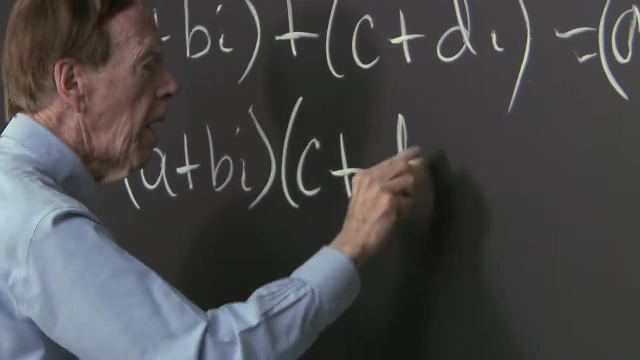 I just added the two pieces here and the two pieces there, separating the real parts and the imaginary parts. Now I'll multiply. I'll multiply those numbers: a plus b, i times c plus d, i. OK, So multiplication, That is the interesting one. 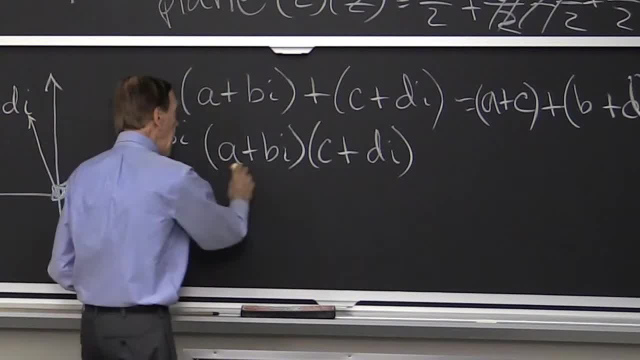 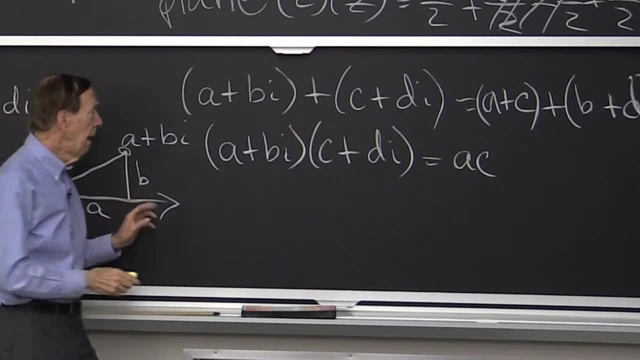 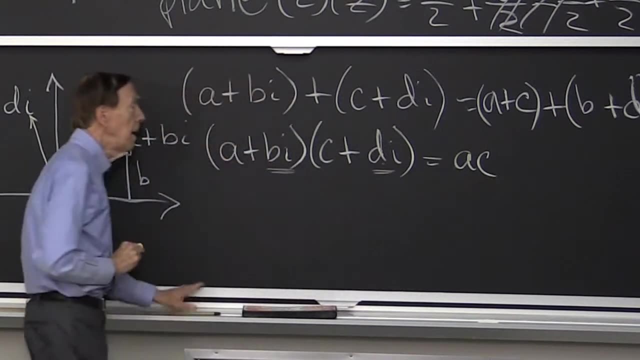 Here. let me do it the boring way: a times c- That's real. Where else am I going to get a real part? a times d i? That will be imaginary. I see a real part coming from b i times d i. 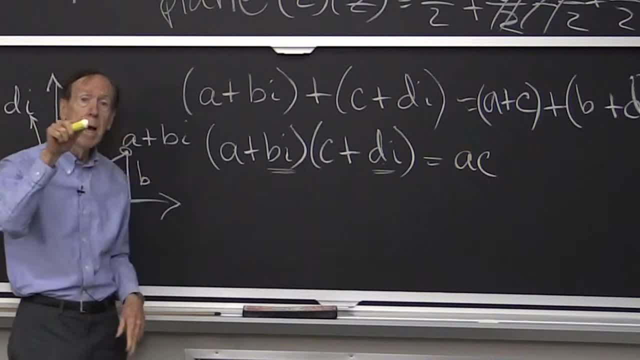 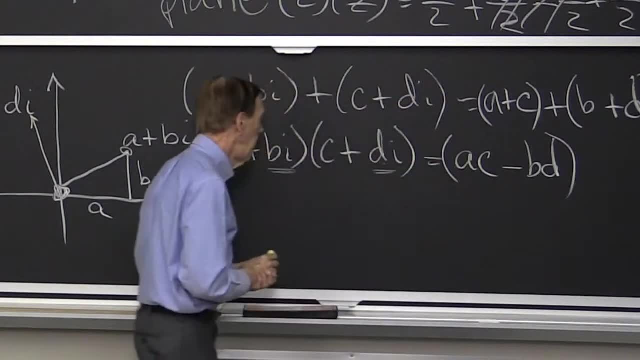 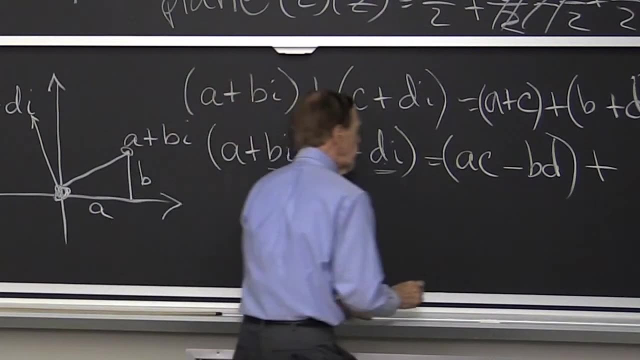 Do you see that When that multiplies that, I have b times d And the i squared is producing a minus b times d. So that's the real part, And now I'm ready for the imaginary part. That'll be a b i times a c. 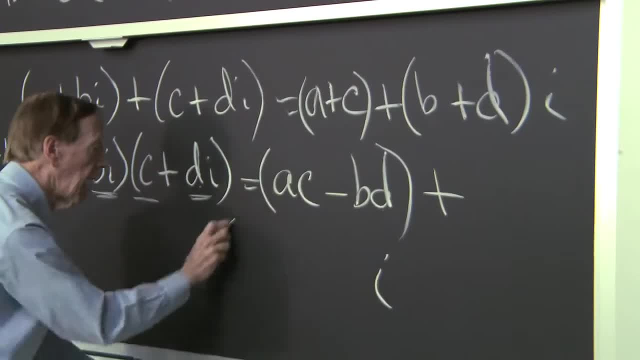 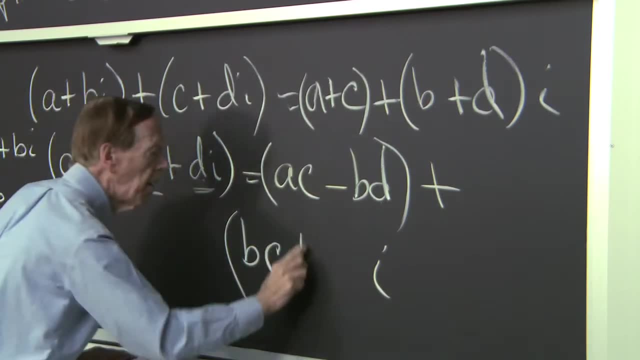 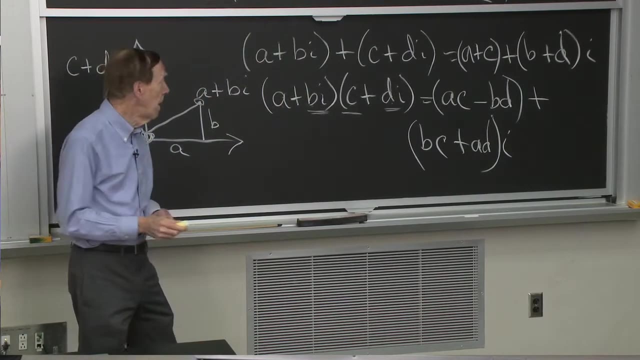 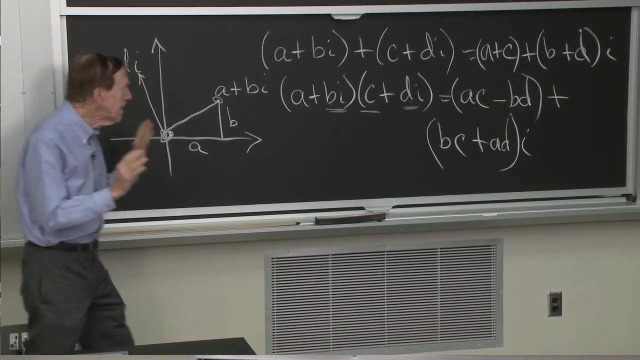 So the imaginary part is going to be an i something times i. So I have b times c times i And I have a times d times i. OK, Success, I multiplied two complex numbers. But But I don't see anything wonderful about that. 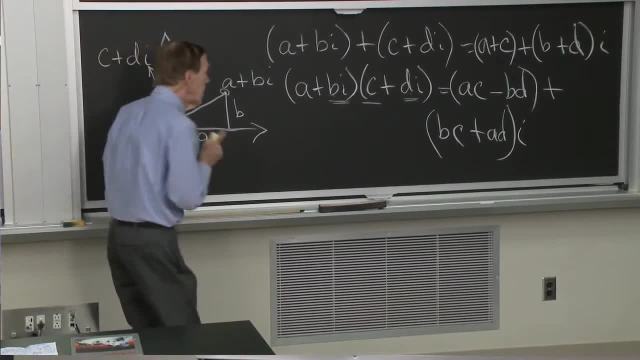 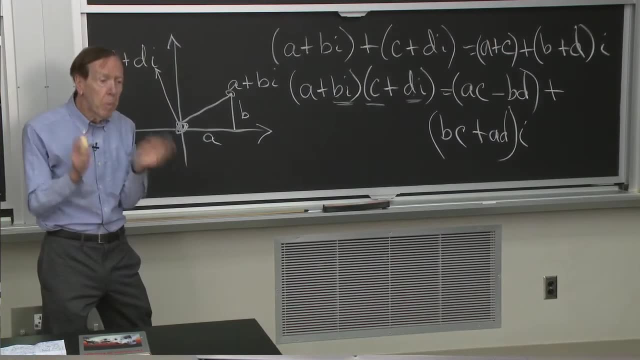 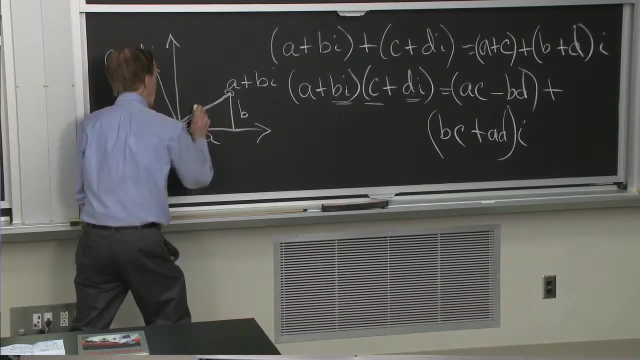 And there is something wonderful about it. Let me show you what happens when I multiply two complex numbers. So the point is to do multiplication. I want to get these distances involved. That distance I'll call r, This distance I'll call capital, R, That's. 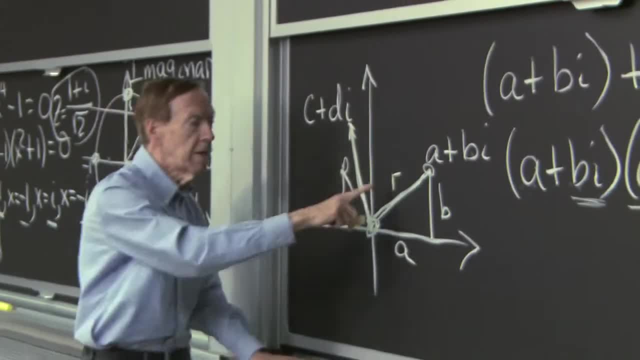 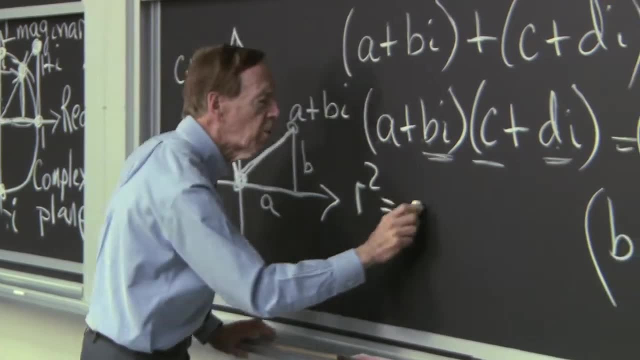 the sort of the. oh well, you see what r is r is r squared? well, Pythagoras is a key here. r squared is a squared plus b squared. Let me tell you what's going to happen in multiplication. 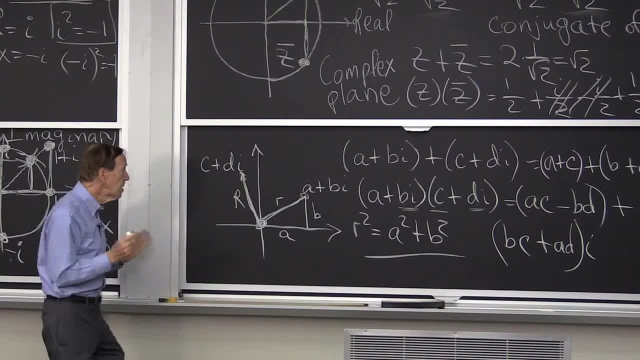 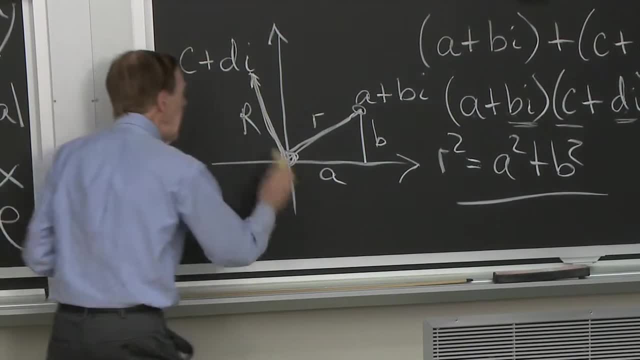 And then show it to you in the next segment. OK, What's going to happen When I multiply that number times that number? I'm going to get a number- oh, maybe out here, And it'll be. I'll add the answer. 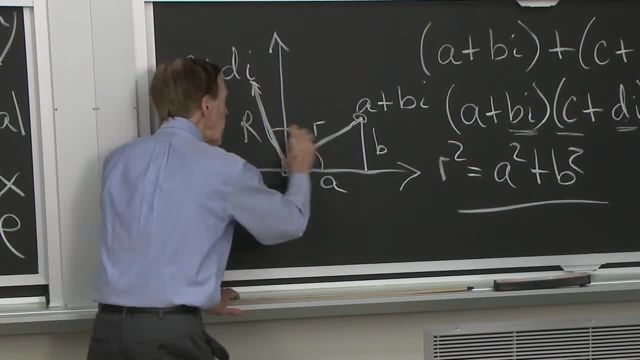 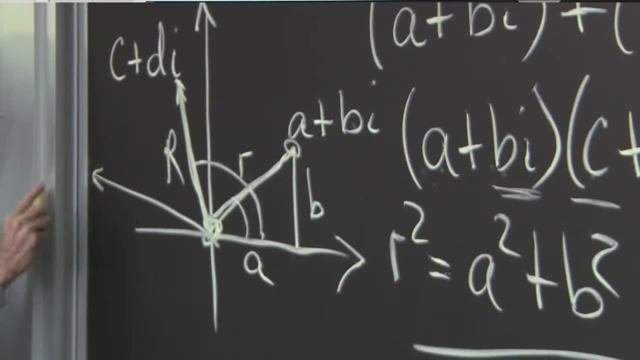 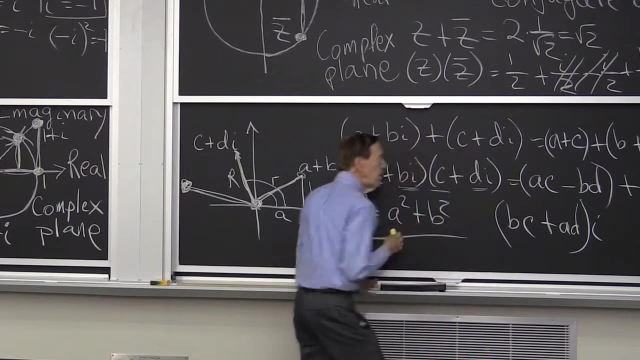 That's the key. I'll add that angle to that angle. What do you think That's about? when I add those, it might be off here. So this, I think, is that answer, And from that picture you don't see it. 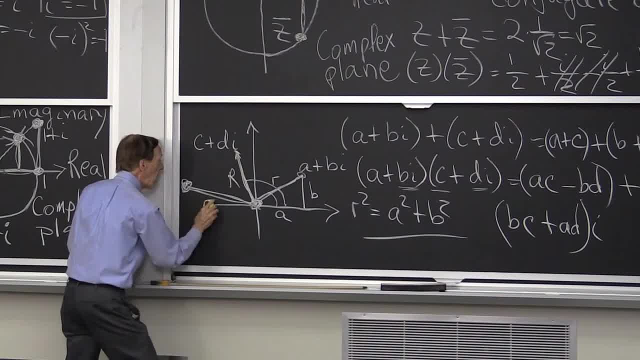 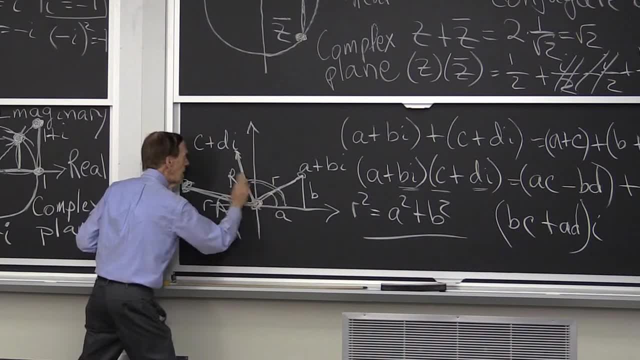 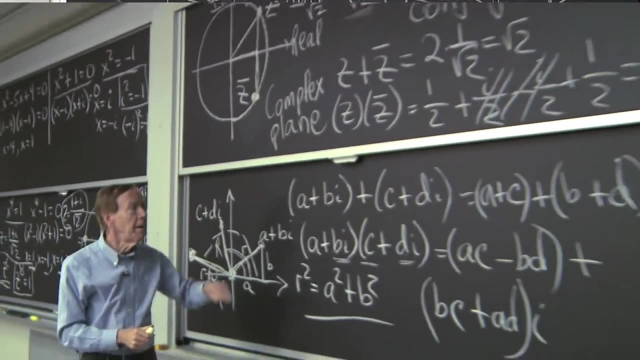 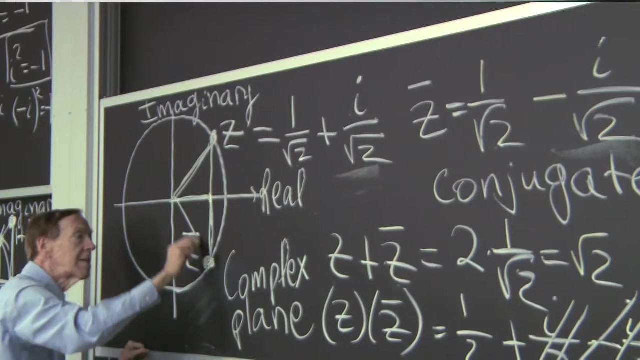 But from this picture with the r times, r is the length of that and the angle plus the angle gives me this angle. OK, Let me just test that on the first one. Can I come back to the first one When I multiply that z times that z bar? OK, 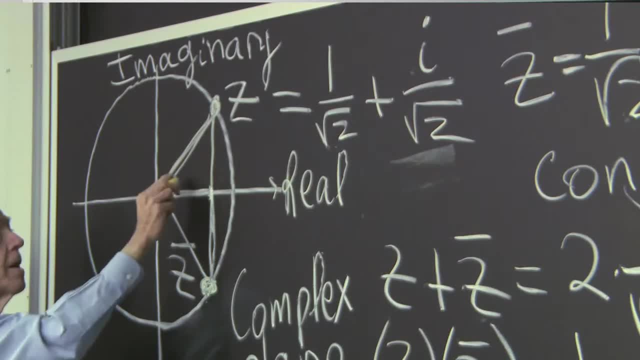 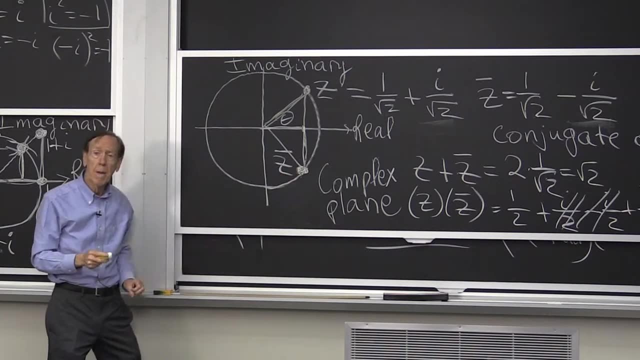 what are the angles here? This z is at some angle, let's say theta. maybe it's 45 degrees. And what's the angle for the complex conjugate Minus theta? you can see it because it's a mirror image. 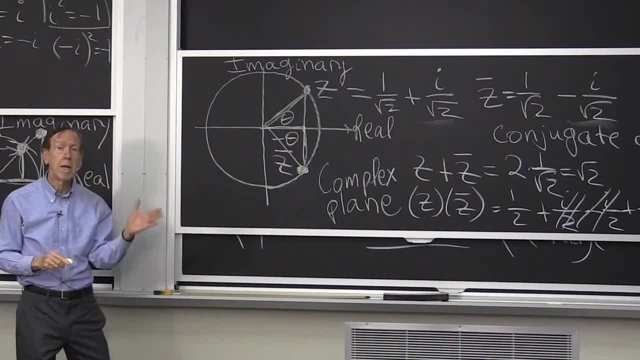 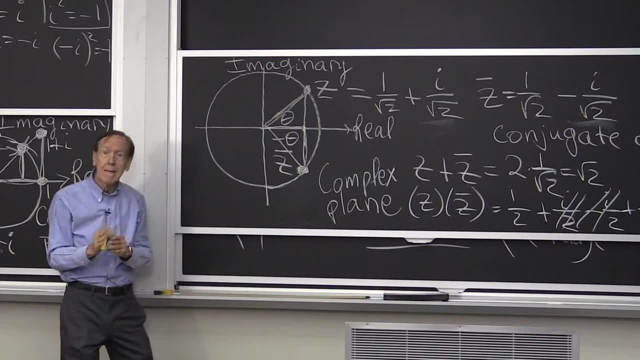 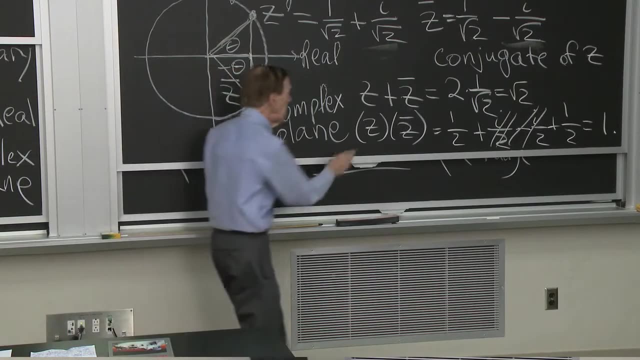 And what is the angle when I multiply z times z bar? I'm going to add the angle. so I'm going to add theta and minus theta 0. So z times z bar has angle 0. And, sure enough, z times z bar came out to be 1 at angle 0. 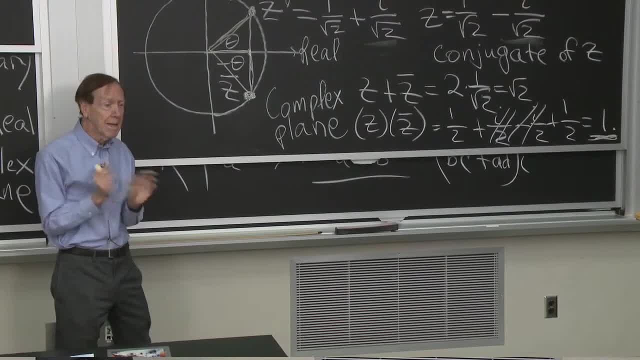 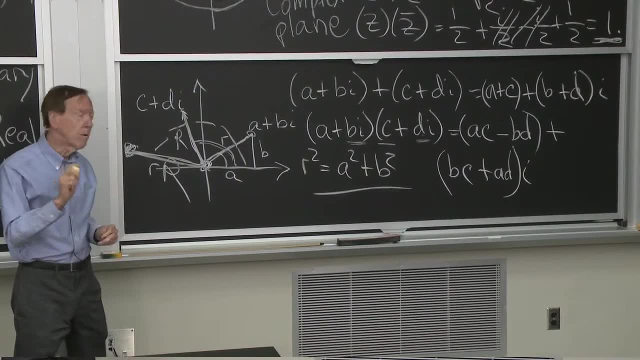 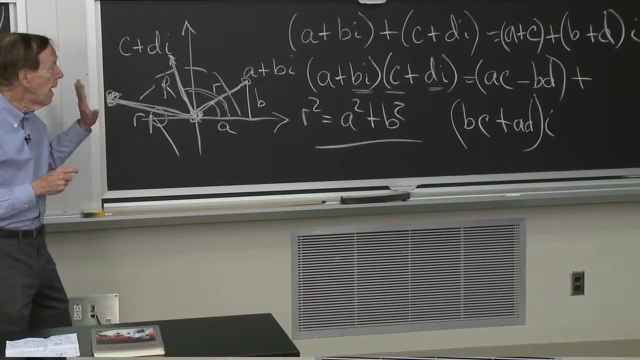 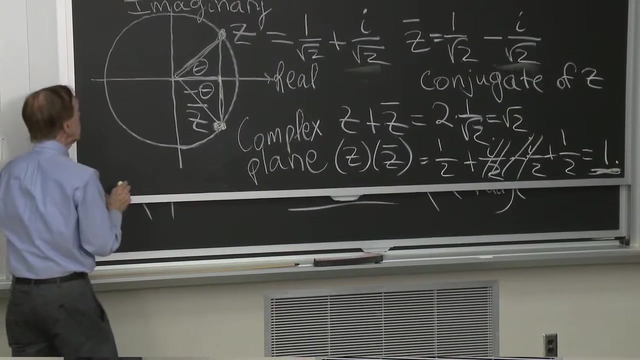 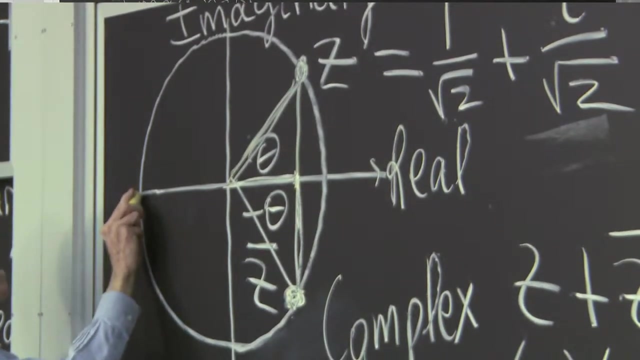 So my rule that I want to develop in the next step is Is multiply r's and add angles. OK, Can I leave you with some practice on these operations: addition and multiplication. Let me choose complex conjugates. So let me take the number minus 1 plus 1 half i 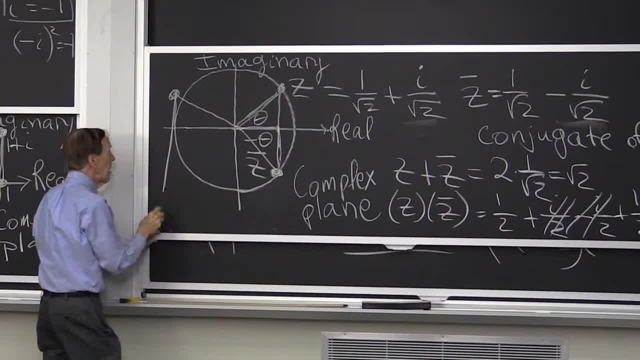 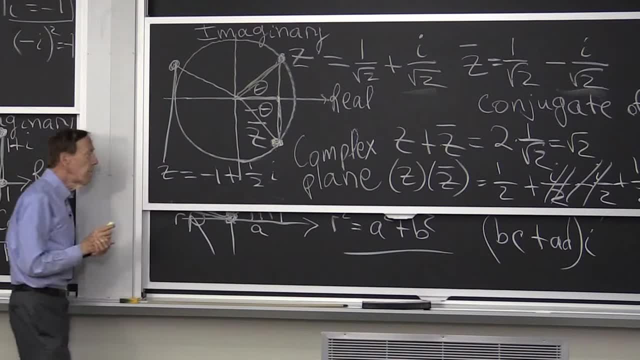 Would you say about there? So that'll be a number minus 1 plus 1 half i And I want to ask you: tell me what is z bar, it's conjugate, What is z times z bar? What is z plus z bar? 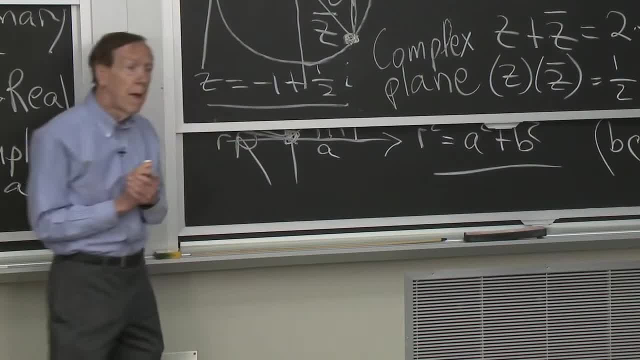 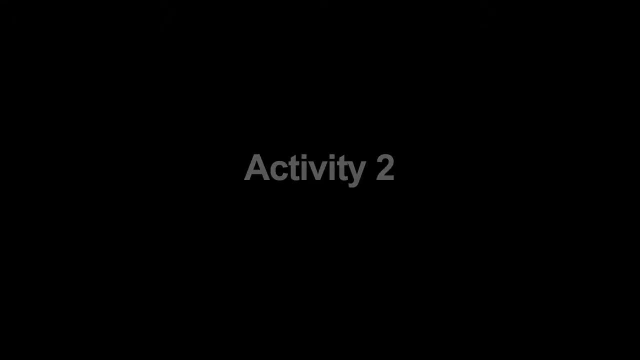 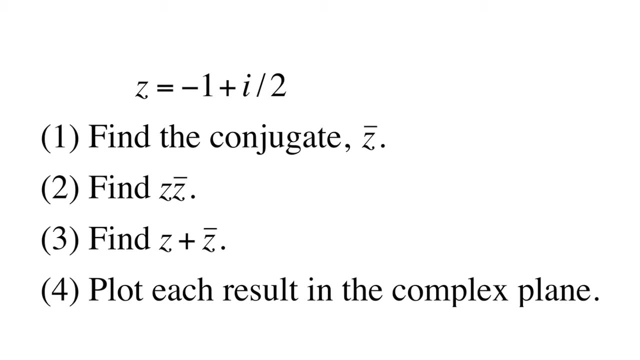 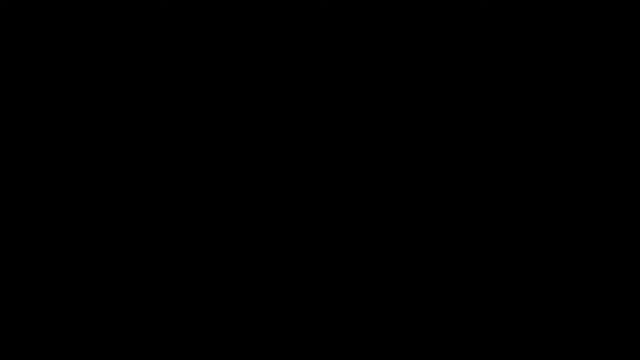 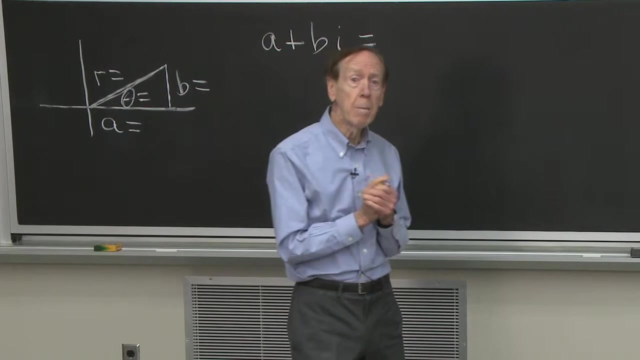 Just do everything you can with that complex number, and then we'll come back to the beautiful way to see multiplication. Good thanks, OK, this is the moment when we multiply the right way, using polar coordinates. That means, instead of the real part a. 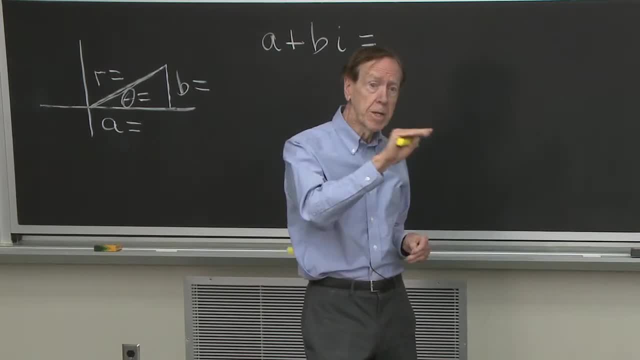 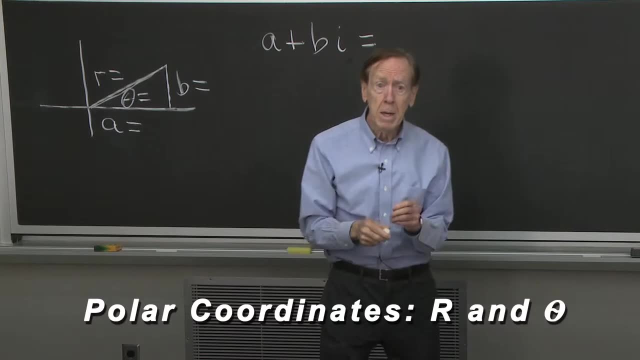 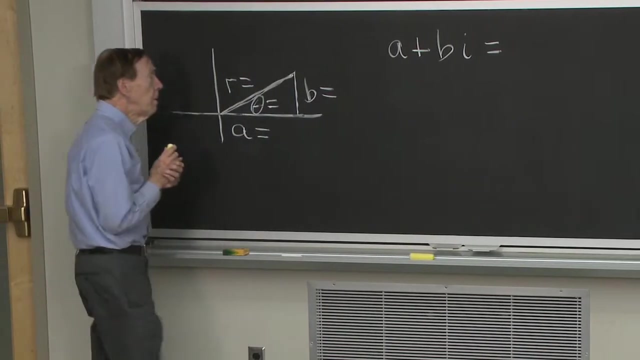 and the imaginary part b. I'm going to use the distance r and the angle theta. The polar coordinates are r and theta. Let me connect those to a and b, So r then in this right triangle. here's my a plus bi. 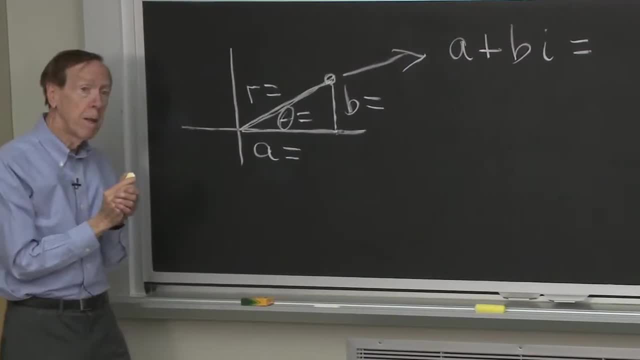 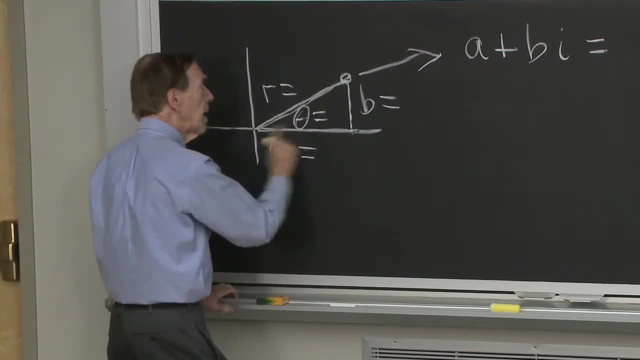 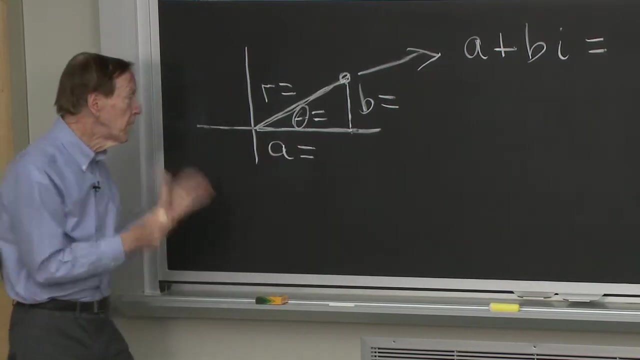 I go: real part a, imaginary part b, Those are the rectangular coordinates, And now I want the polar coordinates, r and theta, And I want to connect those. Well, it's pure, I've got a triangle here, a right triangle. 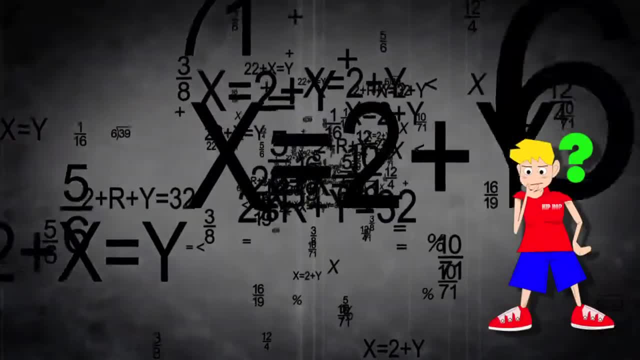 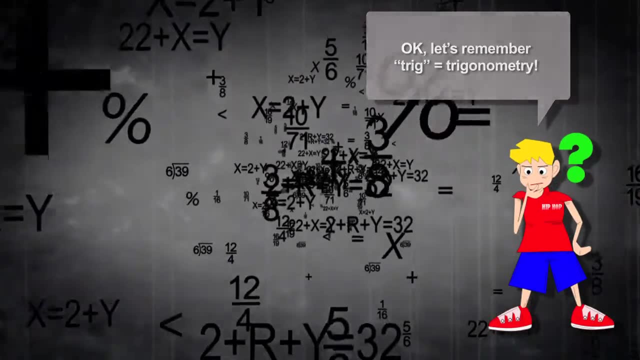 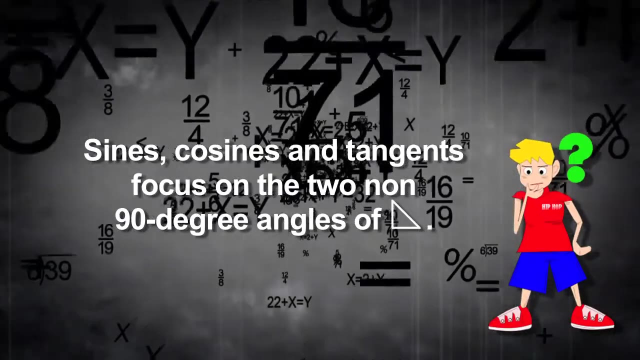 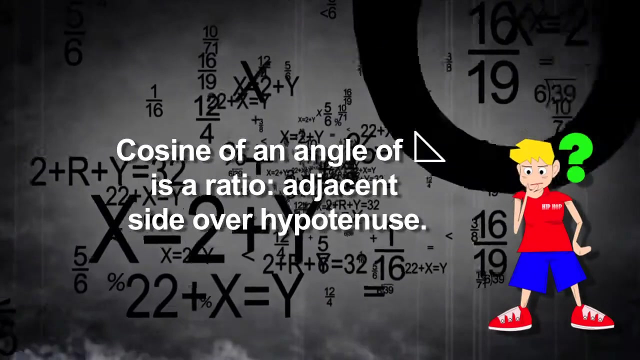 So it's just trig. Let's try that on our ball, Sort of On. this started, You want to do another one? I'm going to do this. Take this yard cause. I already laid it Between evenлан- seen more r and theta. 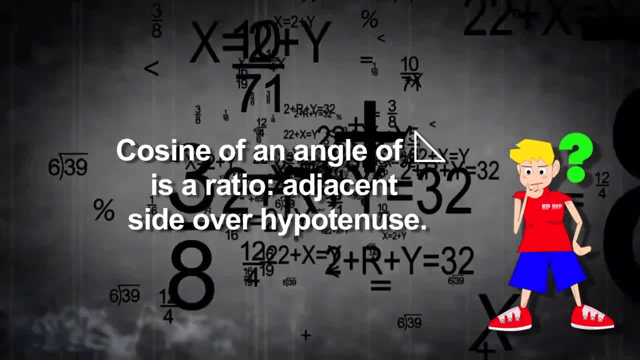 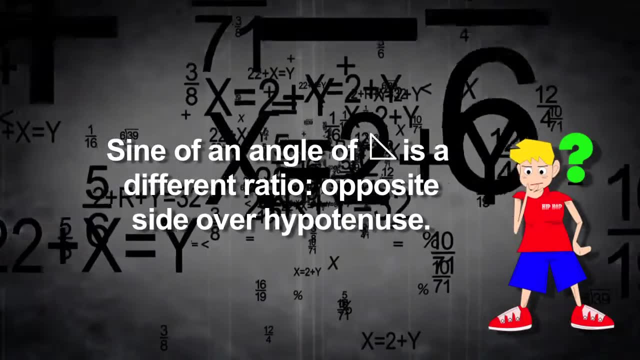 You can also put this here- than you need. Since you're going to do this, you're going to need r and theta. Right, you didn't start the torsional angle, so again, I'm going do r and theta. Let's try. theiento 고. 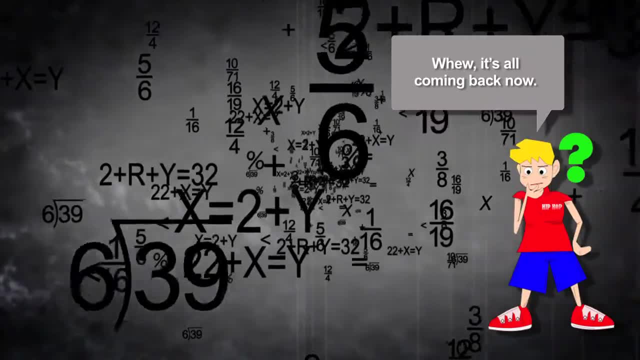 Given this R Document t. for two of these you add up the anarh textbook. if r and theta, what would r and theta do? That's a constant of than I need. That's why all q sine comes out of than I'm getting Musik. 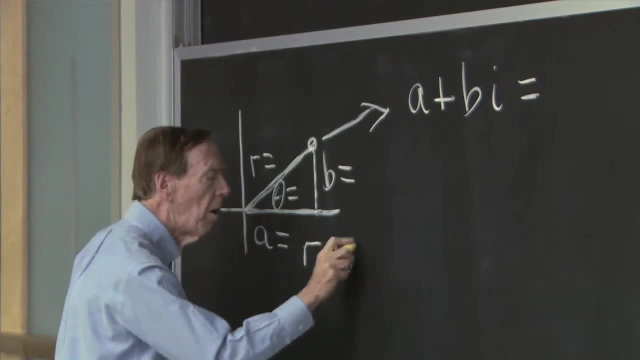 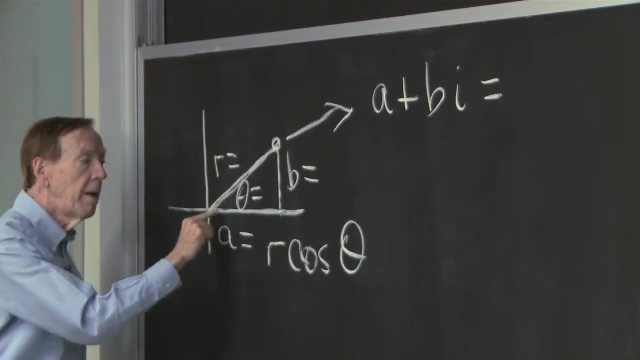 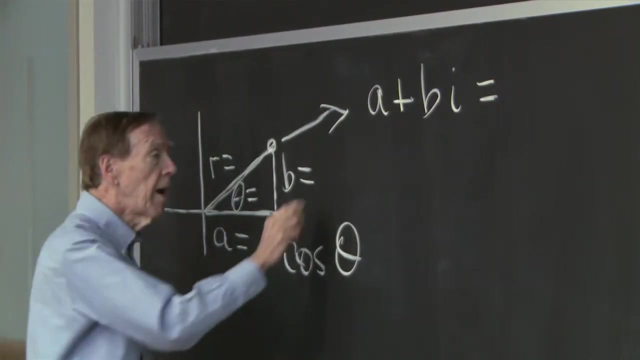 If I's have二 rho, that's greater than square root, something times the cosine right. That's the definition of the cosine, of that angle: The A- the near side divided by the hypotenuse, And B? r sine theta. 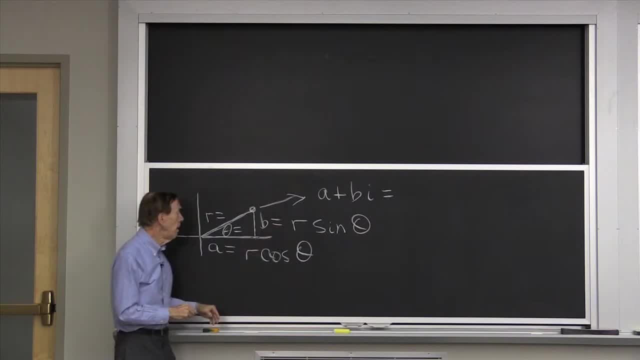 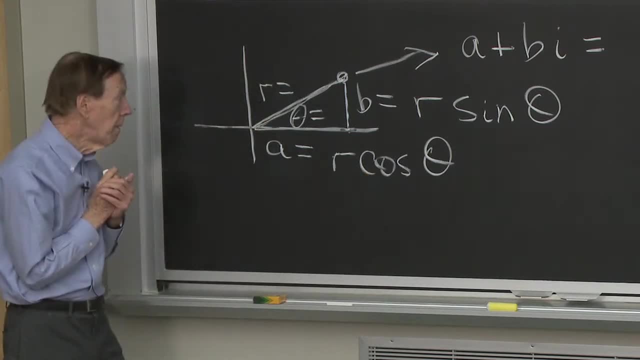 So when I know r and theta, this tells me A and B. Now suppose I know A and B, which is where I start. If I know A and B, what about them? Now I want to find the polar coordinates r and theta. 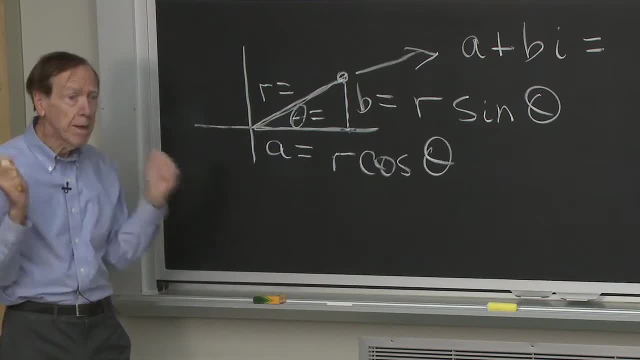 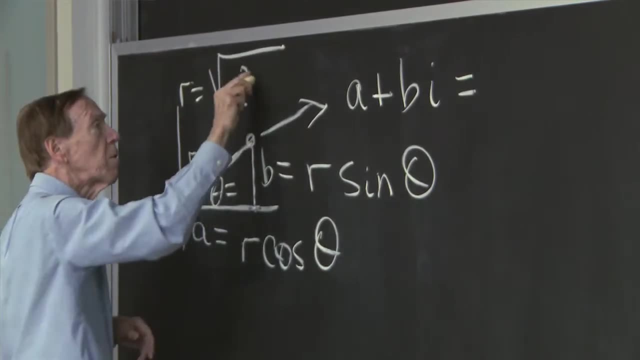 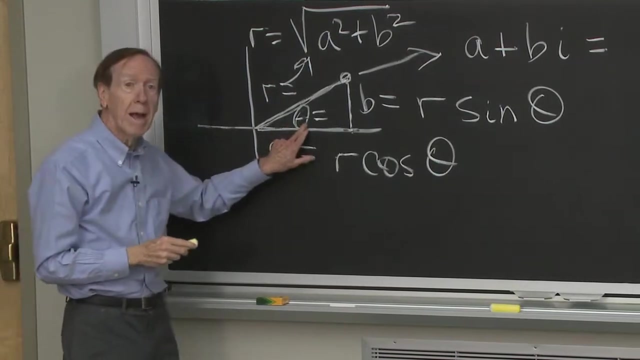 So r is the hypotenuse, And Pythagoras saves us again: r is the square root of a squared plus b squared. So that's the answer for r. And what about that angle theta? Well, I certainly don't have room. 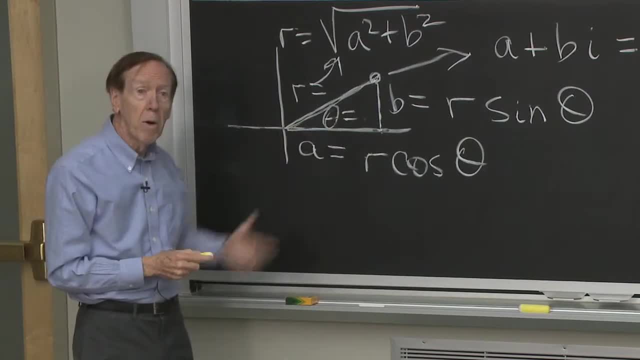 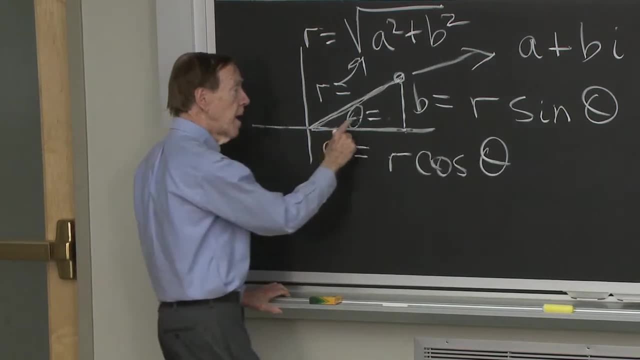 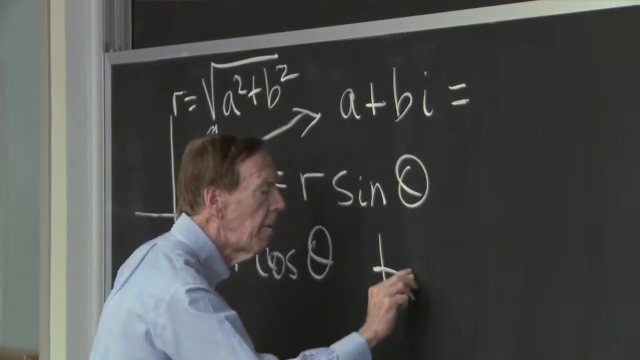 to write the formula for theta in there. What do I know about theta? If you tell me A and B, I know that the tangent of theta, the tangent of that angle, is the opposite side divided by the near side. So tan theta, let me write it here. 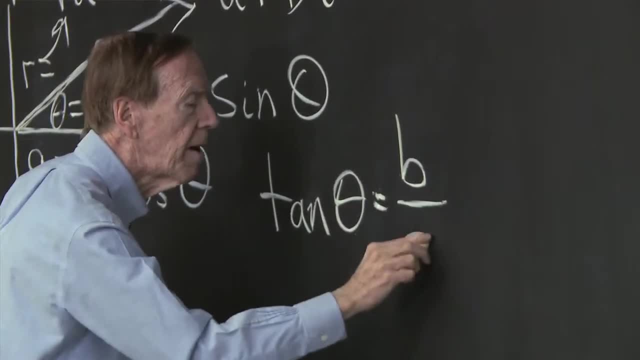 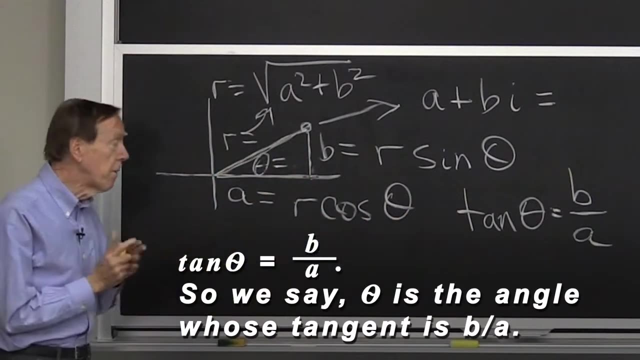 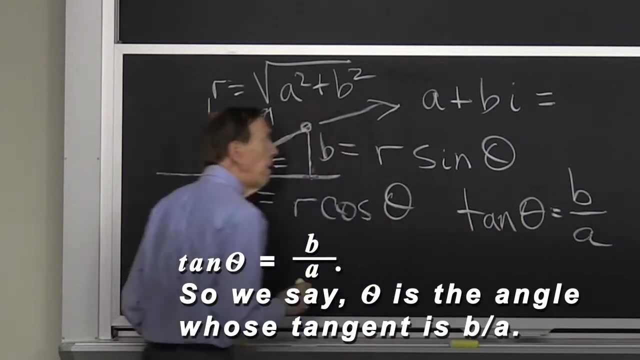 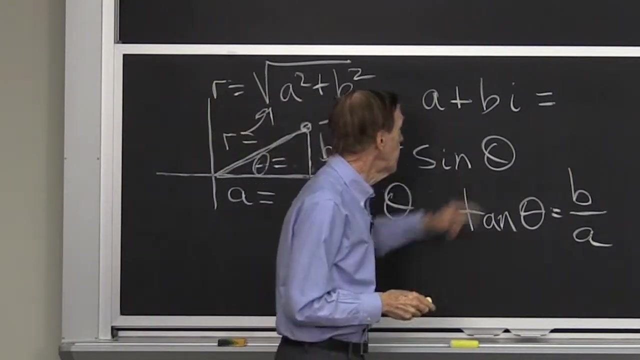 is B, the opposite side, divided by A, the near side. That tells me the main information about the angle, The angle theta. So those are the great formulas r and theta, B and A. And now I'm going to write this number, A plus B. I. 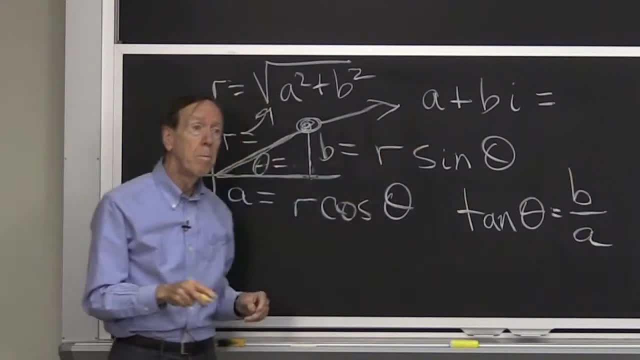 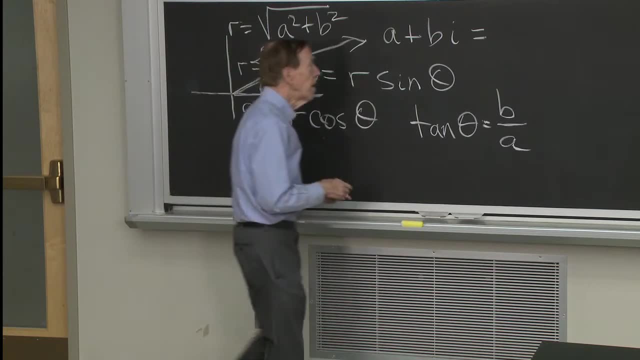 that number there in polar coordinates. So instead of the A and B I want to use the r cos theta and the r sine theta. So this is r cos theta, that's A And the I, B and A. The I is still there. 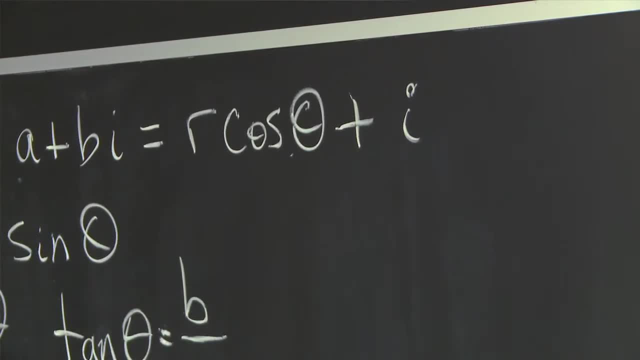 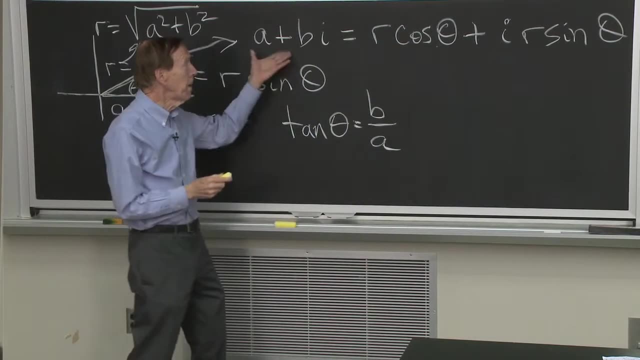 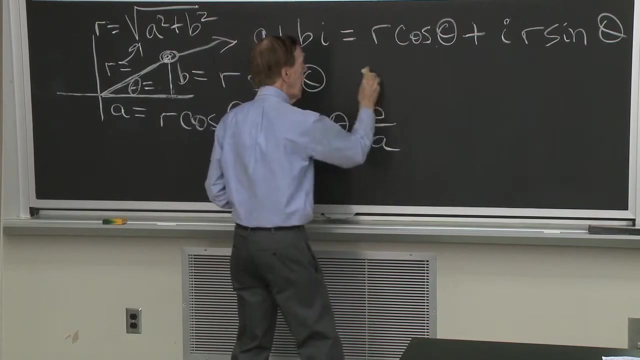 That tells me go up or down times. r sine theta. OK, You may say, well, that didn't look any better than A plus B I, But it is Now. first of all, everybody sees that I have an r in both terms. 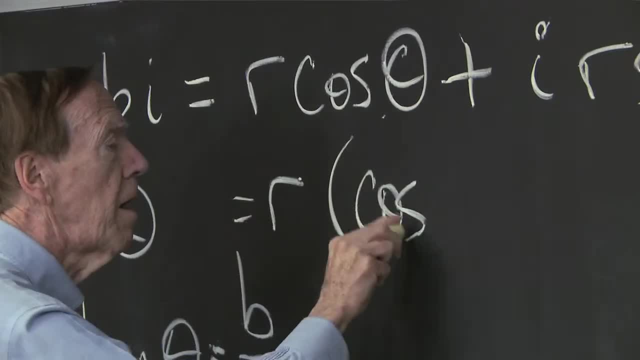 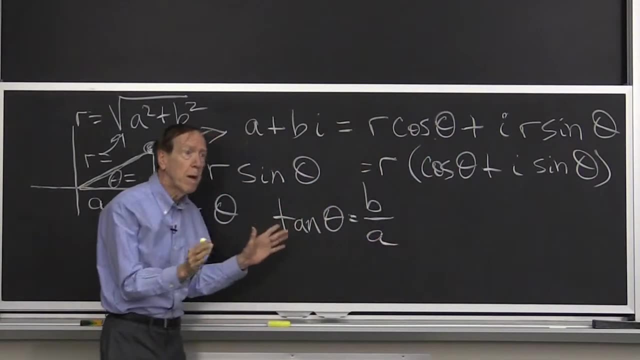 So I factor out the r, and then I have cos theta plus I sine theta. So now I'm separating the distance, part the r, which says how far it is from the angle, part the theta, which gives me the direction. 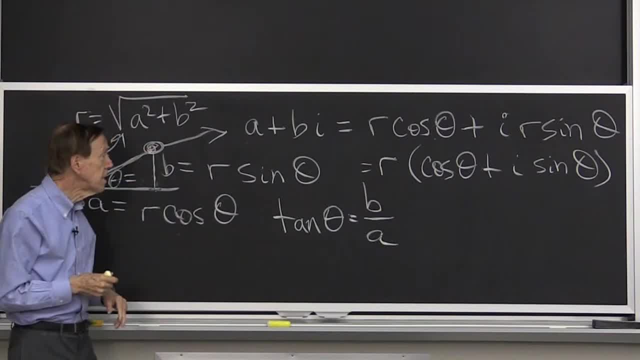 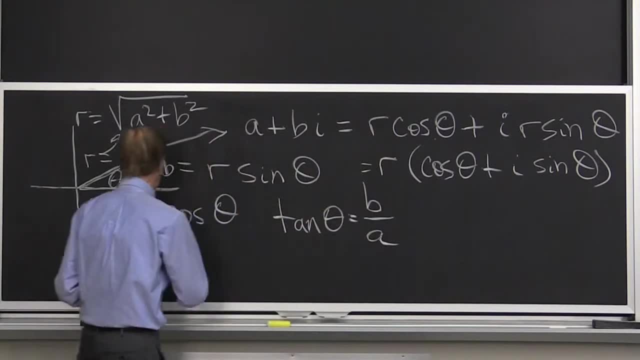 And the distance and the direction tell me where that final point is. OK, Here I'm ready to multiply. I'm ready to multiply that number. Suppose I multiply by itself. Suppose I multiply A plus B, I. I want to do this. 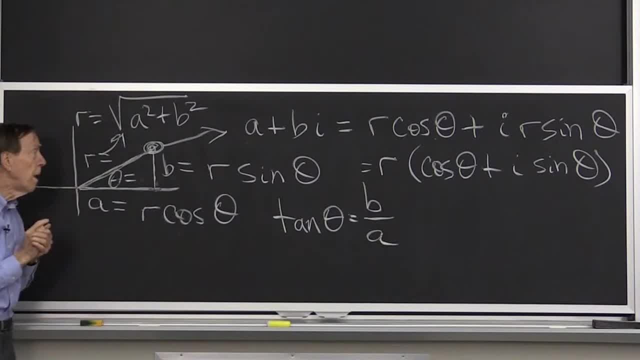 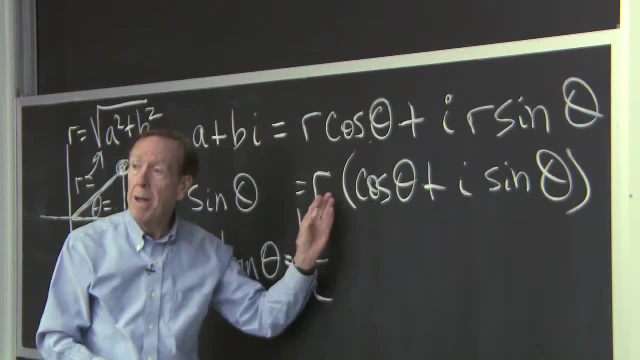 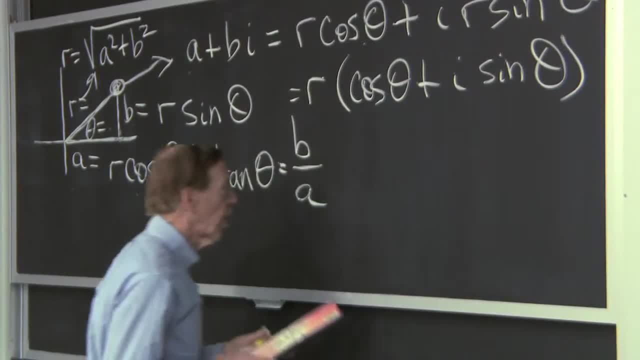 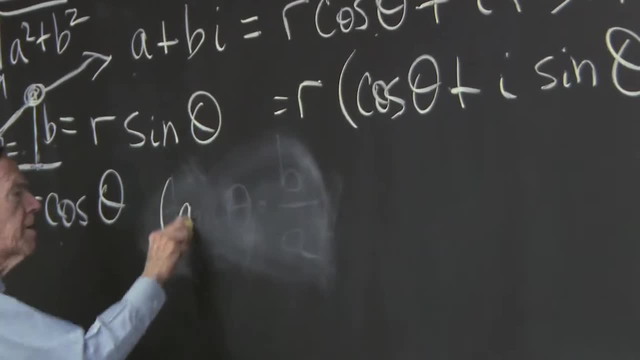 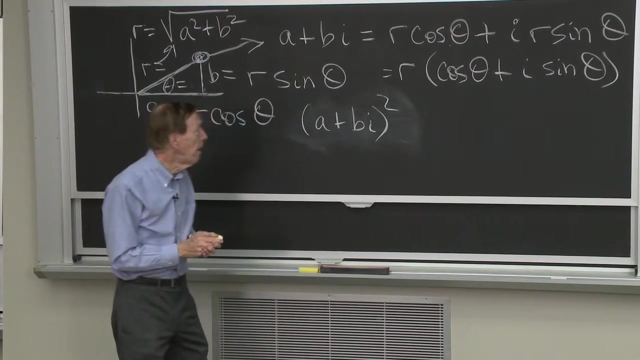 So now I'm ready, for let me take away tan theta, which is getting in our way, and multiply. So now I'm going to do A plus B. I squared just to show you the beauty of this. OK, Now, that's this thing squared. 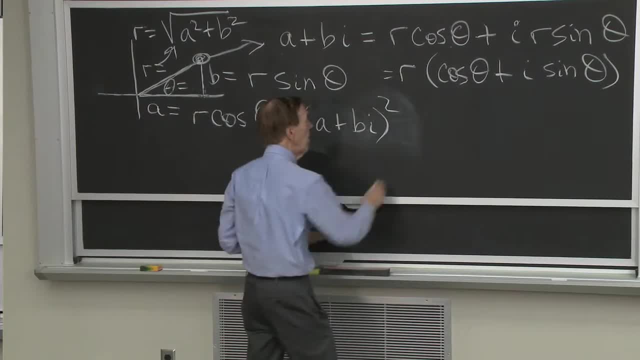 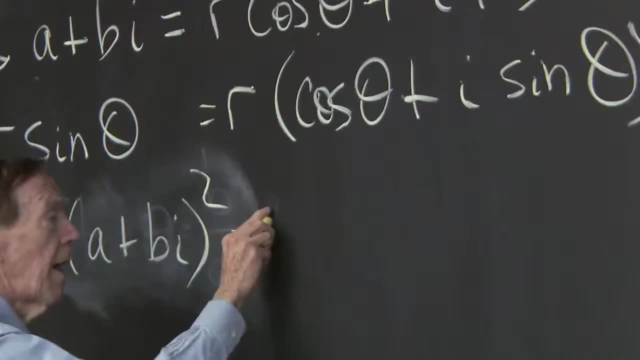 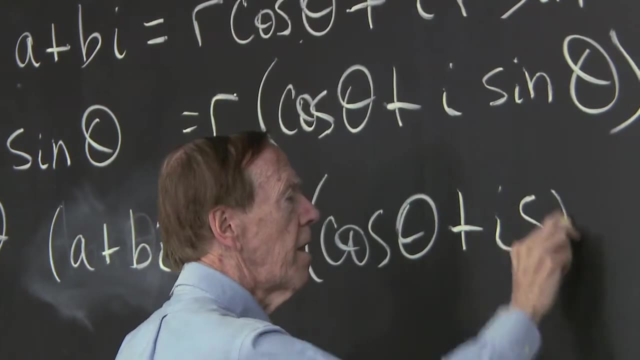 What do I get? I want to multiply. I'm going to multiply that by itself. So I get r. We'll multiply an r, r from one factor, r from another factor. I'll have r squared. And then this part: cos theta plus i sine theta squared. 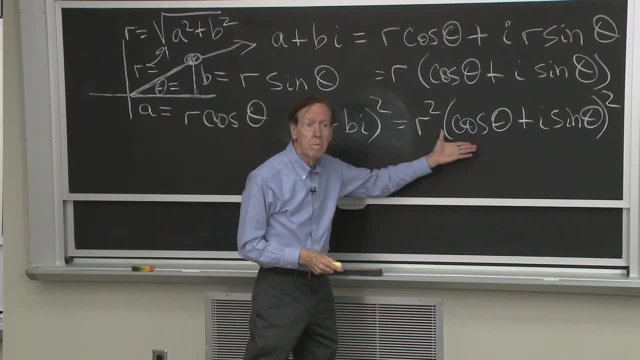 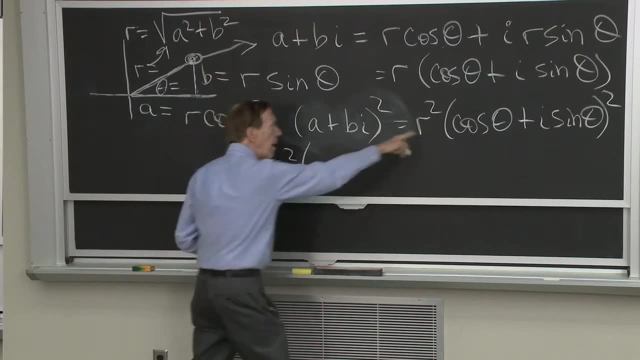 No problem. And now I'm going to get to the bottom of this part. So what do I have? I have r squared, And now can I just multiply that out the usual way: Cos squared- theta is real, Where else is real? 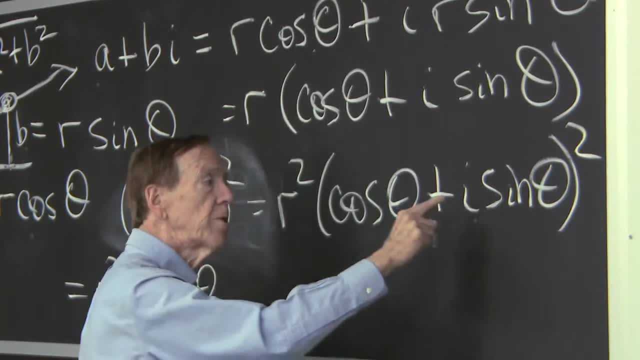 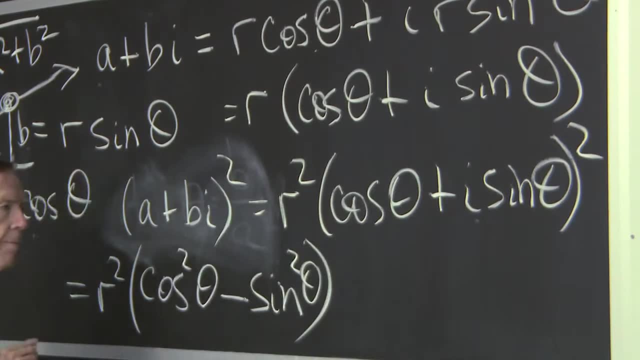 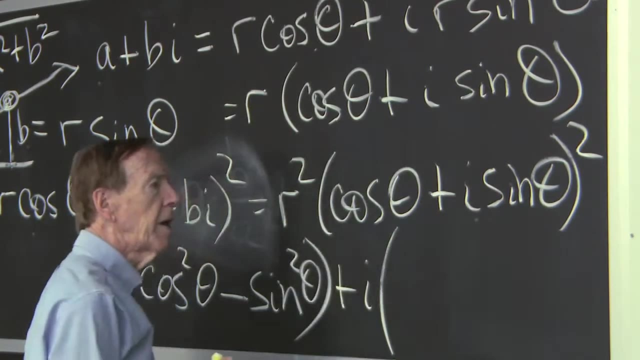 Have you got the idea? When this multiplies itself, it's real with the minus sign. So minus sine squared theta. And now I have the imaginary part. cos theta times sine theta? OK, OK, Very good, I'll put that in. 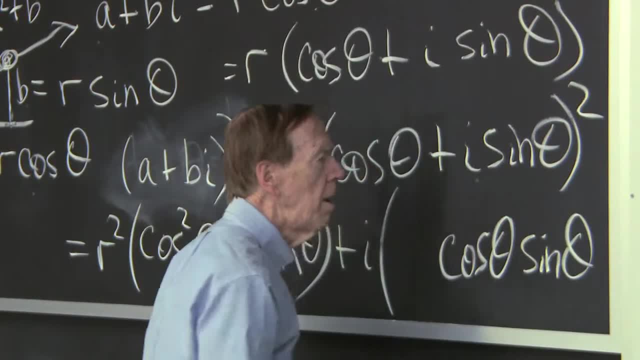 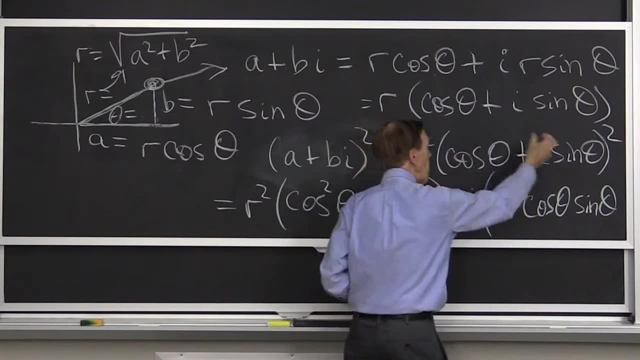 Cos theta sine theta. And another one right, Because I'm squaring So I have this times itself. So a cos theta will multiply an i sine theta And an i sine theta will multiply a cos theta. I have two of them. 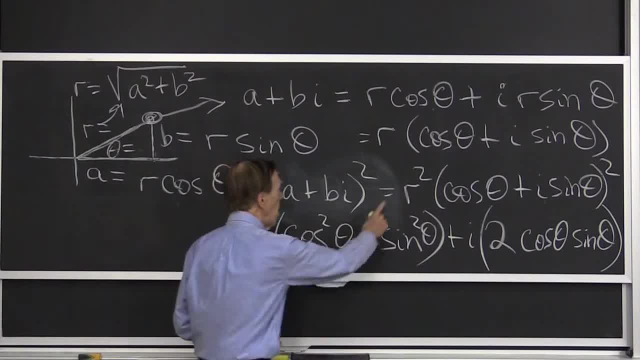 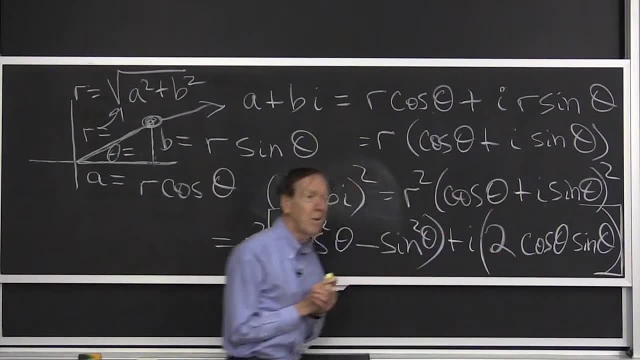 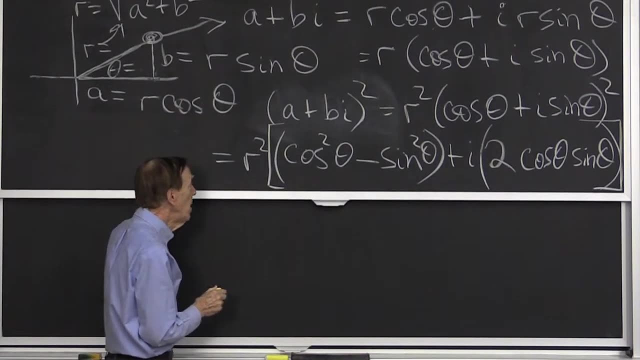 All right, OK. So r squared multiplies all that. So can I put a big bracket around Again? you're going to say This isn't better, but it is better, OK. So I have one more step. One more step. 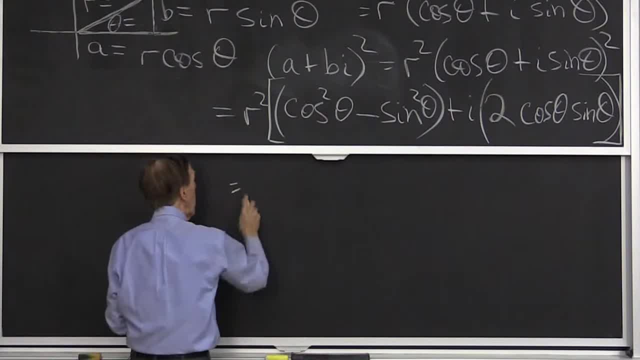 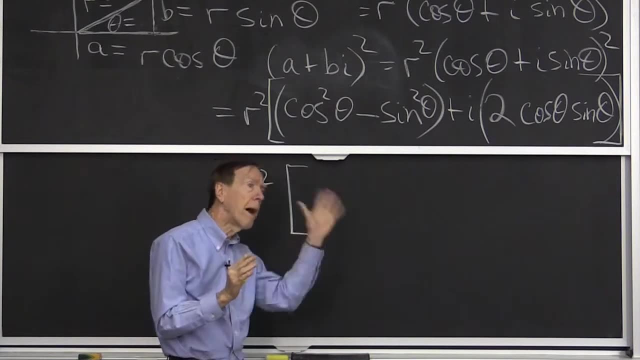 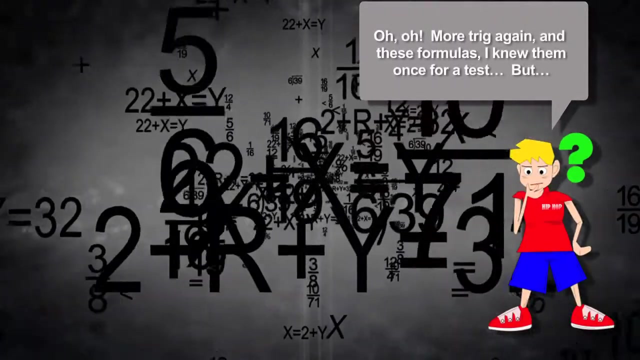 And it's going to come here And this is going to be the answer. The r squared is always good. What do you see inside those parentheses? Do you recognize two cos theta, sine theta. I'm asking back to trig formulas. So it's just going to be an i and a sine theta. 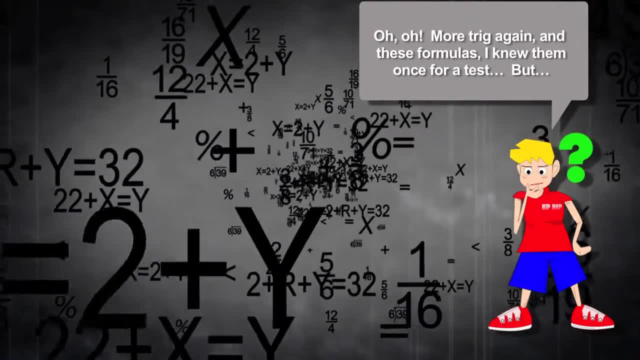 So I'm just going to say that r is an i sine theta, So I'm going to put this 2 to 1.. OK, So I told you. I told you that only 1 to 2 is an i times 10.. 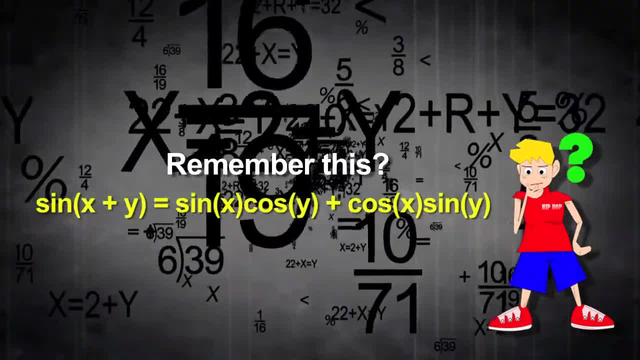 So one more parameter. So, if you remember this, you didn't understand the equations, So it should look like this, And I'm going to put this 1.. All right, Let's put this 1 here, And now I'm going to put this 3 here. 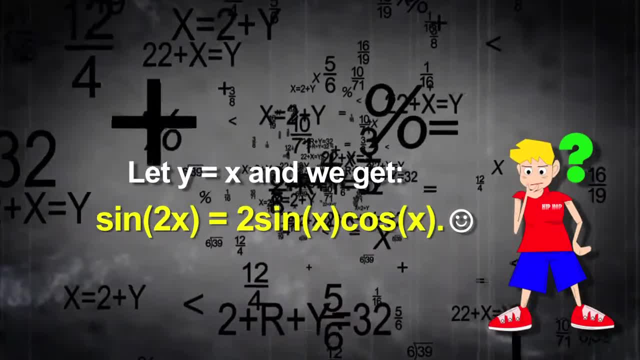 So this 1 is the total for 1.. I'm going to put it in this n plus 1.. What I'm going to do is put this 1 here for the one on the left. that's going to be the plus 2, plus 1 to the one on the right. 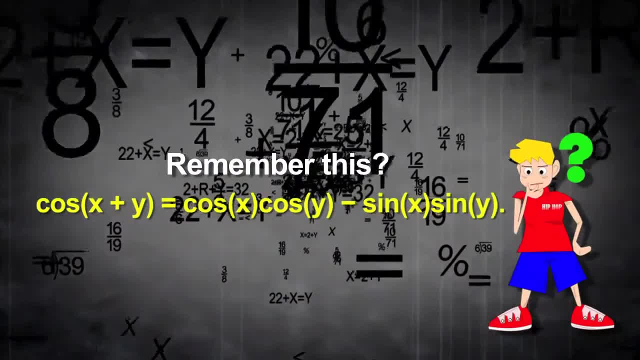 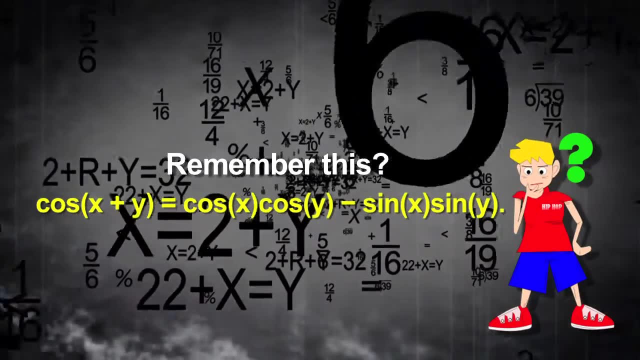 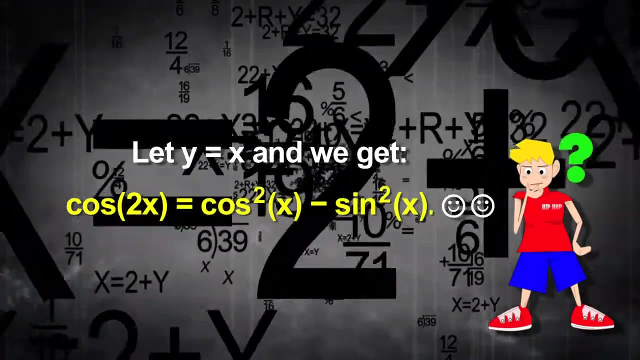 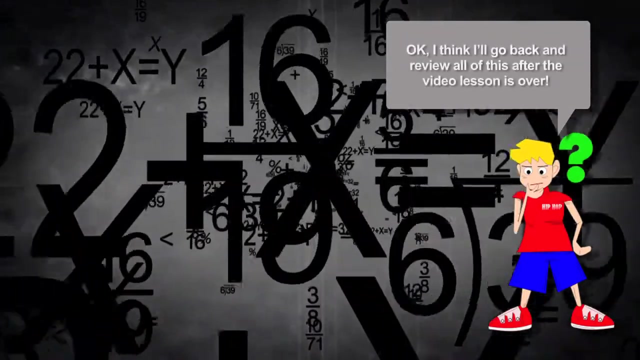 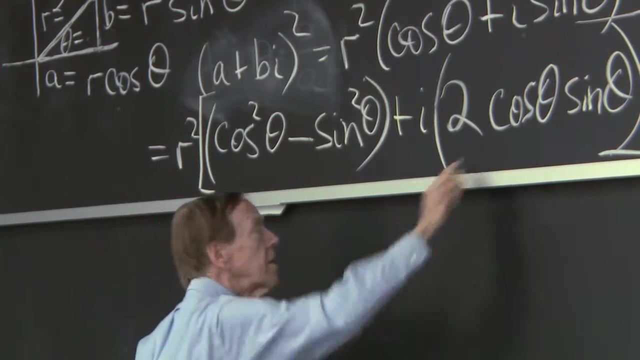 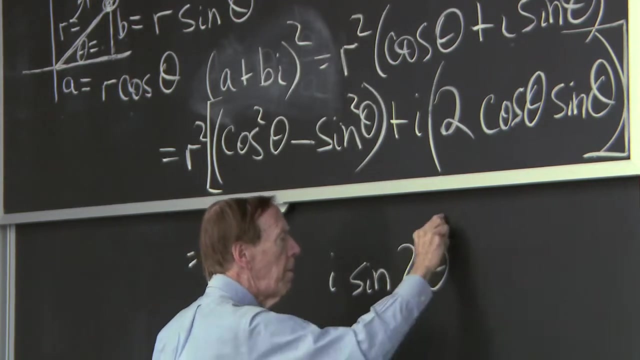 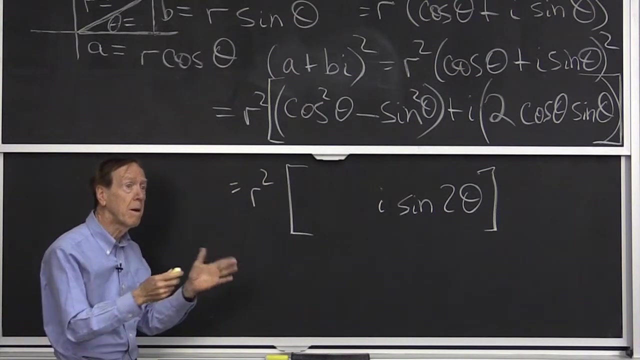 All right, Thank you for watching. That is the same. that i part is the same, as that's the sine of 2 theta. And do you recognize this thing? Cos squared minus sine squared, There's the trigonometry for the double angle formula. 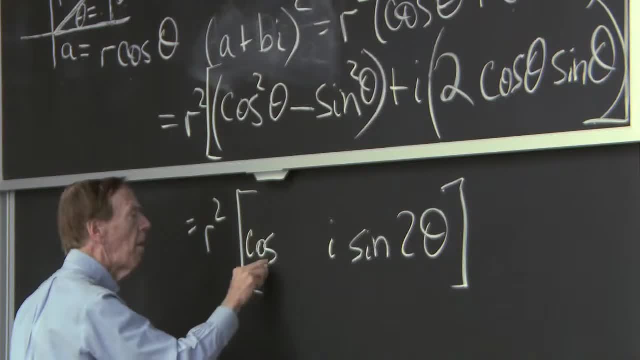 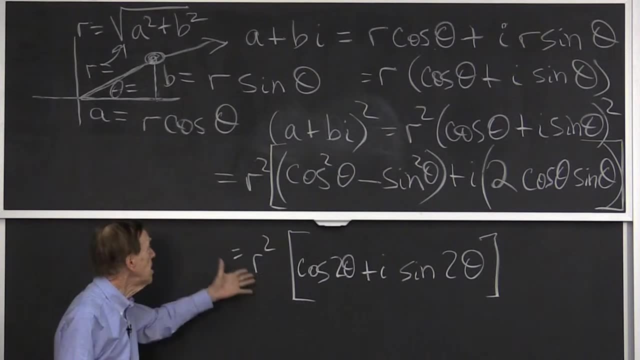 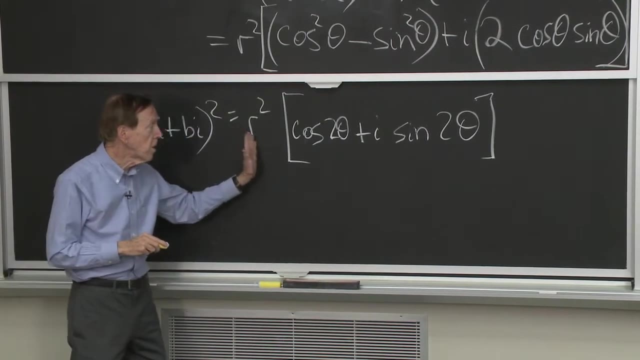 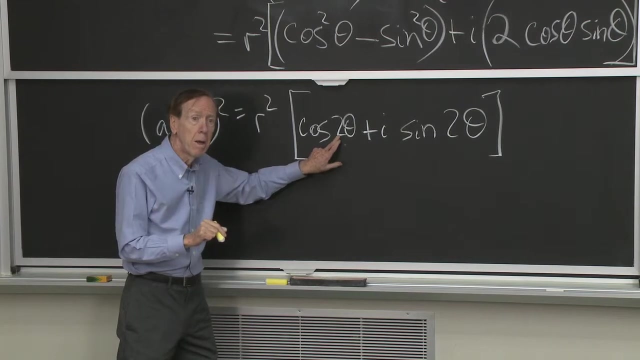 tells me that that is cos 2 theta. Now look at that answer. So this is z squared. I've squared it here. a plus bi squared is what I did, But I did it in polar coordinates, r and theta, because now I see that the r's multiply and the thetas add. 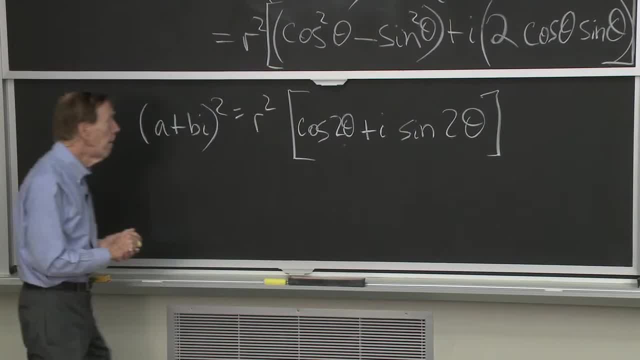 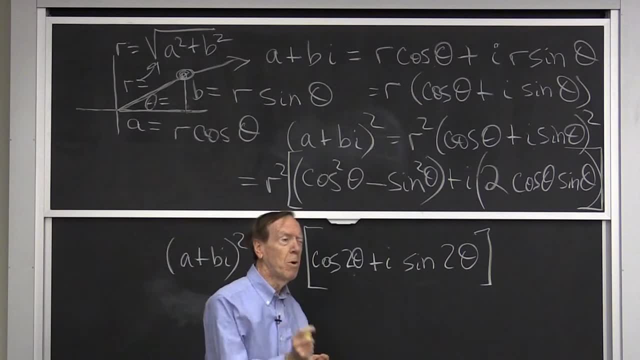 One theta adds to the other theta, to give me 2 theta. And in general, angles add numbers, multiply. OK, I have one more improvement to make on this multiplication And it comes from A brilliant formula of Euler, Euler's great formula. 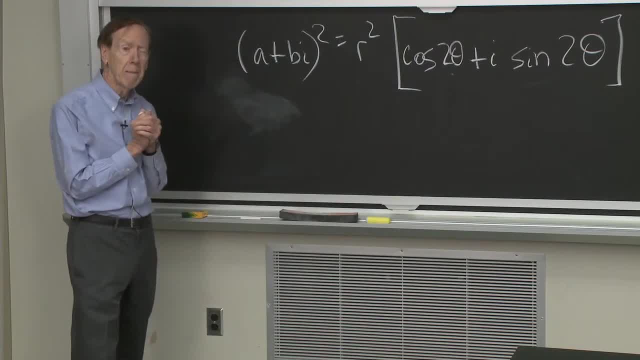 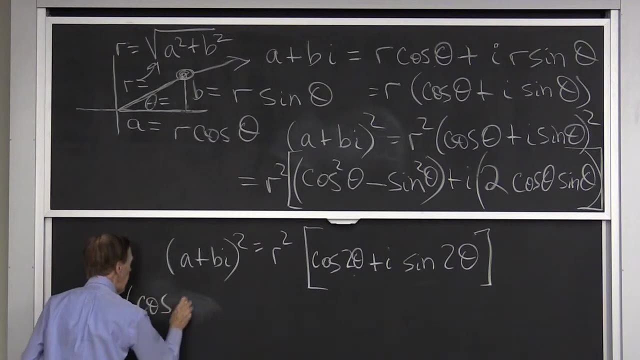 It's one of the most beautiful formulas in all of mathematics, So let's see it here, And I'll present it more fully after a break. OK, so I want to write this: r cos theta, I'm going back to cos theta and i sine theta. 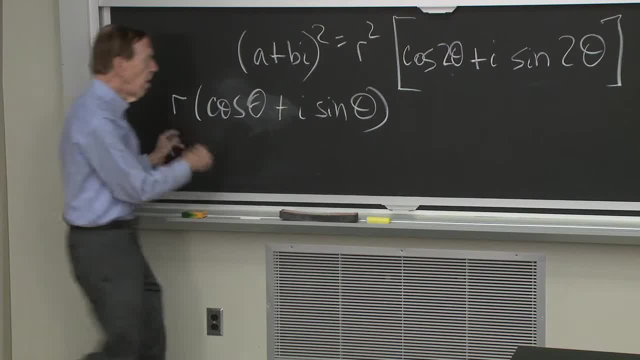 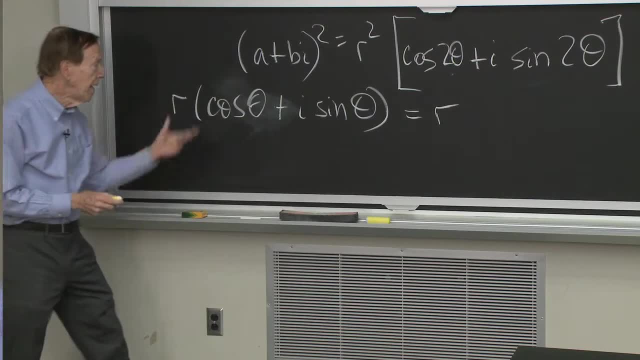 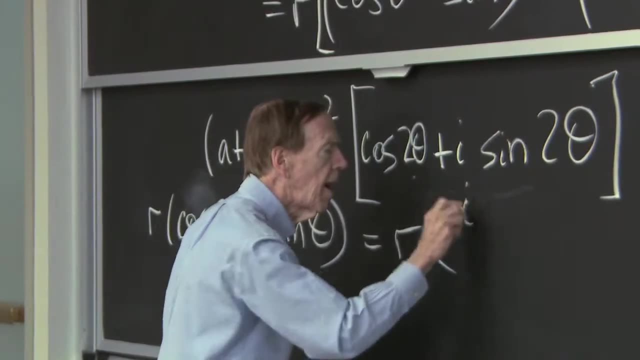 That's our complex number, a plus bi. This is the r part. I'm very happy with the r part, But Euler had a great idea for the angle part. He realized that this combination is exactly the same as e to the i theta. 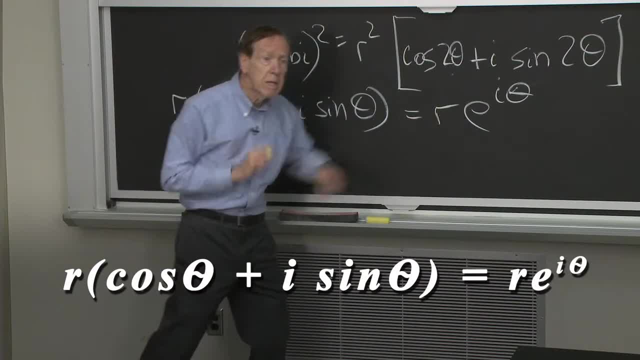 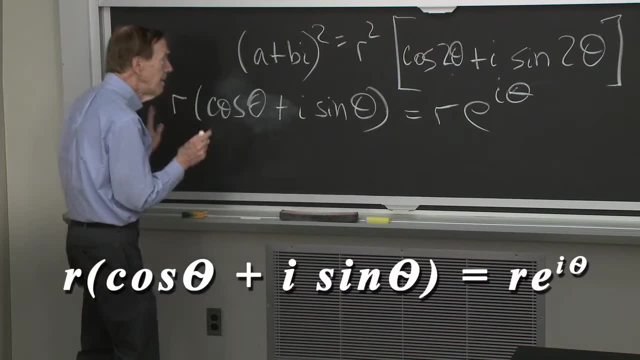 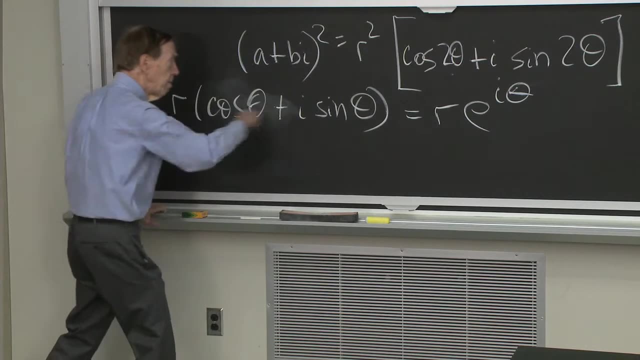 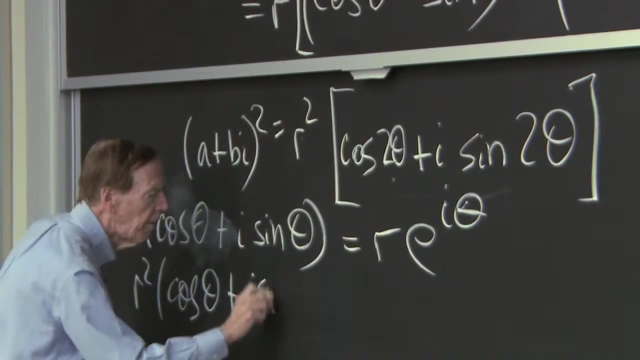 The exponential, this is the 2.7 something, but taken to an imaginary power, And I'll show you. I'll show you why that is correct. And then let me multiply by itself. So r squared times cos theta plus i sine theta squared. 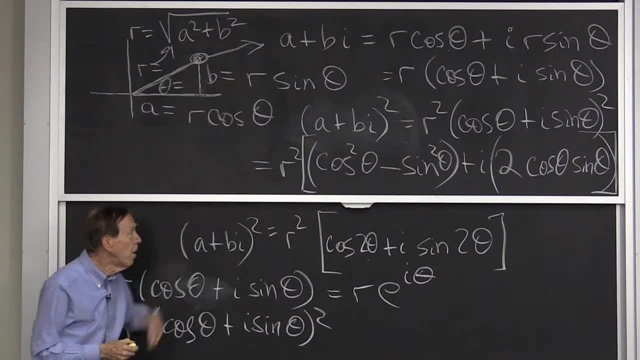 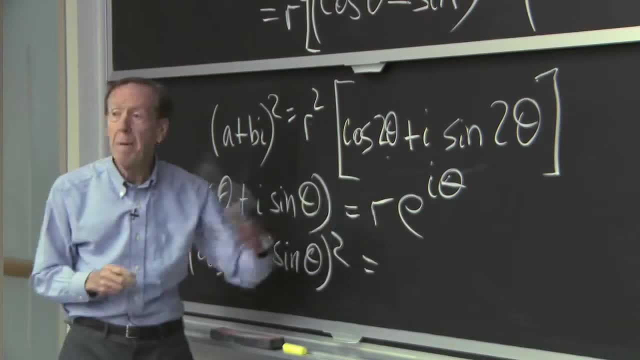 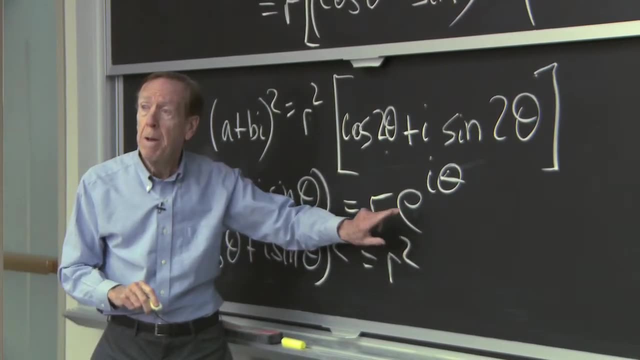 That's what I did out with your help on that. That took time, But let me just square that number. Can you multiply that number by itself. r multiplies r to give you The r squared we expect. e to the i theta times. e to the i theta is. 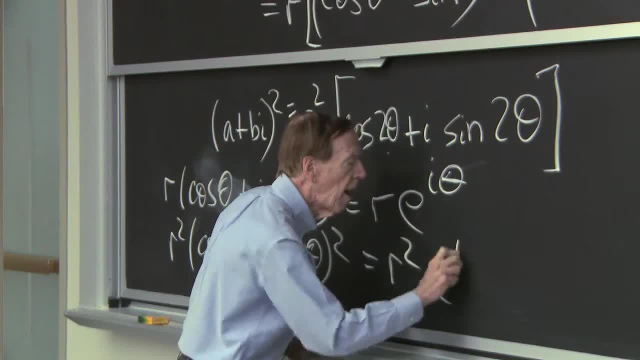 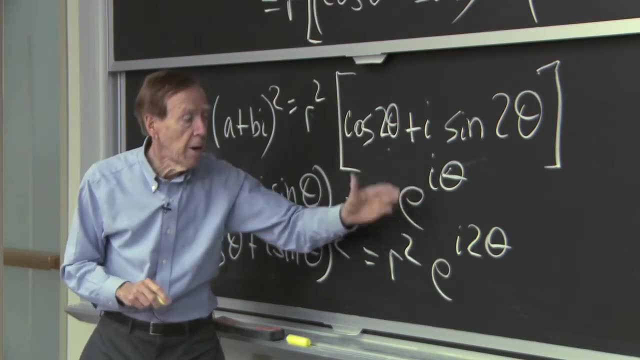 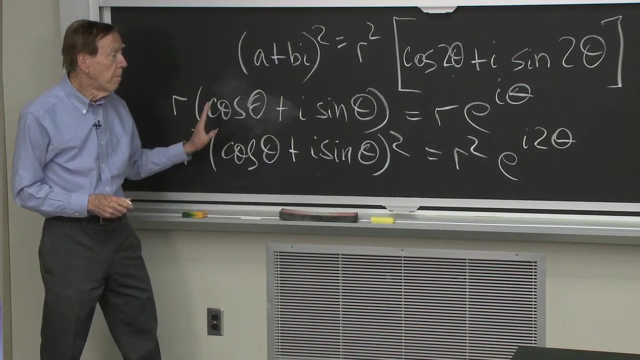 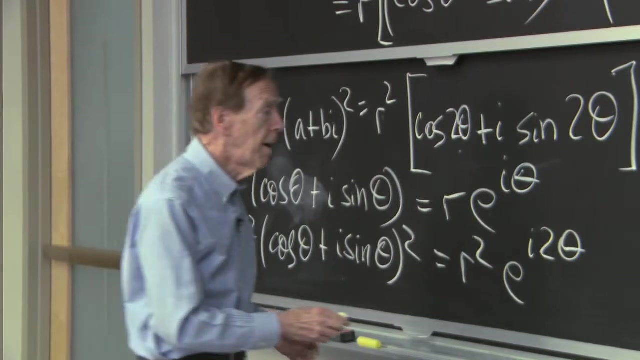 Exponents: add e to the, i to theta. I added i theta to i theta and got two of them, And that's exactly the right answer. So this is the way to multiply: Multiply distances, add angles, Thanks, So let me leave you with a specific example then. 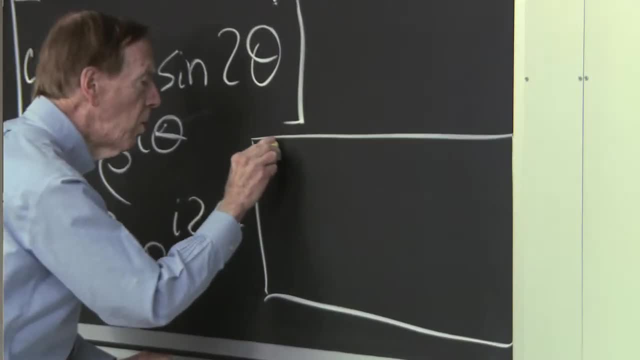 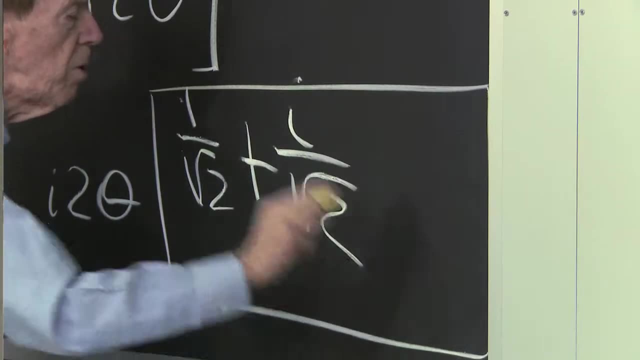 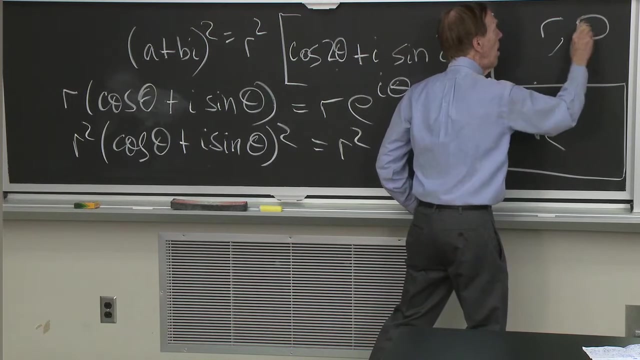 Take our favorite number, z. that number we've been calling z, 1 over the square root of 2 plus i over the square root of 2.. So you can see a, you can see b, Find r, find theta and find e to the i theta. 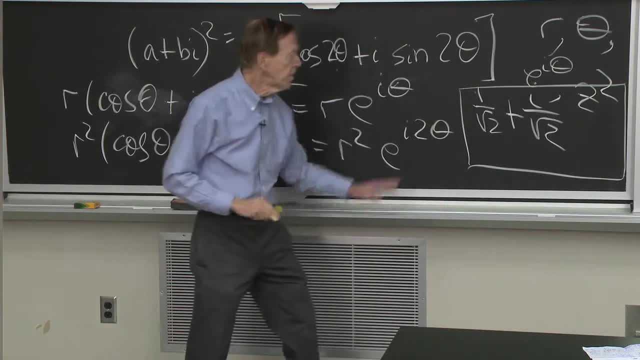 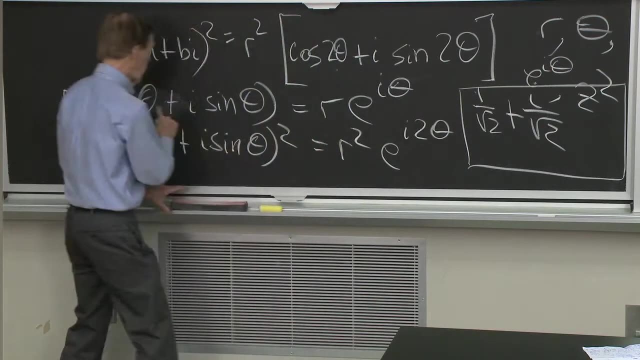 And find z And z squared. So this is our z, that complex number that you know, at the 45 degree angle. that I've helped you. So it's got an r, It's got a theta. The combination cos theta plus i theta is this: e to the i theta. 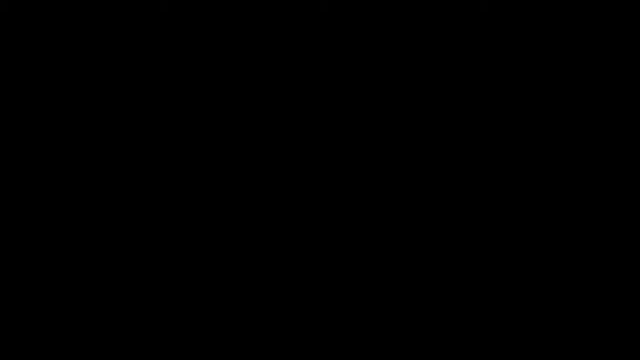 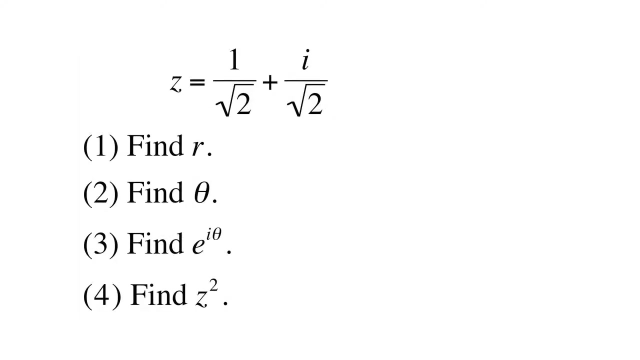 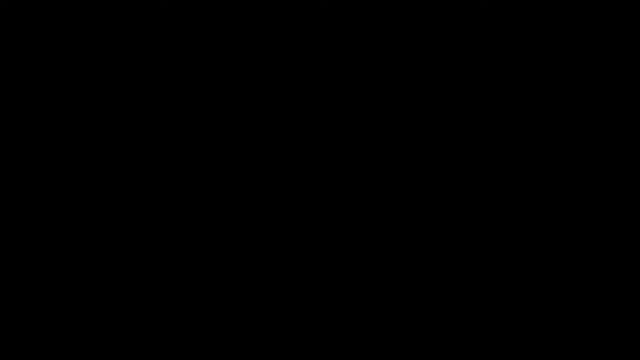 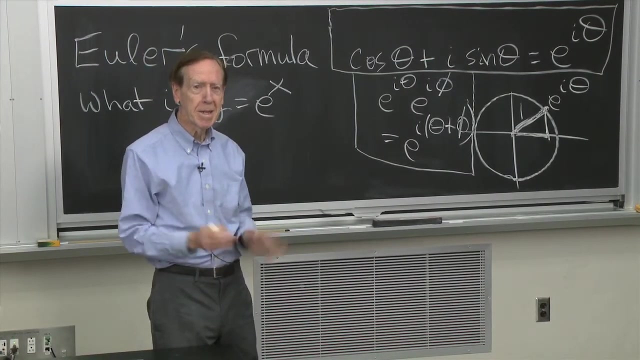 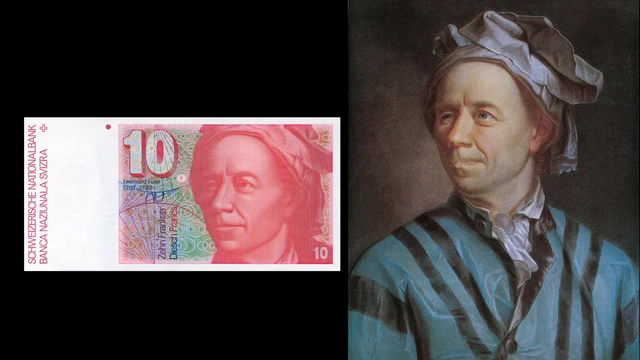 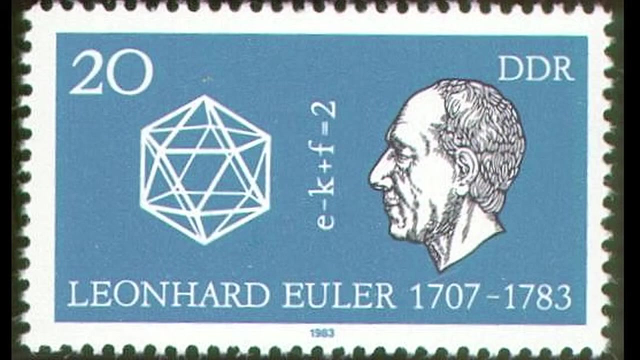 And then you can square it. Thank you, OK, I have to say more about Euler's great formula. This is the heart of complex numbers. He was from Switzerland but he worked in Russia And he wrote in Latin, And he wrote more math papers than anybody else. 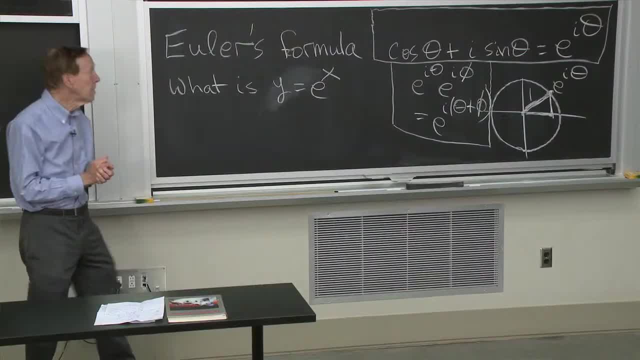 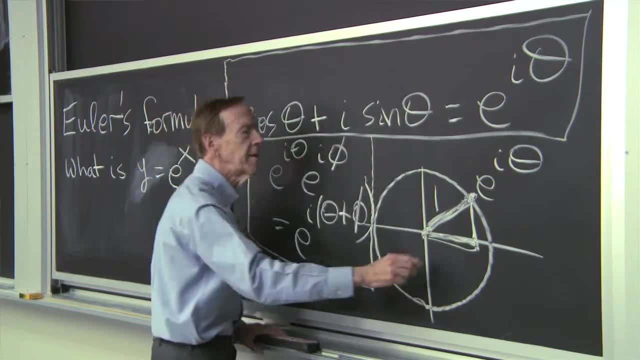 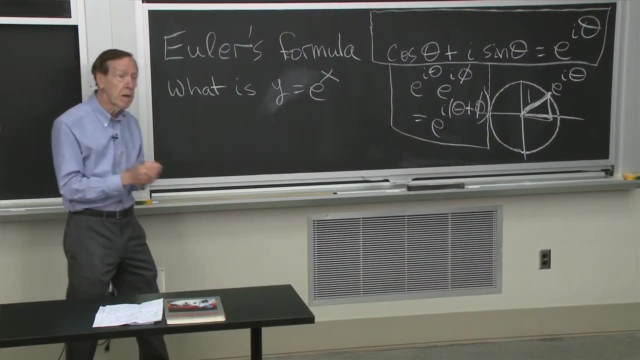 And he did great work. So here's the formula that we ended up: The combination of cos theta- this part across plus i sine theta, is that number, The distance is certainly 1.. The magnitude, because cos squared plus sine squared is 1.. 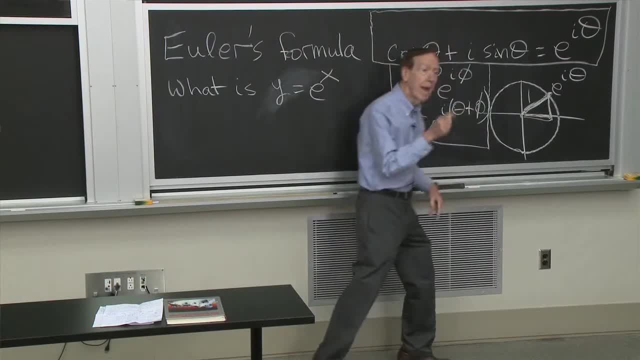 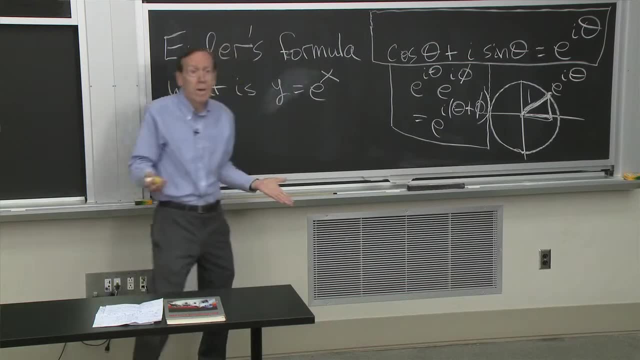 The hypotenuse is 1.. But the and the angle, And the angle is theta And we can express that number. Euler says as e to the i theta. So what could e to the i theta be e or e squared or e cubed? that's tricky enough. 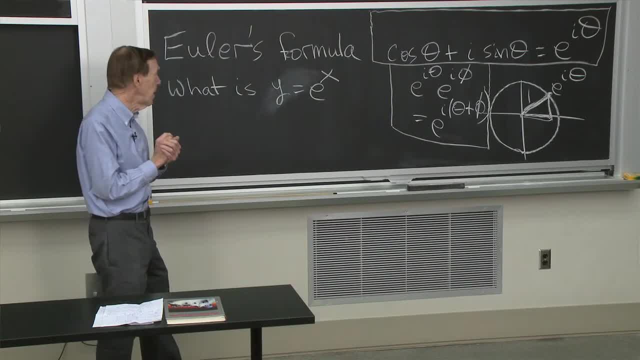 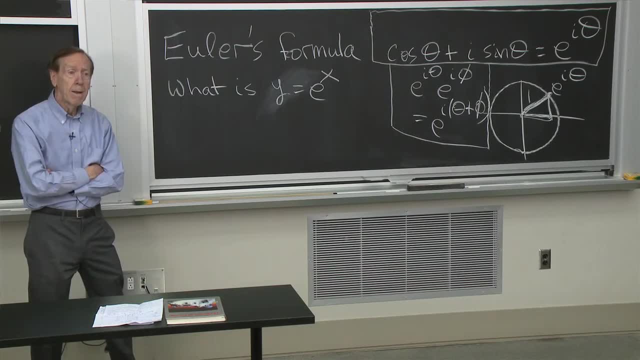 But here we have an imaginary number, i theta in the exponent. So let me start with a real x And just remember what is e to the x. This is the most important function. e to the x is the great function of calculus. 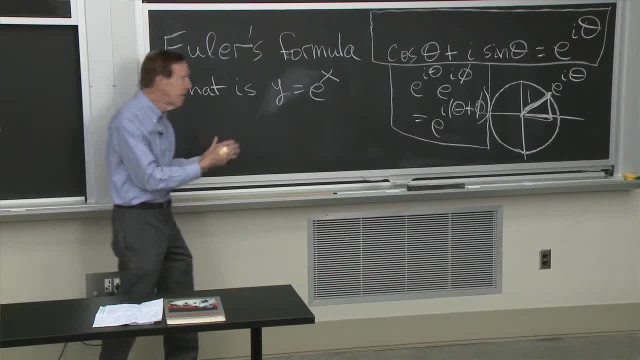 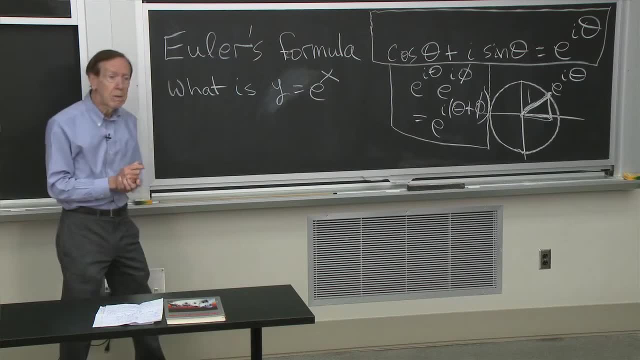 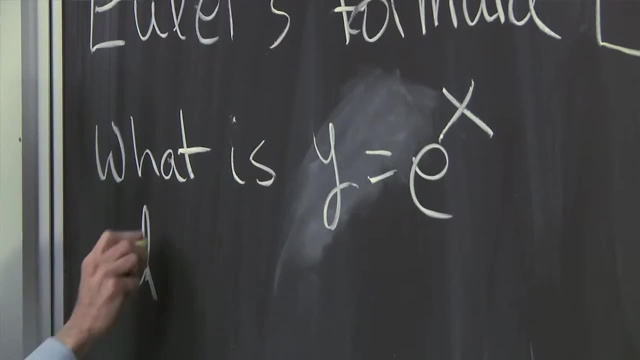 calculus. It's the function that you can't create in just simple algebra with some quadratic or cubic, but we can create it using calculus, And so I'll give you the calculus part. Calculus is about derivatives, And this function, e to the x, satisfies the amazing equation. 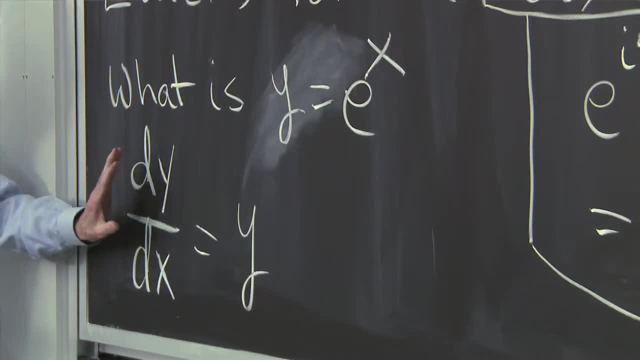 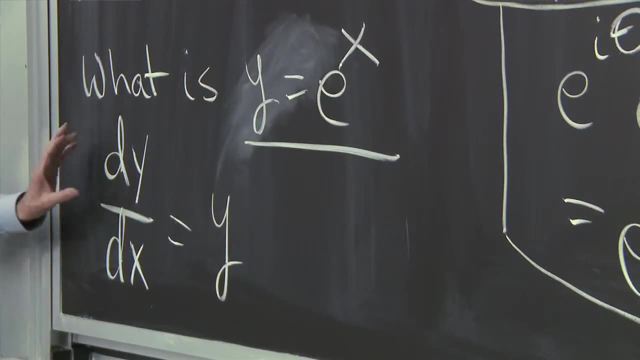 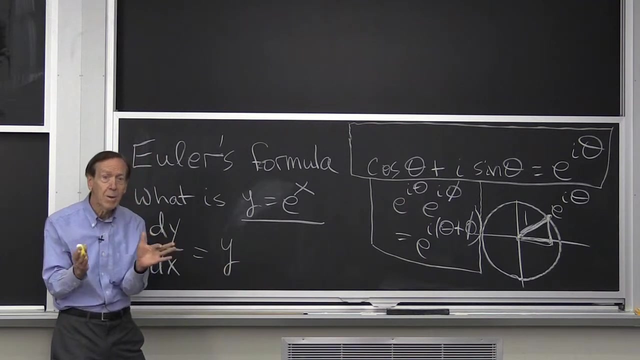 dy, dx equal y. So from the point of view of calculus, the key to that function, e to the x, is that it solves that equation. But I want to tell you, well, I can't do it in algebra, but you'll see where I have to carry algebra to an extreme. 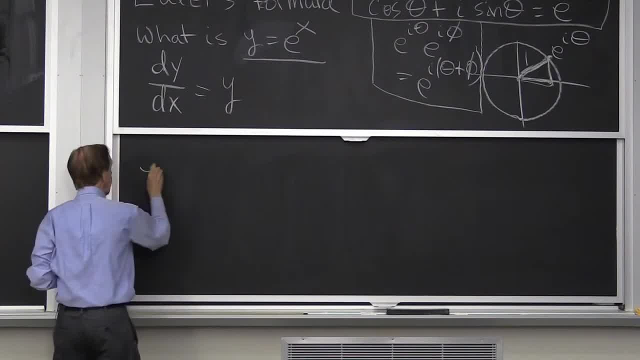 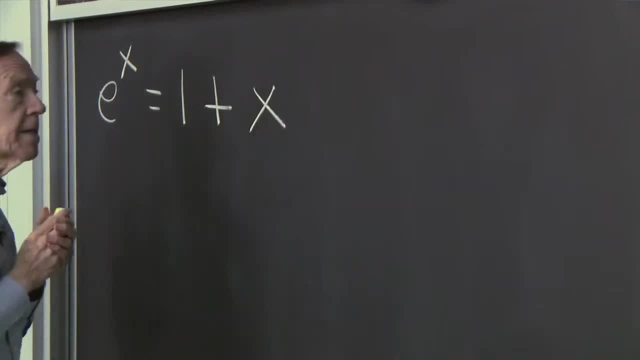 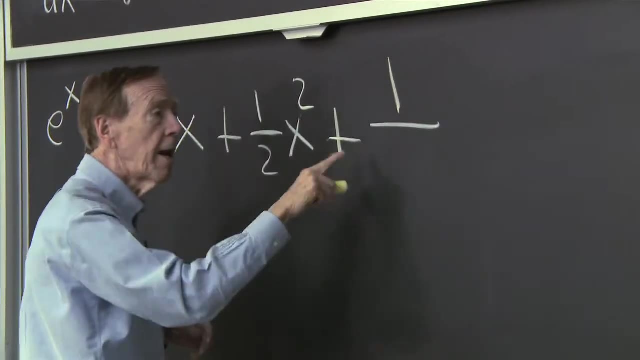 Let me tell you what e to the x is. e to the x is. it starts with 1.. And I need an x, And I need a 1 half x squared And I need a 1 sixth. That next one is going to be 1 sixth. 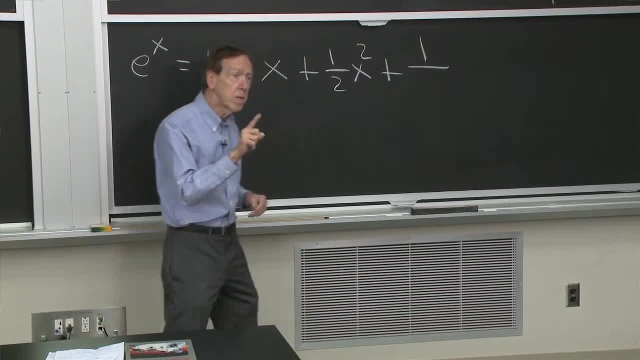 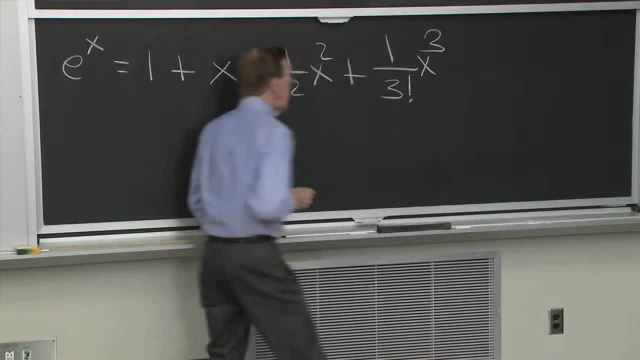 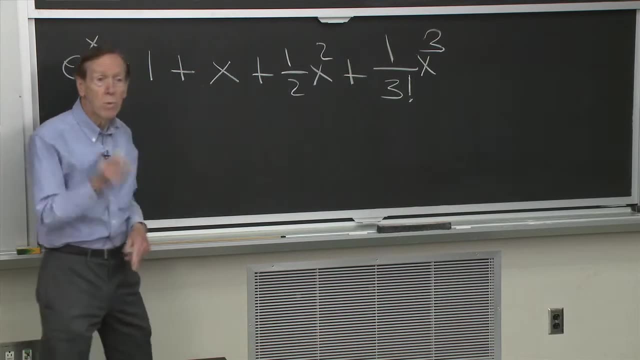 but I'm ready to see the pattern here. 6 is 3 times 2 times 1.. 3 factorial x cubed, This was that. 2 is really 2 factorial 2 times 1.. This 1 is 1 factorial. 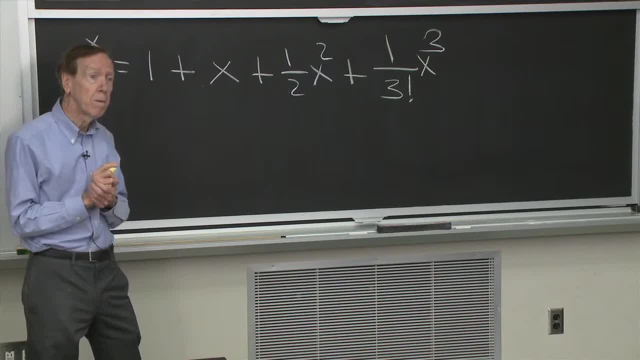 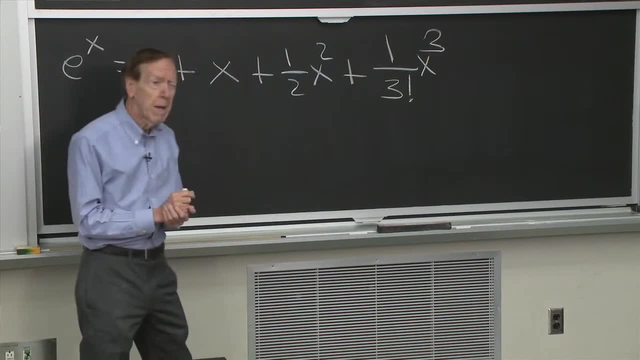 That 2 is 1 factorial. That 2 is 1 factorial. 1 is 0 factorial. 0 factorial is 1,, by the way, And I have to keep going. That's why algebra is not enough. I cannot stop. 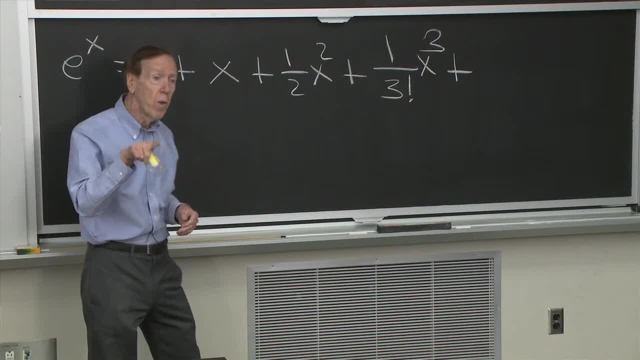 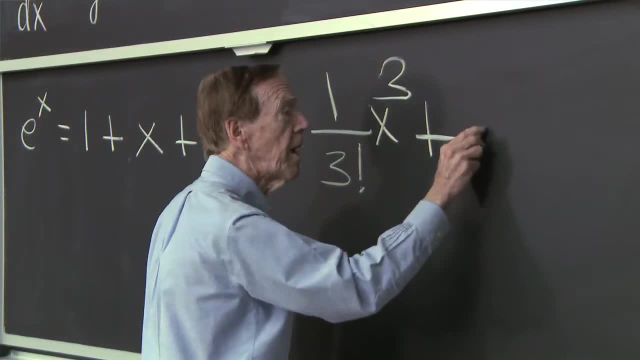 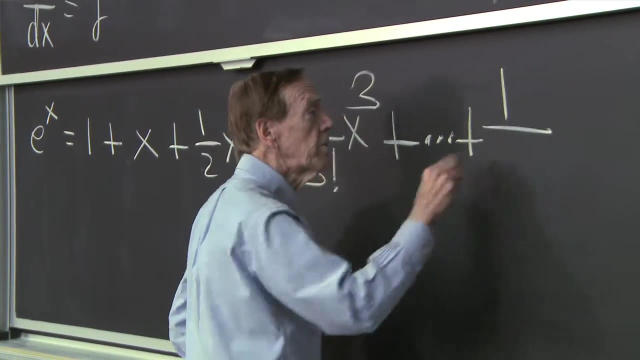 So the next term would be 1 over 4 factorial. 1 24th of x to the fourth and onwards. So can I use the three dots that mathematicians love to say: keep going. And then the typical term- So that is the typical term- is 1 over some n factorial. 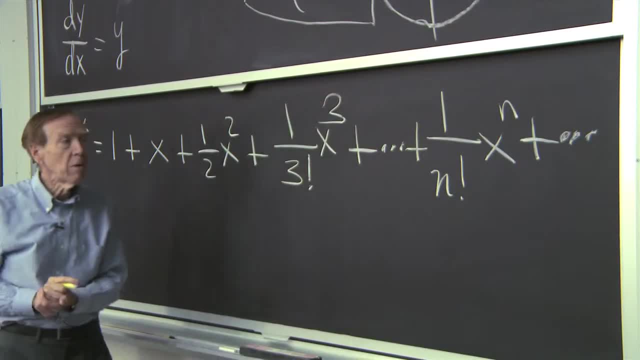 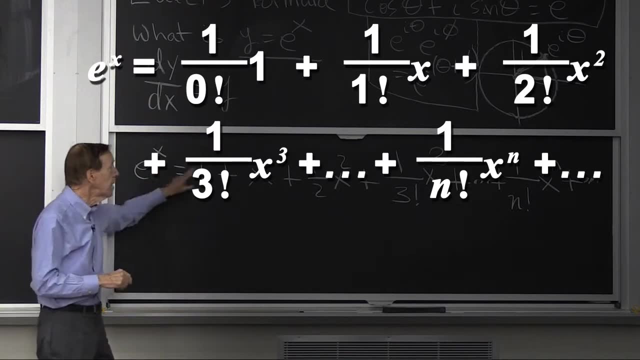 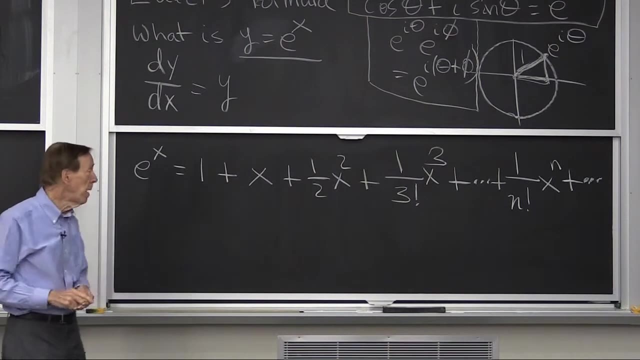 x to the nth and keep going. Those three dots are the key to everything. So that is my de-construction of e to the x. And now I'm ready for e to the i theta. I just take x to be i theta. 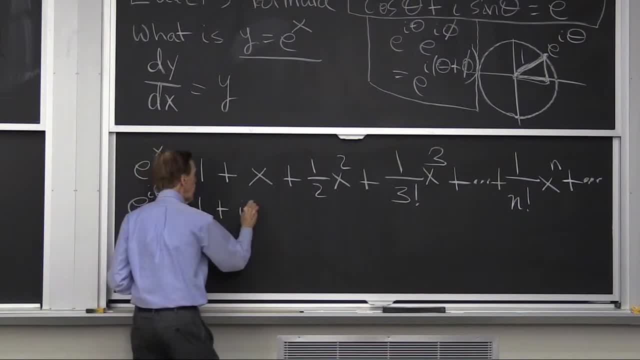 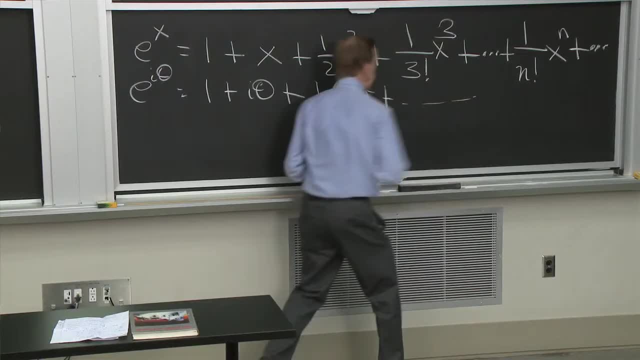 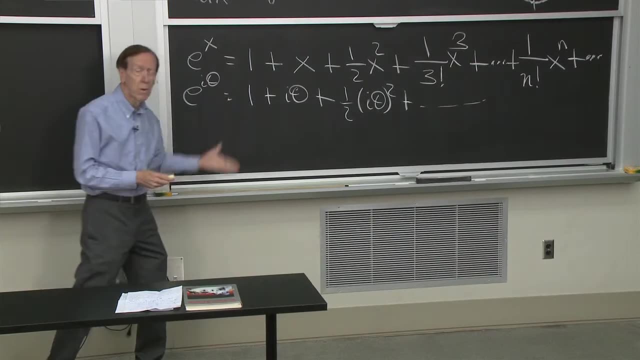 So e to the i theta is 1 plus i theta 5 times n over the seulphs, plus 1 half i theta squared and 1: 6, and so on. OK, now I'm ready for Euler. So now we know what one side of the equation is. e to the i. 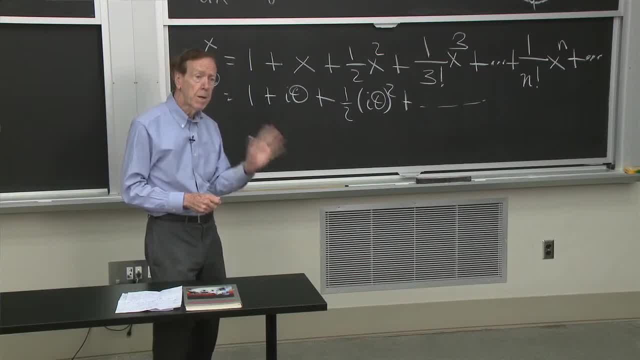 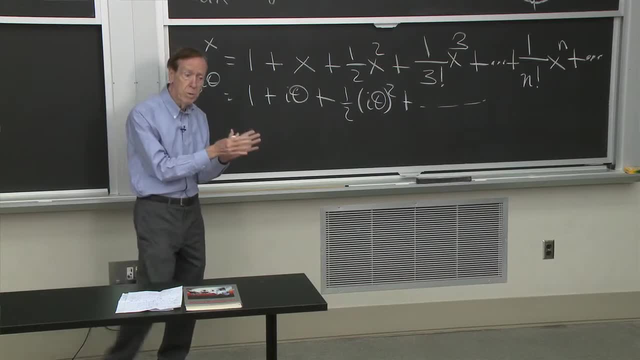 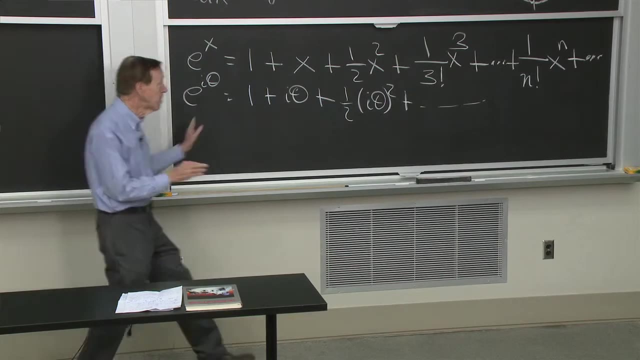 theta, The other side, cos theta plus i sine theta. I want to see those. So that's back to trigonometry. So can I write the formulas for cos theta and sine theta And you'll see that it comes together. Let me go one more term here, so you see it. 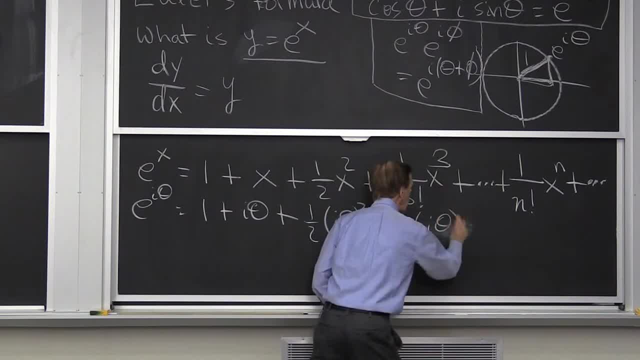 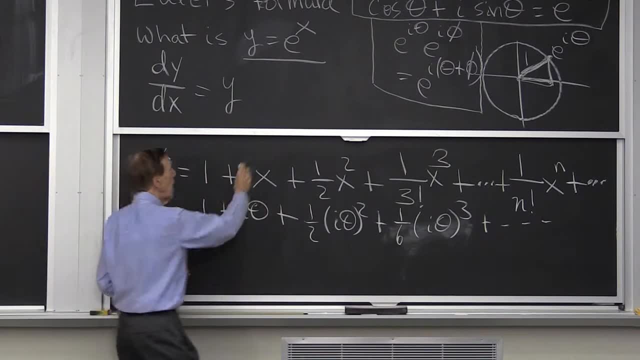 1, 6 of i, theta cubed and onwards. OK, now what Euler is telling me to look at, cos theta as the real part. So let me take the real part of this. The real part is the part without the i, so the real part is 1.. 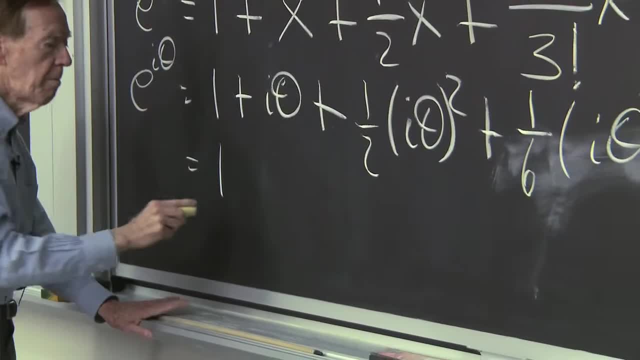 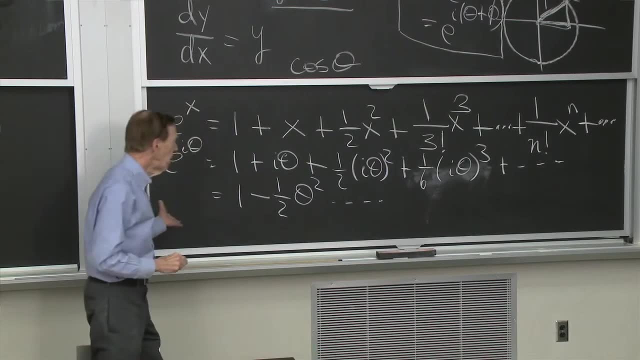 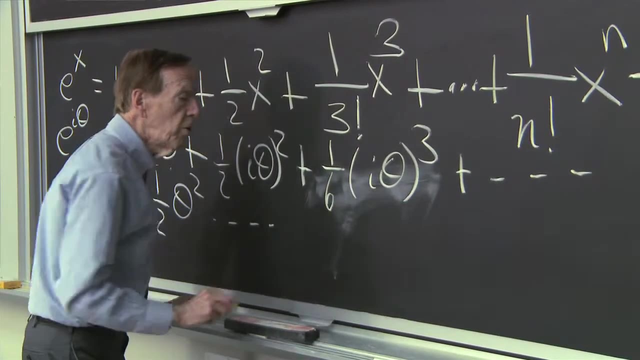 That's got an i in it, That has an i squared, so that's minus 1 half theta squared And then onwards. that's the real part And then the imaginary part. can I do the imaginary part? I have the i and the i cubed. 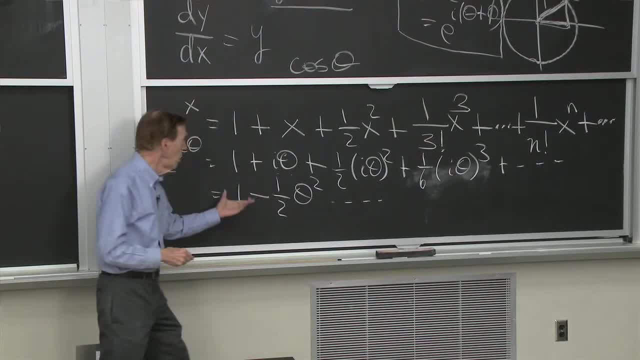 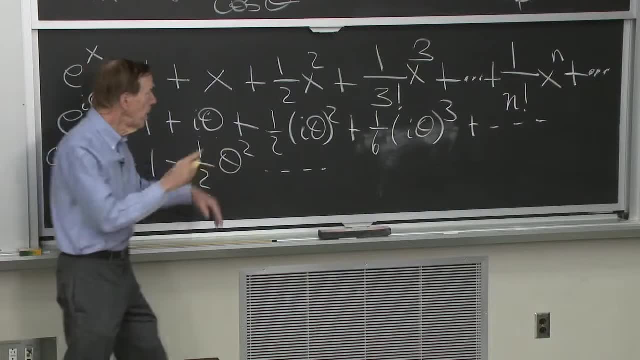 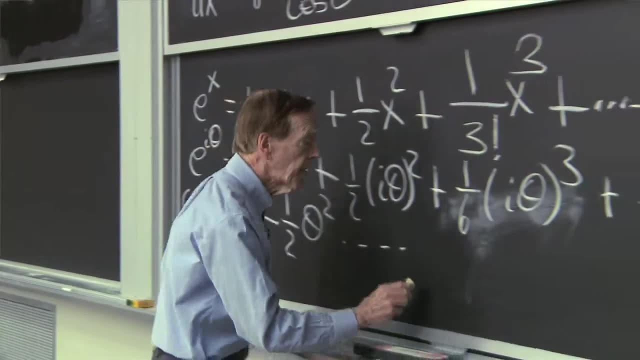 You see that the even powers are going to go in this part And that part is amazingly cos theta. The odd powers will have an i in them. They go into the imaginary part. So I have the imaginary part. is i times theta? 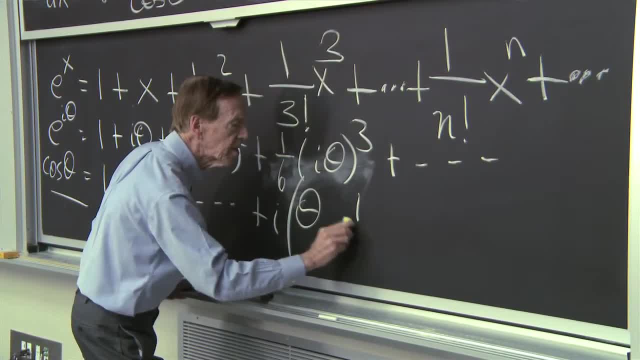 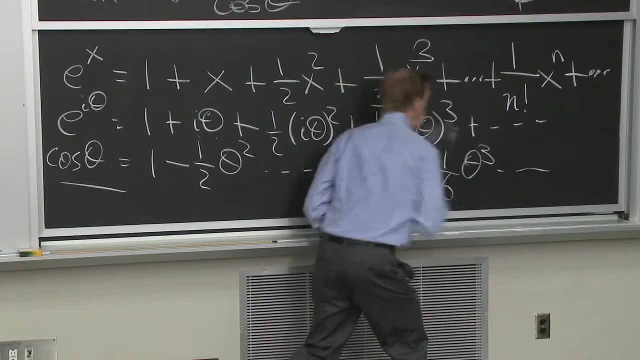 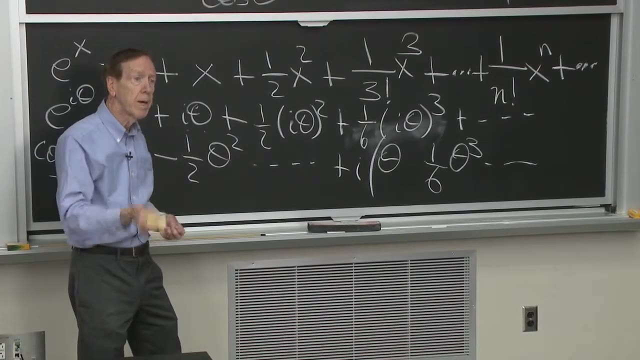 And how do I have it? This is 1 sixth of i cubed, theta cubed. OK, what's i cubed? What's the i cubed there i cubed is i squared times i, So that's minus 1 times i. 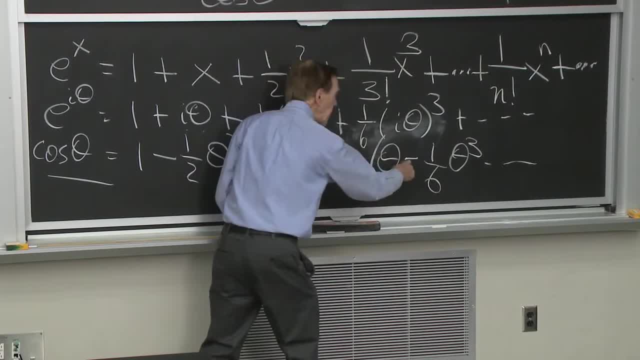 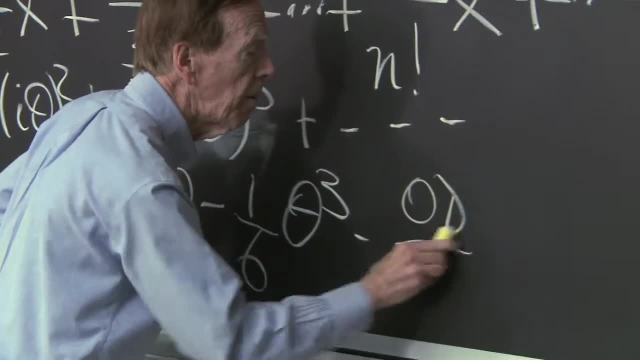 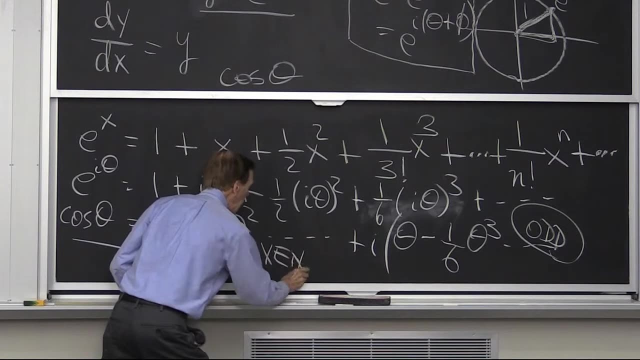 So I just need a minus there. I have an i Minus accounts for i squared And then the 1 sixth theta cubed and onwards. So this is the odd powers, This is the even powers, And the even part gives the cosine. 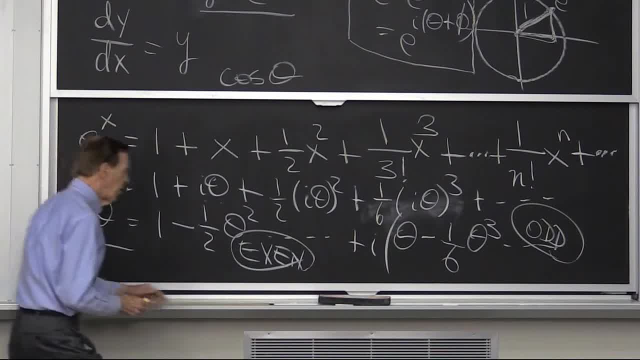 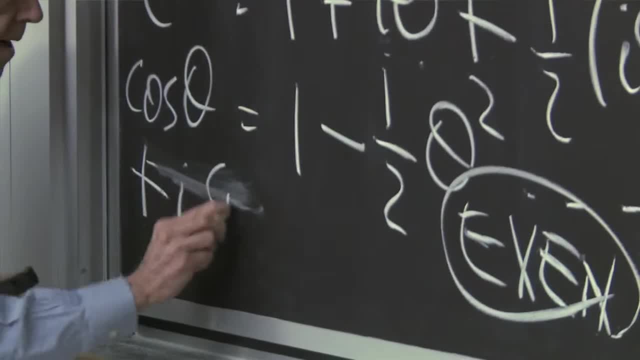 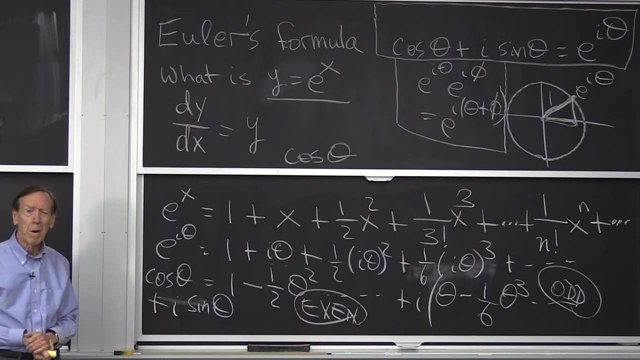 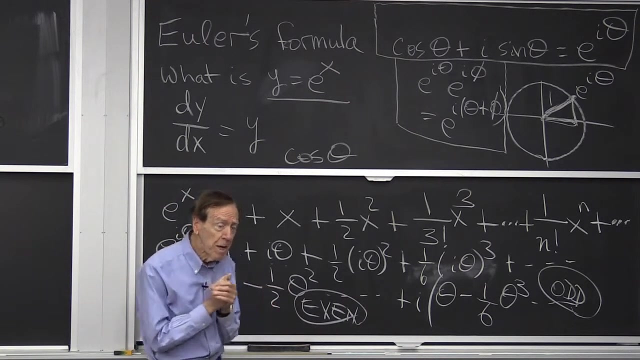 The odd part gives the sine. So let me make this formula all perfect. We're putting the two together: cos theta and i sine theta. OK, so that's my way of understanding Euler. That's my way of understanding Euler, And let me just ask you- I'll give you a few minutes. 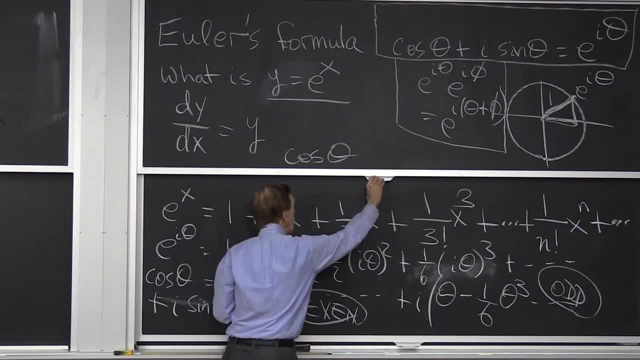 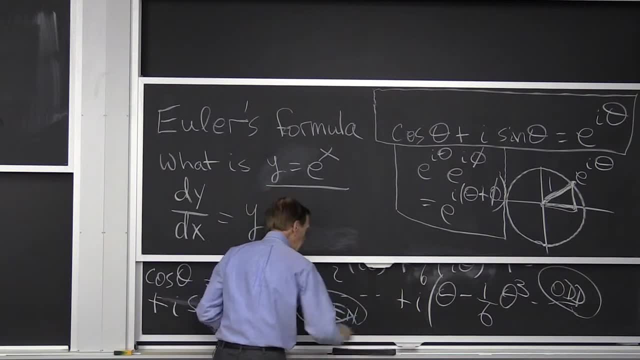 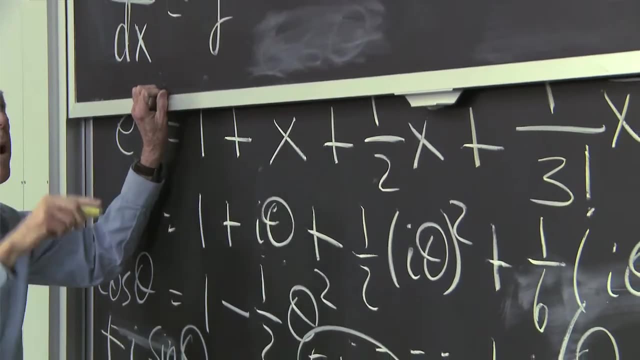 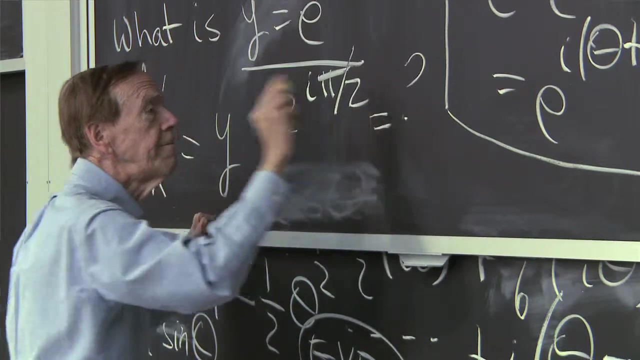 to do it. what about? could you figure out? what is this? What is this? What is this? What is e? If I take e and I plug in x, equal i pi over 2, e to the i pi over 2, equals what? 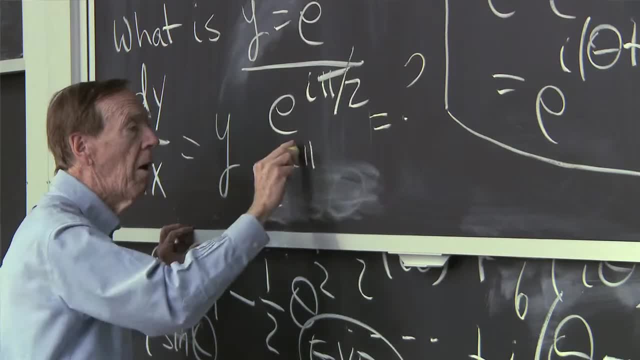 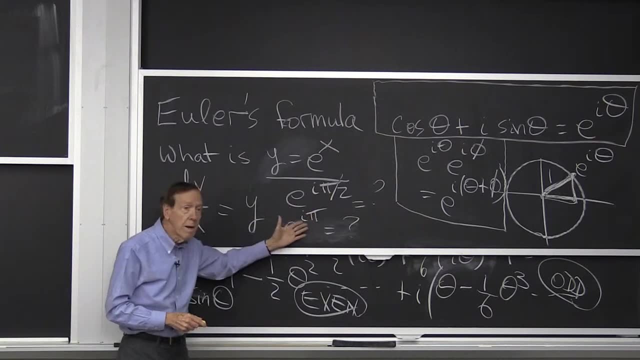 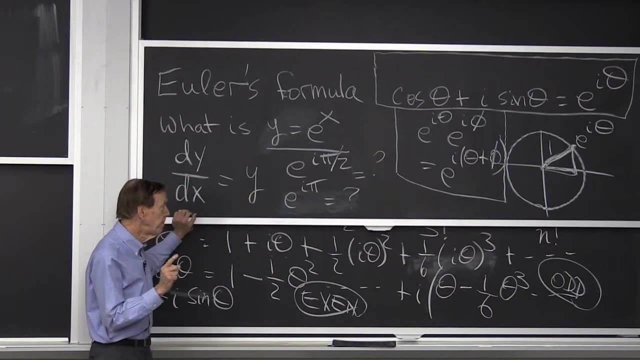 Or e to the i pi would be another one. OK, I'm going to ask you for these numbers Incredibly. they're simple numbers: e to the i pi. I'm not expecting you, even though I'll give you a little time. 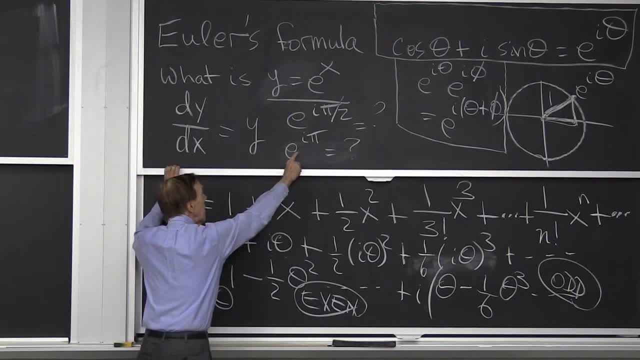 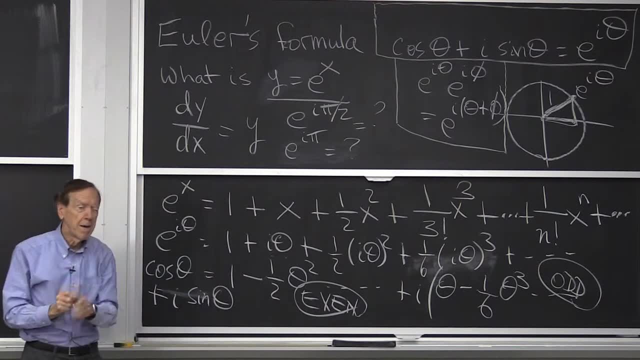 I'm not expecting you to put x equal i pi in there. That number is 1 plus i pi plus 1 half of i pi squared, and so on. But infinite series are beautiful to look at, but you don't want to add up all the terms. 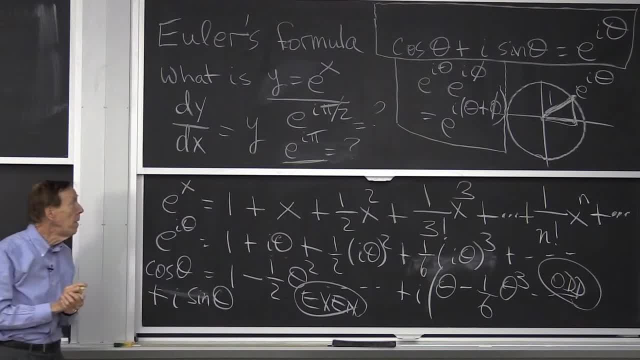 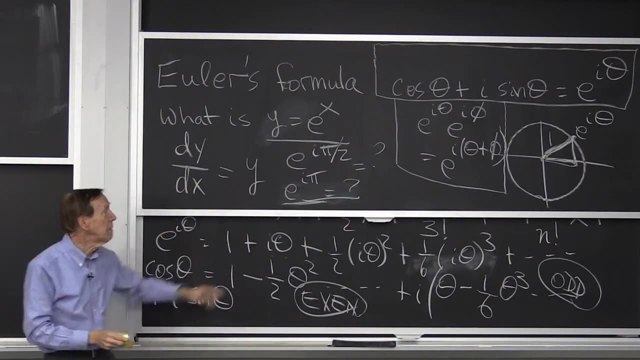 I want you to think about this as a complex, Complex number. The angle is pi, The distance, the magnitude r is OK, you can do it. You can do it, You can figure out what e to the i pi turns out to be. 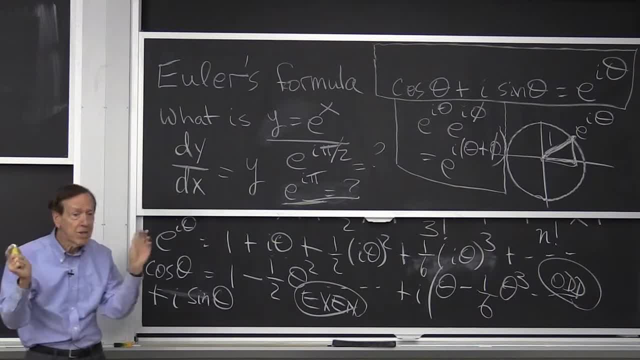 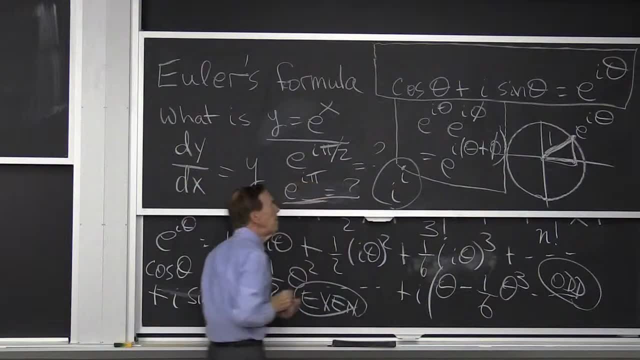 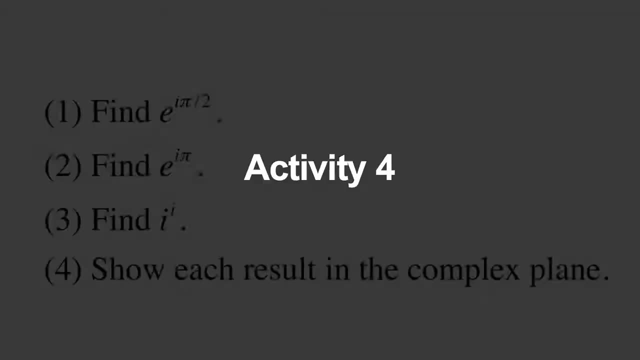 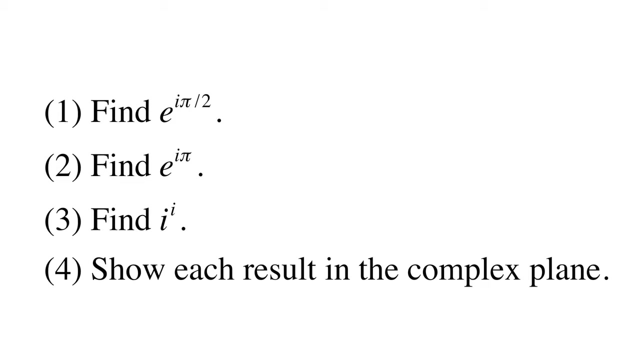 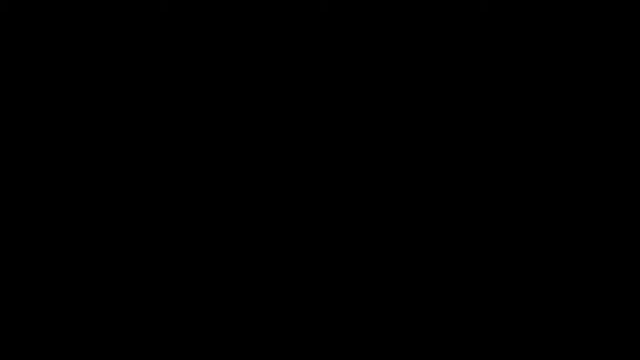 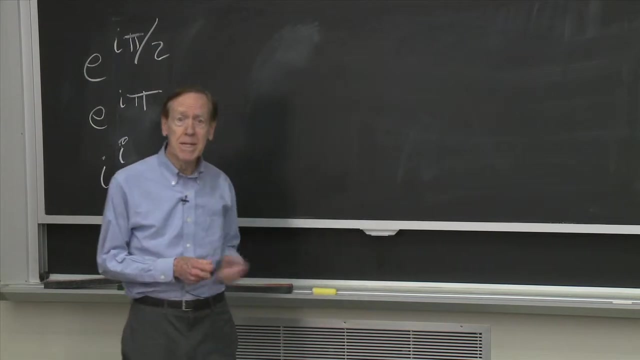 and what e to the i pi over 2 turns out to be. And then, if somebody is really weird or interested, what is i to the i? Oh, that's an amazing number. OK, thanks, Well, OK, I left you with three questions. 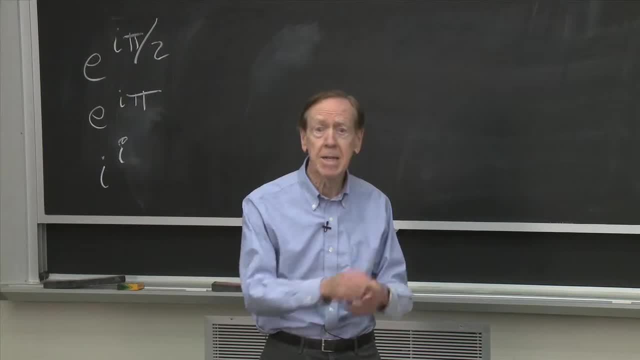 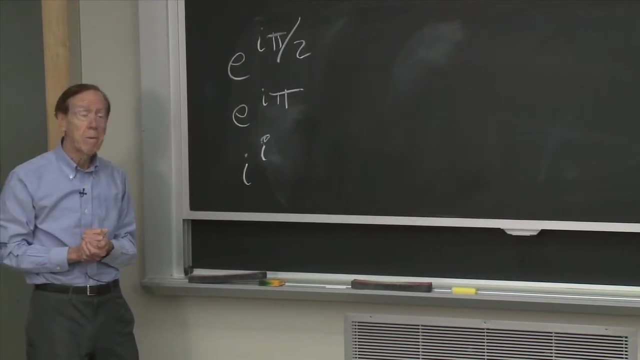 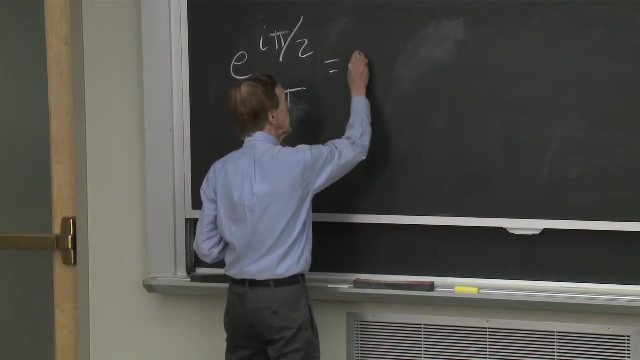 Let me make some comments on those and then tell you about a fantastic picture called the Mandelbrot set. OK, so my questions were: what are those three complex numbers? So how to do that? first one: OK, Euler said that this is the same as the cosine of pi over 2. 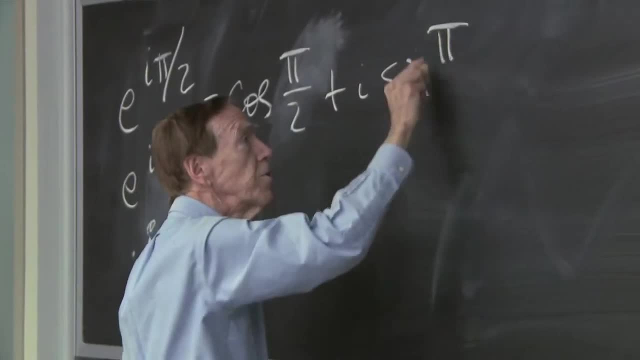 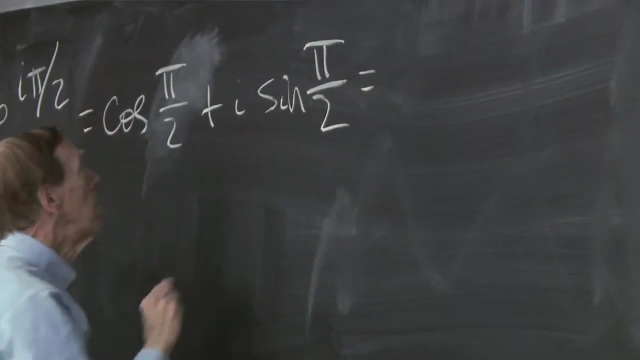 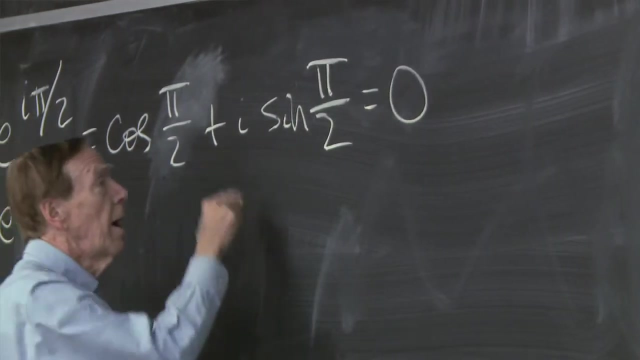 plus, i times the sine of pi over 2.. And those are things that we know. That's 90 degrees, The cosine of 90 degrees is 0. And the sine of 90 degrees is 1.. So I have i. 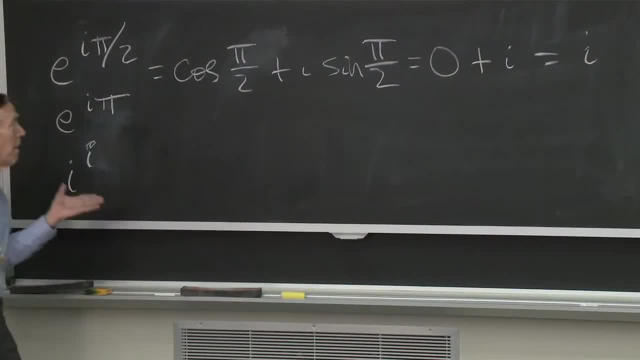 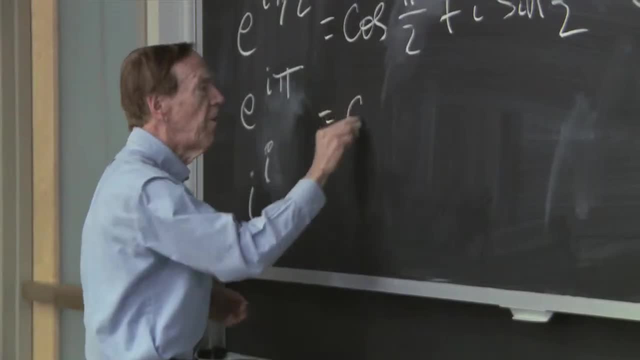 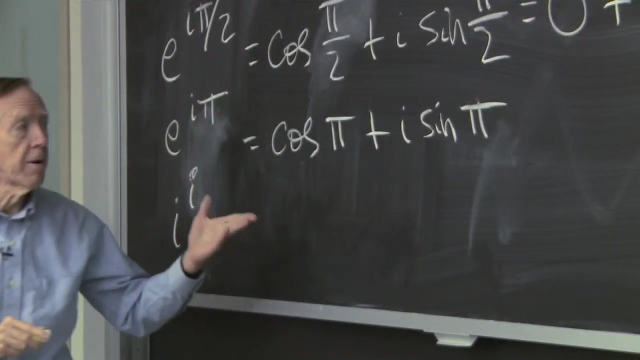 The answer to that question was an amazing number: e to the i pi over 2 equals i. What about e to the i pi? OK, if we follow Euler again, that's cosine of pi plus i, sine of pi, 180 degrees. the cosine has dropped to minus 1.. 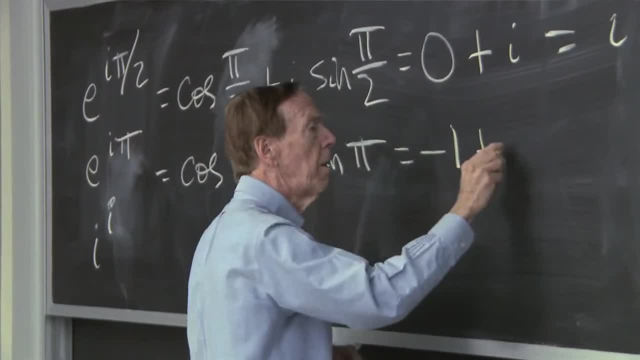 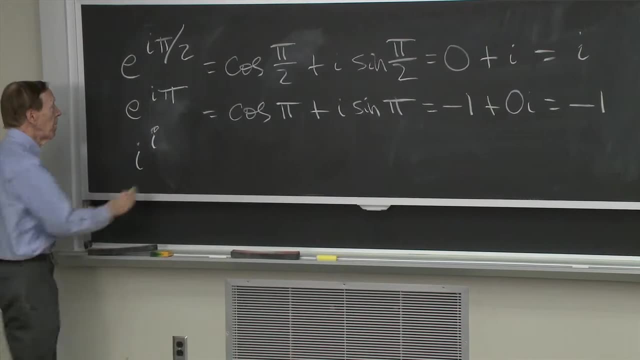 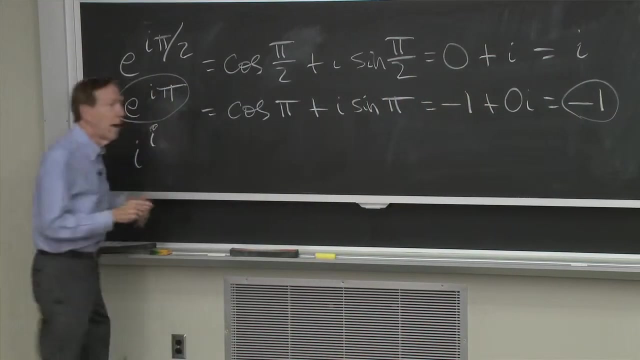 The sine of 180 degrees is 0. And I get minus 1.. A lot of people think this is a wonderful formula. e to the i pi is minus 1.. If I put the number i pi into that infinite series and add it up, you won't see it happen. 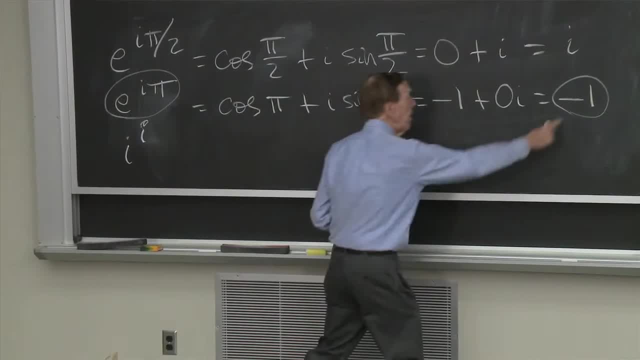 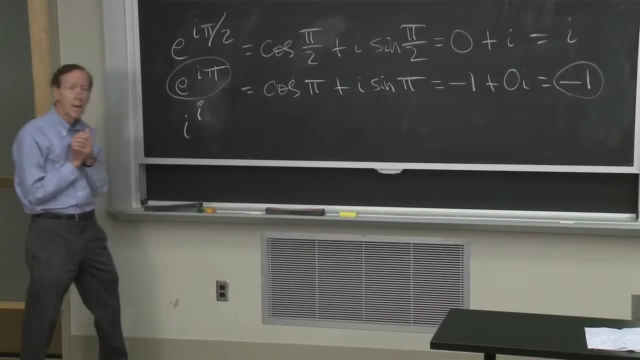 But somehow, at the end the whole thing adds to minus 1. And now This was a crazy one for teachers, for professors. What could i to the i be? What sense can I make of it? Let me suggest a way to do it. 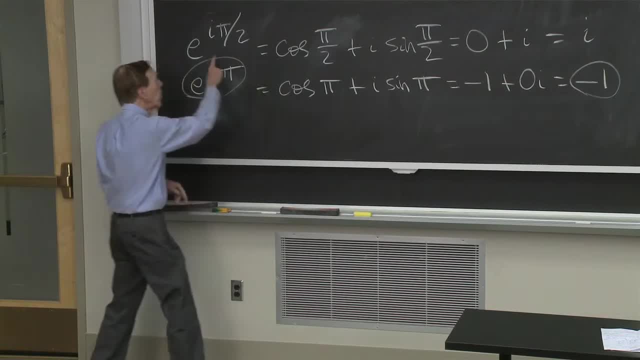 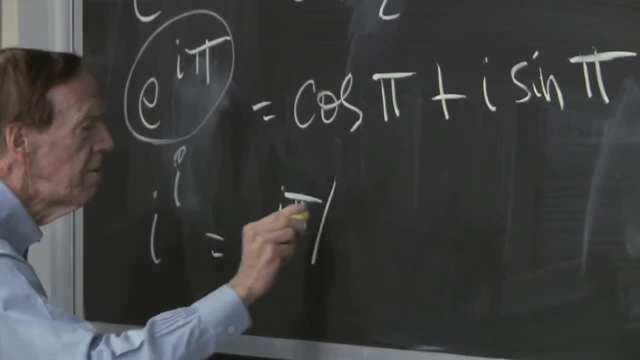 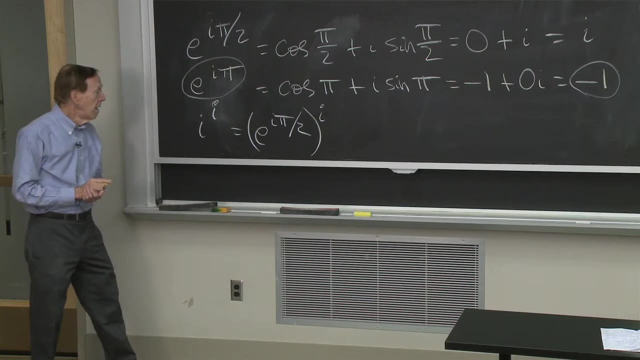 That i is, according to our first formula, e to the i pi over 2.. So that i is e to the i pi over 2.. Thank you, Euler. To the power i Now. Now I've got something I can work with. 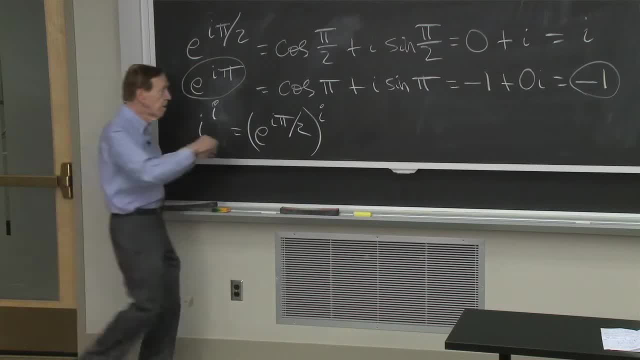 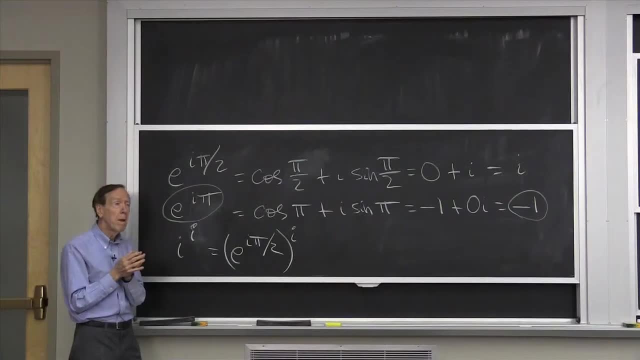 Do you remember what the rule is for exponents when you take a power? If you took x, cubed to the fourth power, that would be 3x's times 3x's times 3x's times 3x's, 12x's x to the 12th. 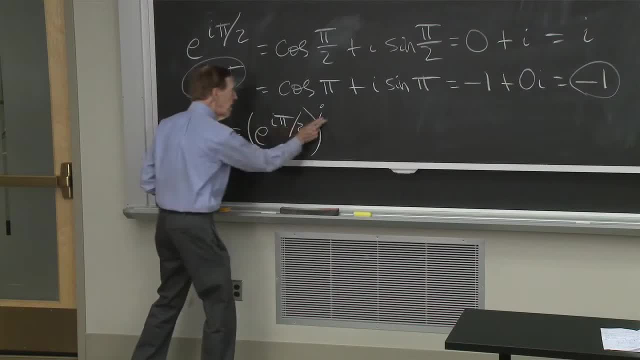 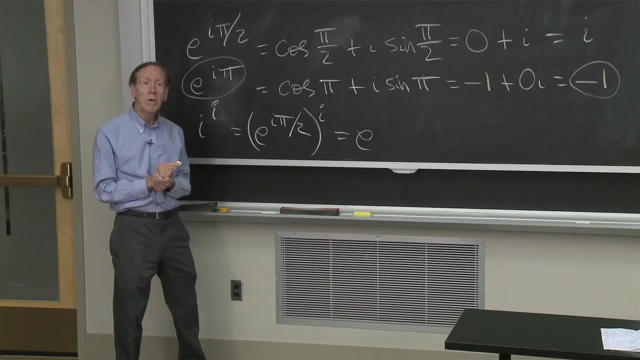 You multiply the 3 and the 4.. Here I multiply those guys, So it's e to the i times i, So it's 2x squared over 3.. Give me the number: is i pi over 2, which is minus pi over 2.. 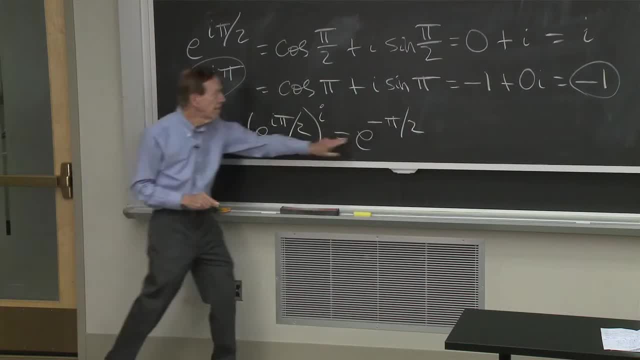 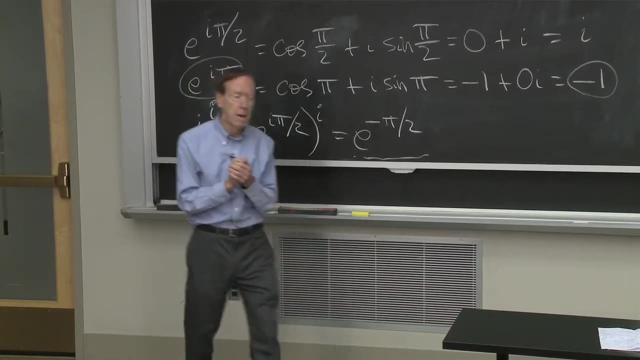 Look at that i to the. i has come out to be some real number And I don't actually know what the digits are. You'll find them Anyway. that's the amazing answer to i to the. i Now for the Mandelbrot set. 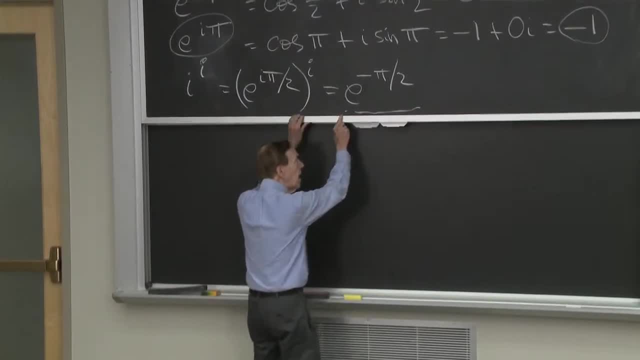 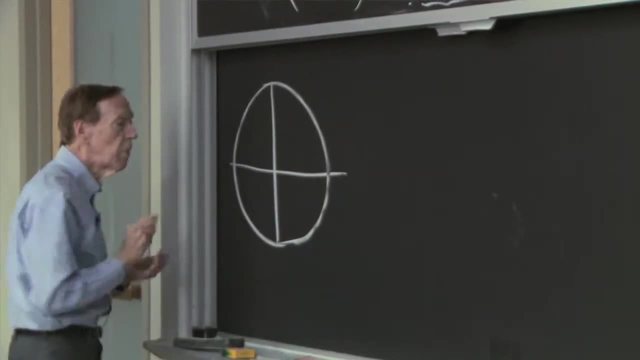 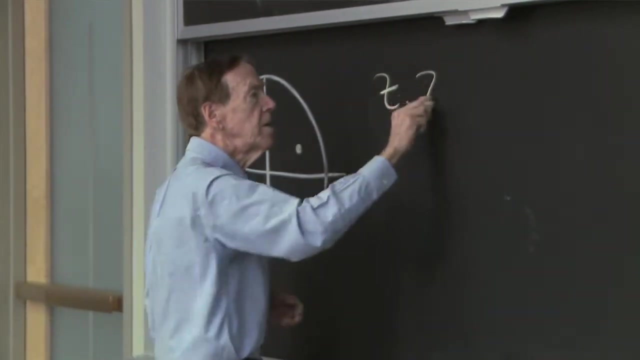 Can I first ask a question to lead into the Mandelbrot set? Remember the complex plane, Remember the unit circle, the things of size 1.. Suppose I start with a complex number there, Start with z. Look at z, z squared, z, cubed forever. 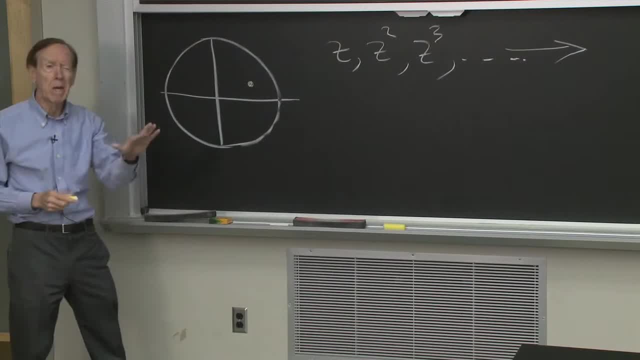 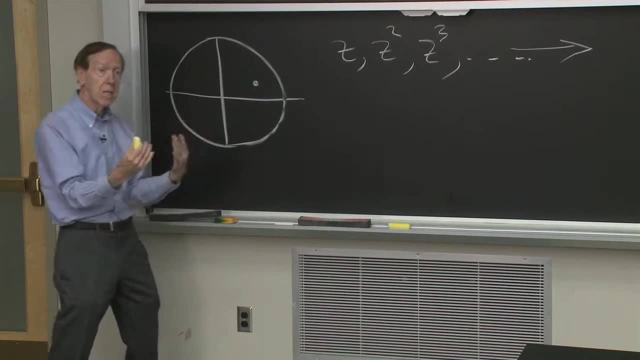 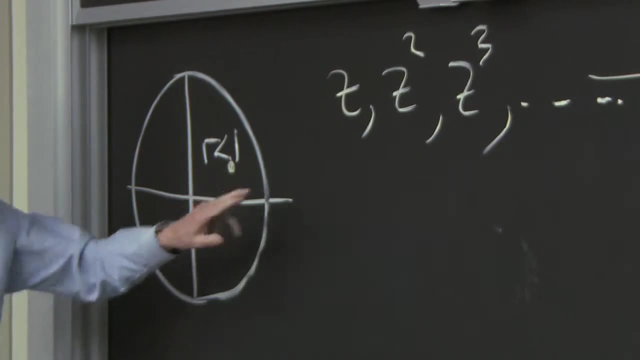 What do I get in the limit? So I take that number z. The point about that number z is that it's inside the unit circle. What does that mean? It means r is less than 1 in here. Then what about z squared? 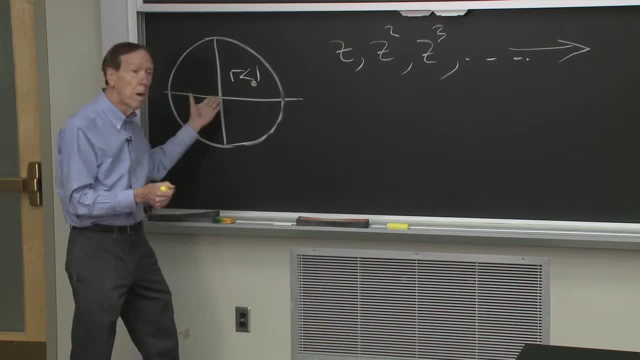 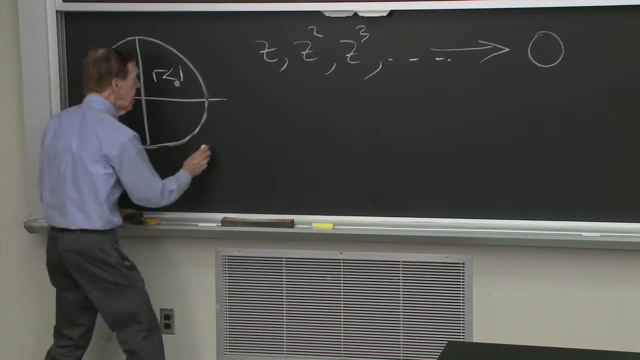 z squared, the magnitude of z squared is r squared. The magnitude of z cubed is r cubed. And with r less than 1, those numbers are getting small. My conclusion here is that that goes to 0.. Suppose I take instead a number out here. 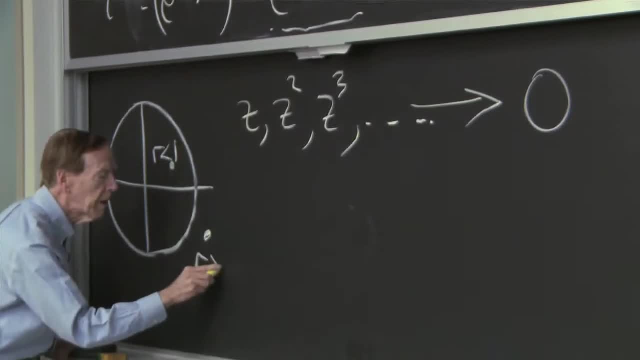 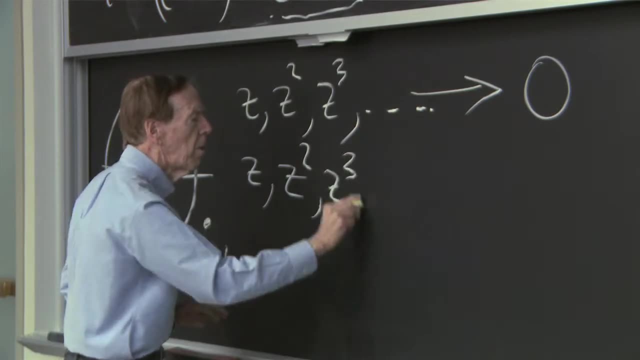 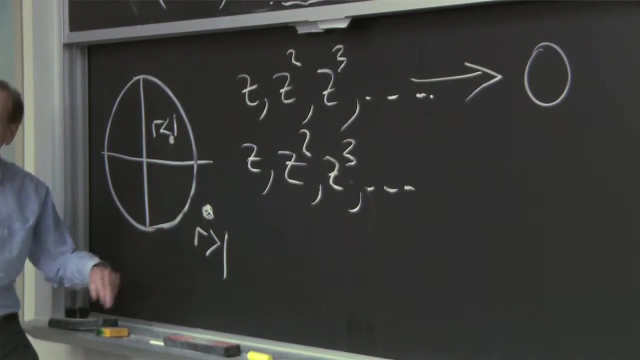 That'll be my second number Out there, r is bigger than 1.. Now I do z z squared, z cubed, so on, What's happening here? When I multiply that number by itself, the r's will multiply to give r squared. 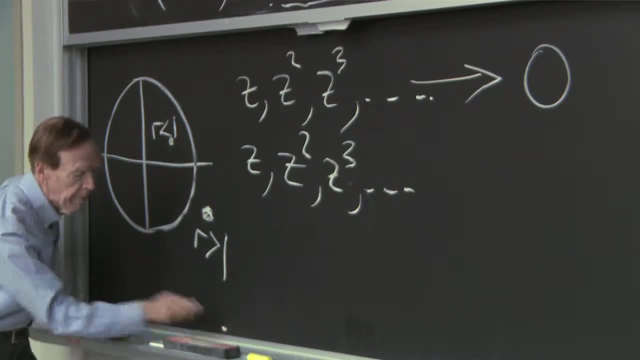 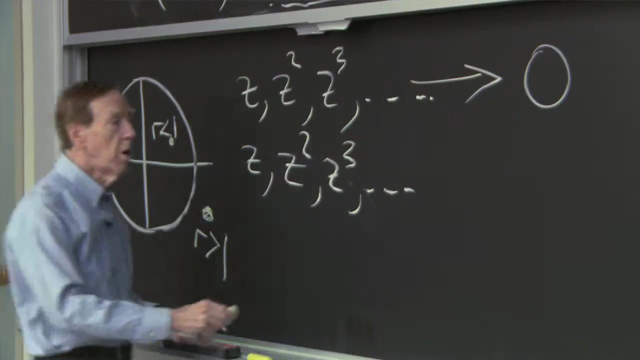 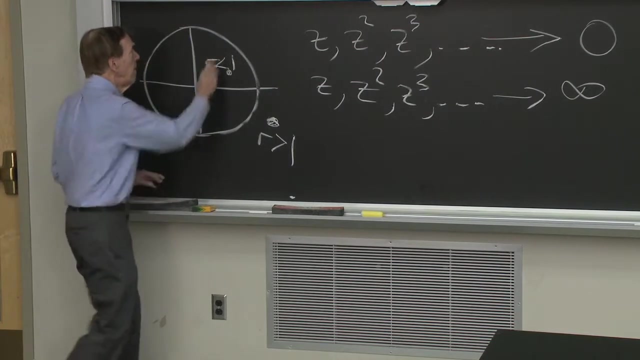 The angles will add, so it'll be a number down here. It'll be about there. That'll be z squared, z cubed will be further out. This will go to infinity, And points on the circle. Now let me take a point on the circle. 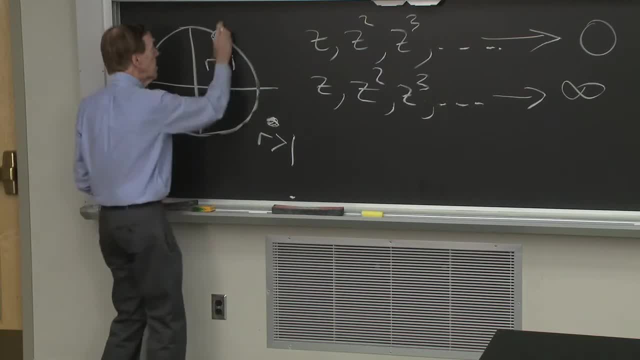 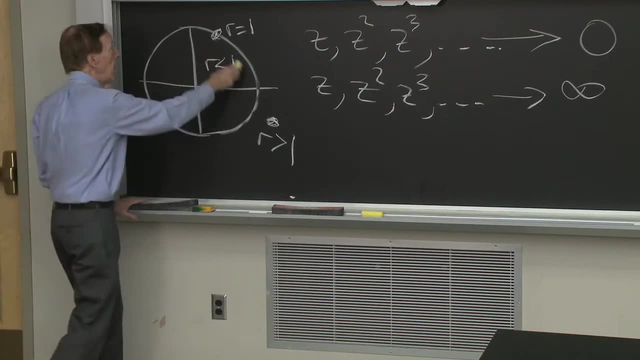 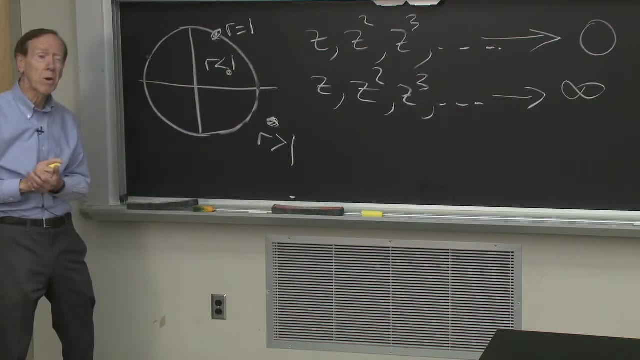 What happens to those? If that's my, this is r equal 1 on the circle. The square of that is on the circle, again at twice the angle. The cube is three times the angle, four times the angle, So I'm running around the circle. 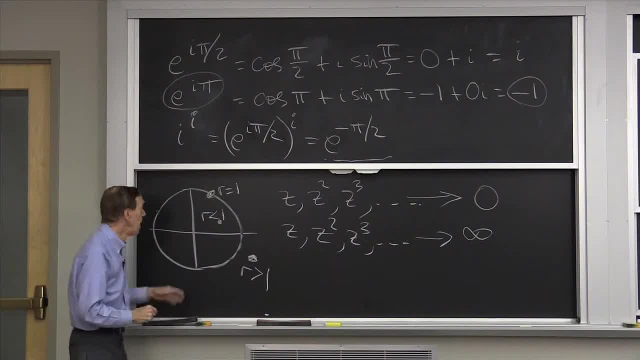 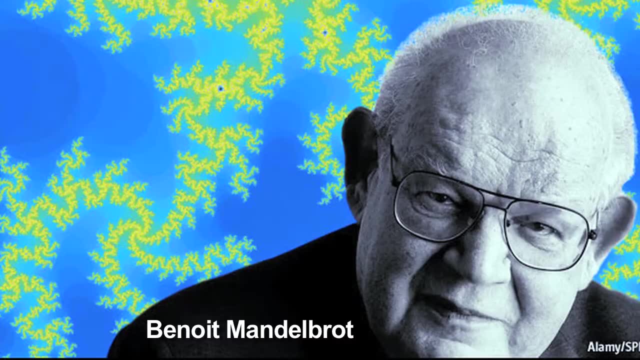 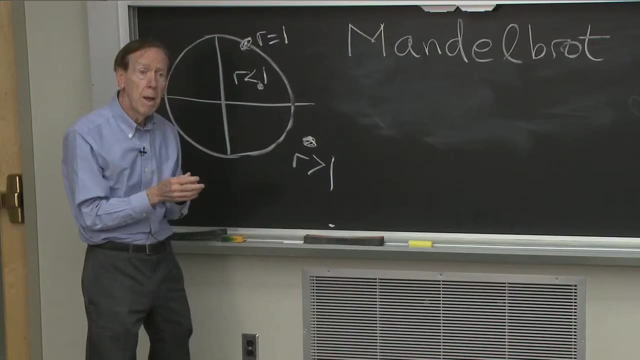 I'm running around the circle, or jumping around the circle when I take powers of that one. All right now for Mandelbrot. Mandelbrot had a fantastic idea. This Mandelbrot set is going to be a part of the complex plane. 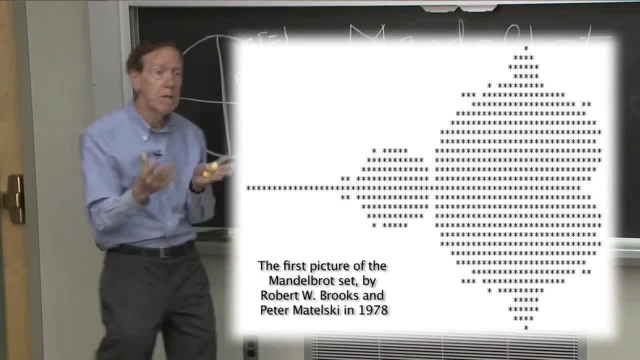 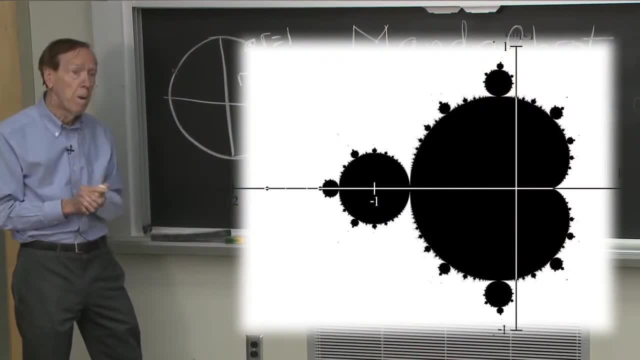 It won't look like a circle. It has a very, very strange shape, which you'll have to see with a blown up picture. What I want to do is the math part, to tell you where did that Mandelbrot set come from? 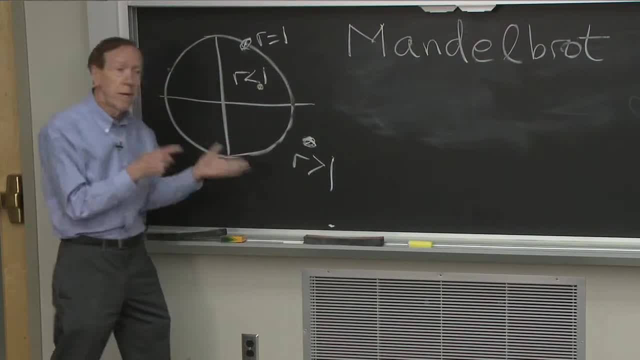 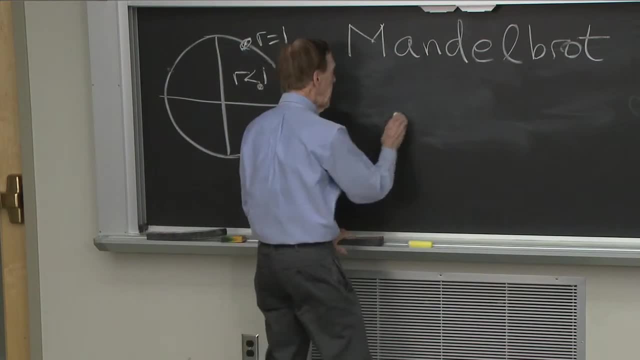 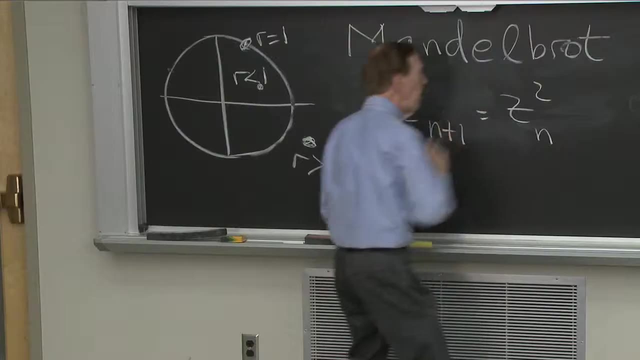 So you remember, with what we did. first, I took a number, I squared it, square, that square, that square. that Mandelbrot had the idea: let the n plus first one be the square of the nth one. So if he stopped there, we're just. 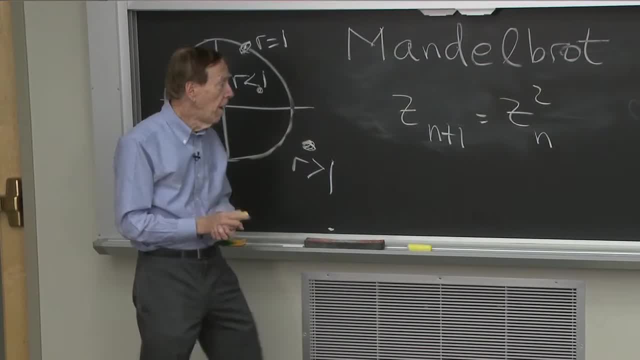 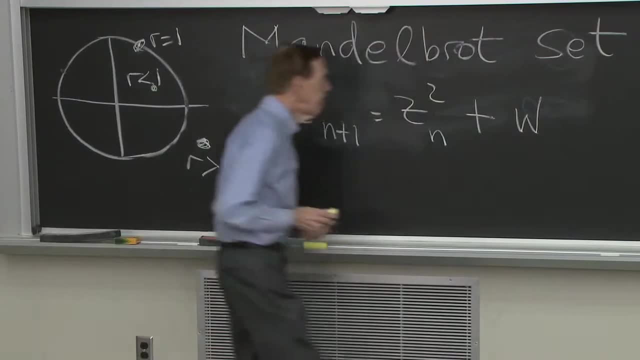 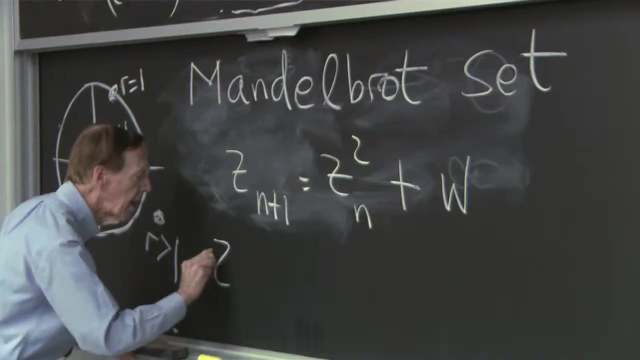 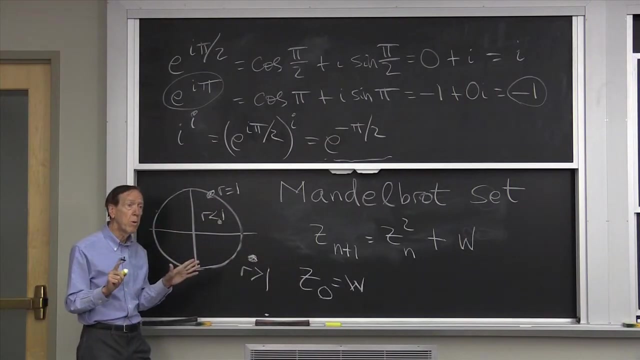 taking powers of the original z0.. But you're going to add in a constant say w. That'll be another complex number, OK, and I have to start this thing with z0 at w, OK, so here's the question that Mandelbrot asked himself. 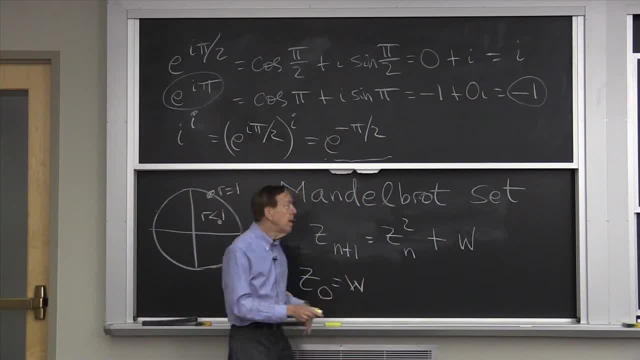 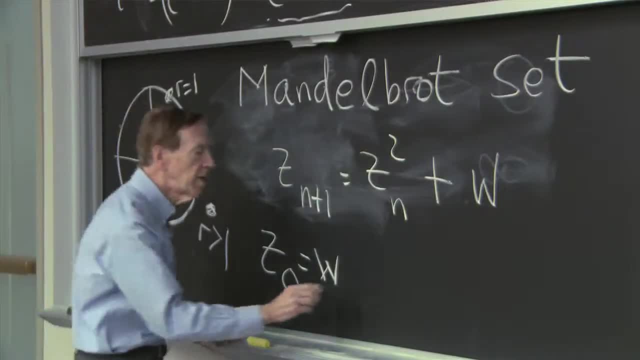 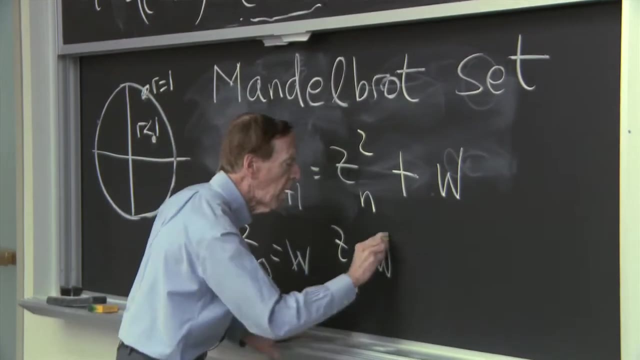 If w is some complex number, anything in the complex plane, I start z0 at that number w. then what is z1?? z1, I take one step- is z0 squared, that's w squared plus the w. OK, 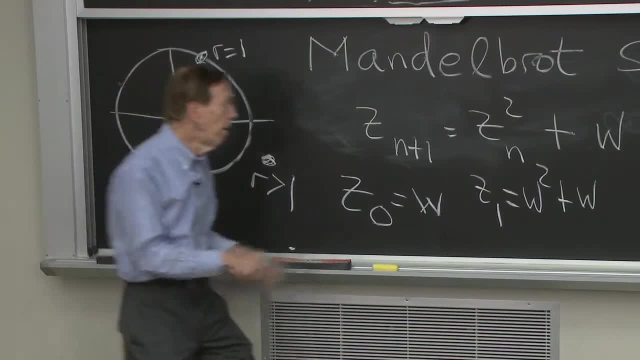 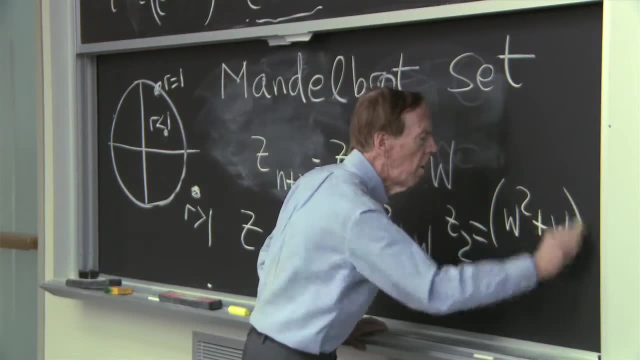 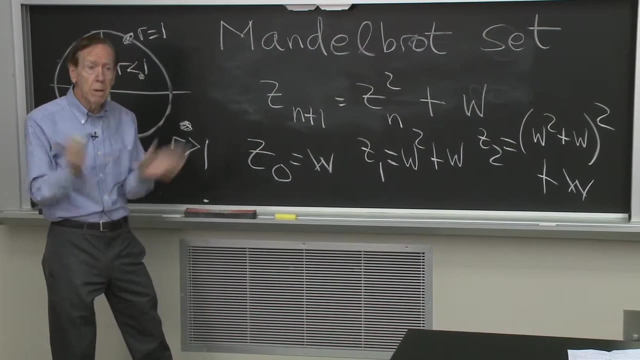 That some other complex number, Maybe bigger, maybe smaller, z2 will be that number squared w, squared plus w, all squared plus 1 more w from there. Right, I just keep going in theory And I ask the question. 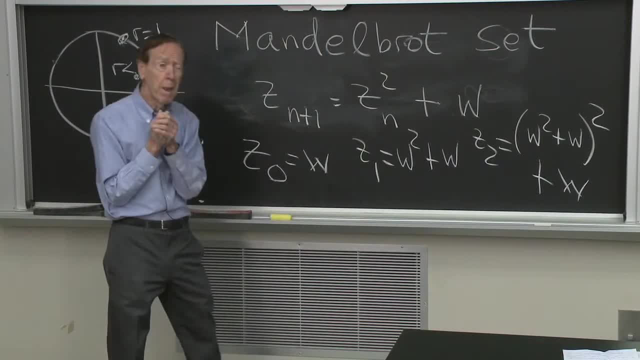 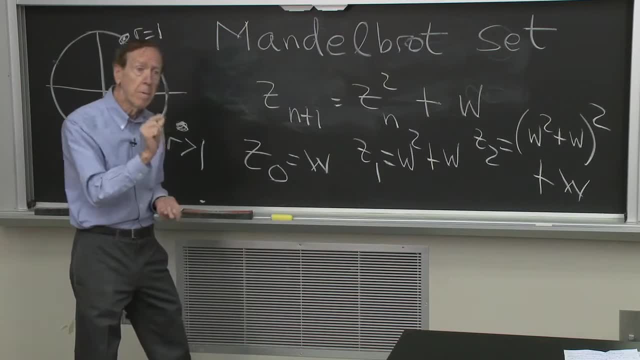 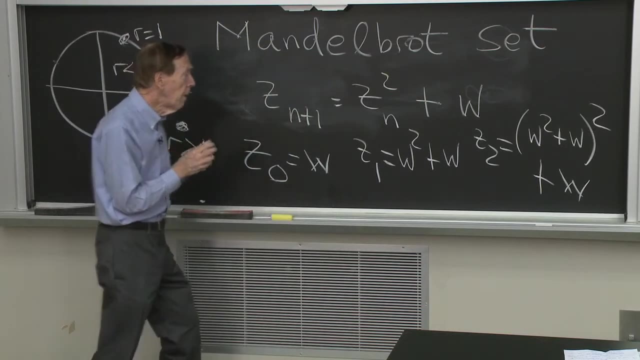 Yes, Sure, Do these numbers blow up or not? If they don't blow up, I put w, that complex number, in the Mandelbrot set. I put w in the Mandelbrot set. So let me do an example. 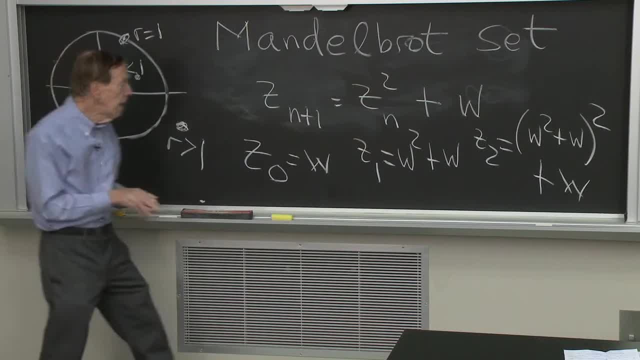 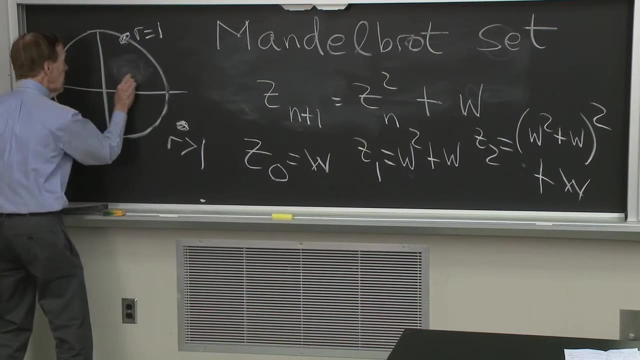 Suppose w is a pretty small number, Then I start small. That doesn't add much. That doesn't add much. If w is small, it's going to be in the Mandelbrot set, All right. so let me put a w. 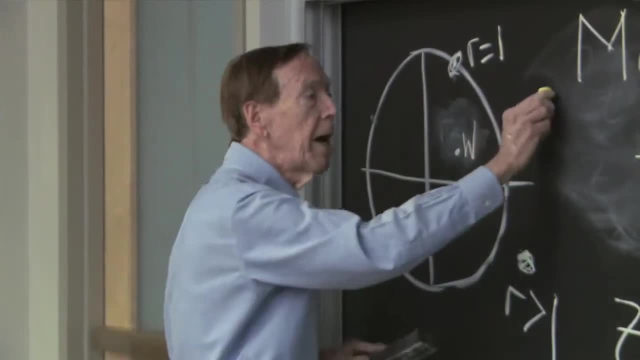 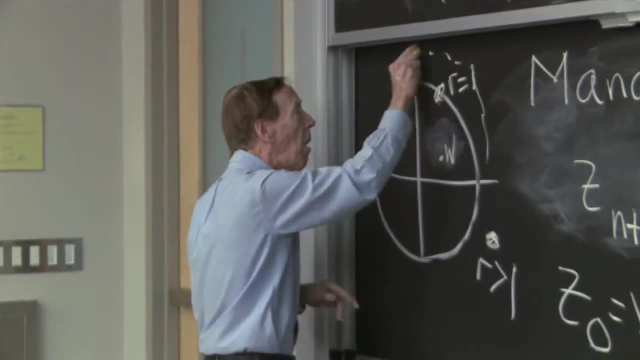 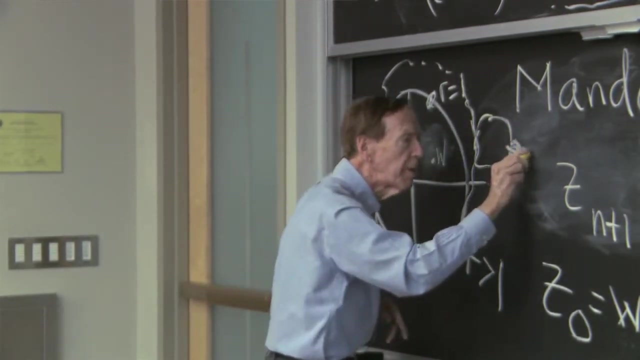 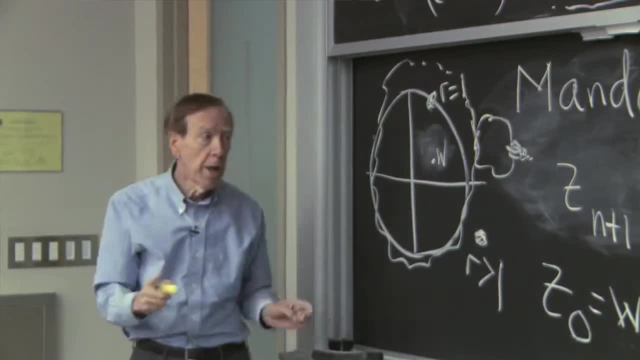 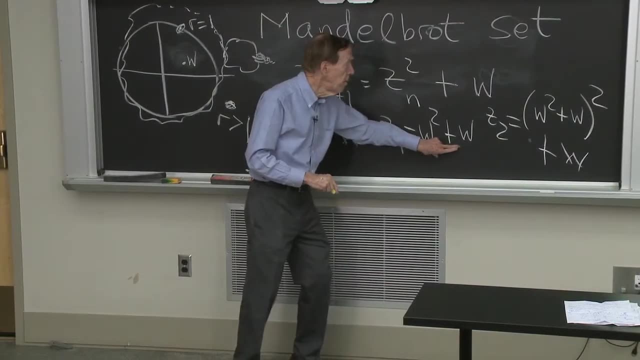 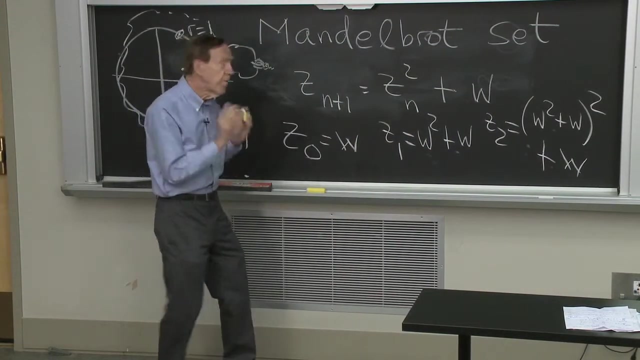 contains a set of numbers. So I put all the w's so that if I start with w, go to w squared plus w, go to that squared plus another w, go to that squared plus another w and keep going. if w is in this set I don't blow up. 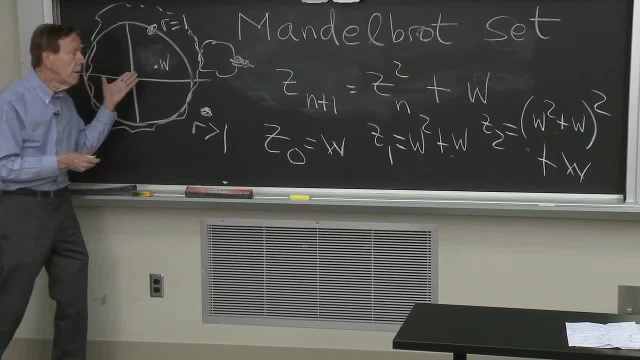 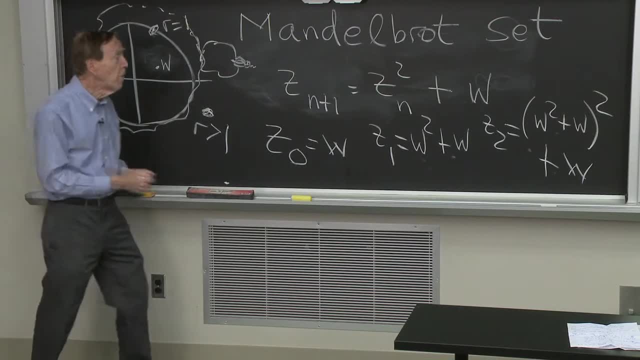 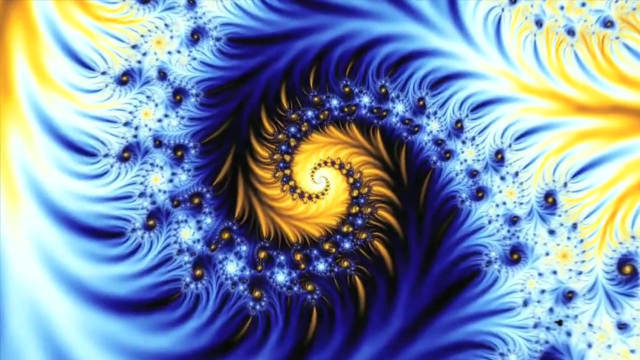 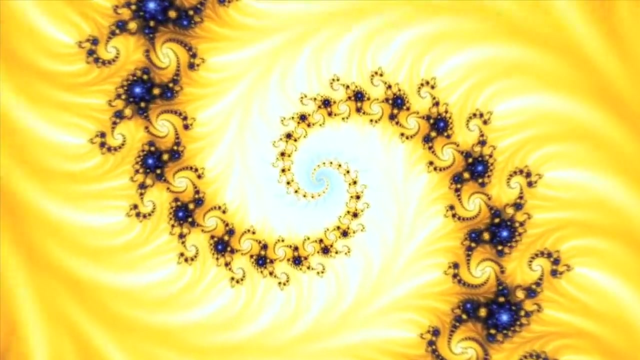 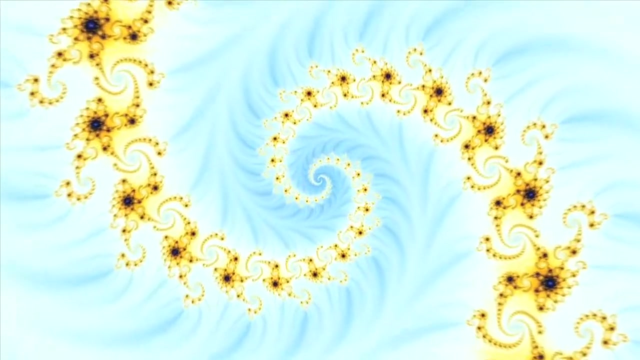 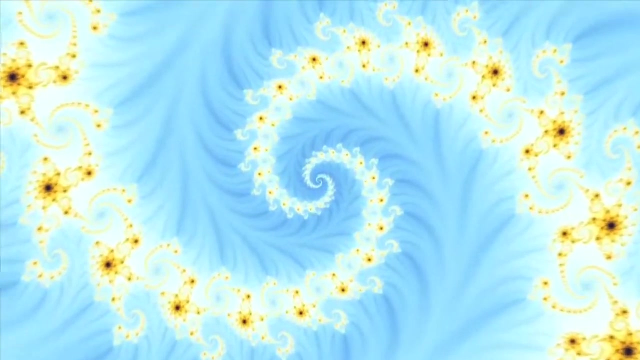 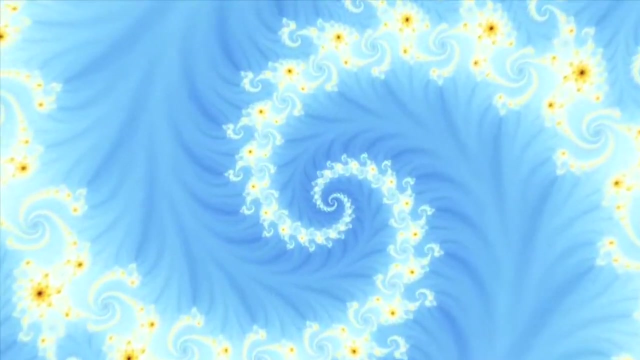 So w the Mandelbrot set is all the w's that stay bounded when it's a little bit crazy iteration on them. OK, you'll have to see a picture of that. That comes next. Thank you … … … …. 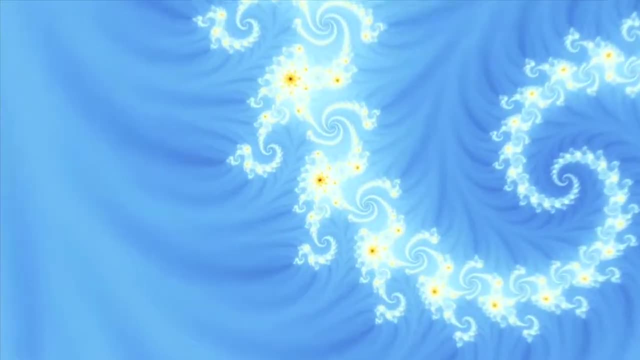 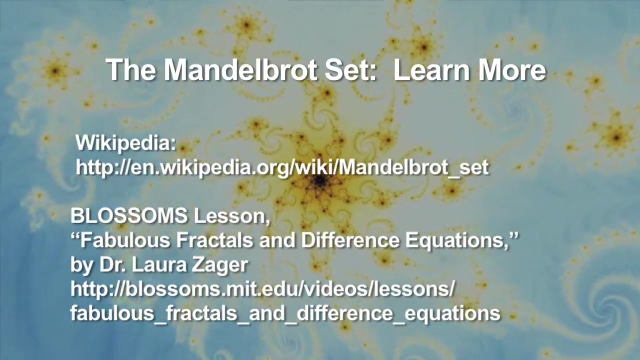 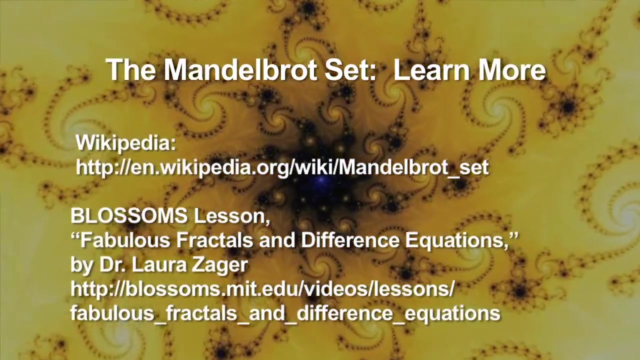 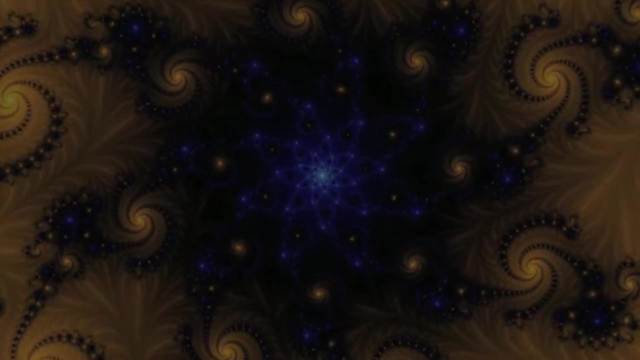 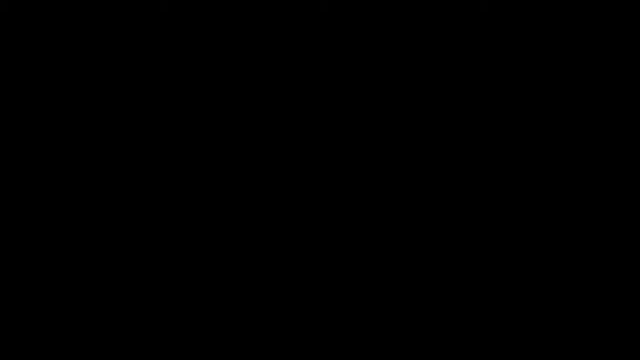 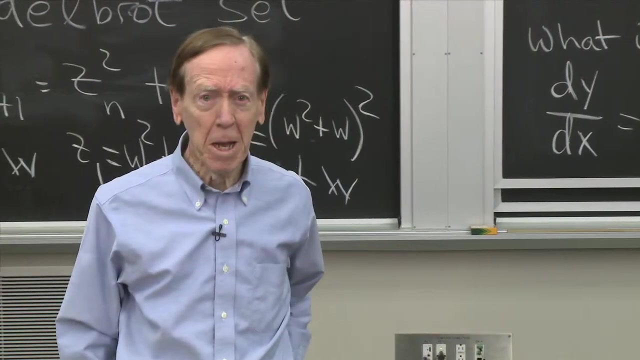 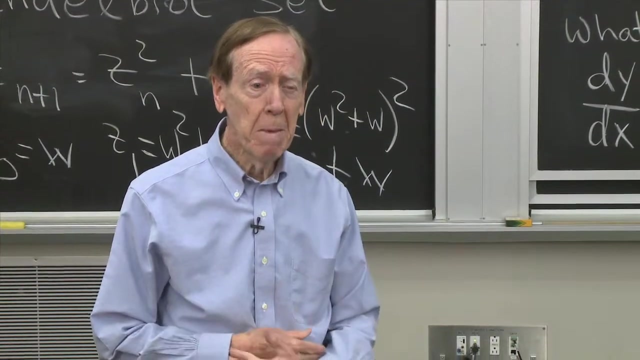 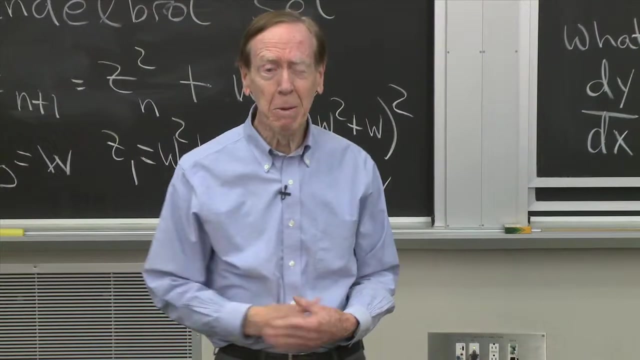 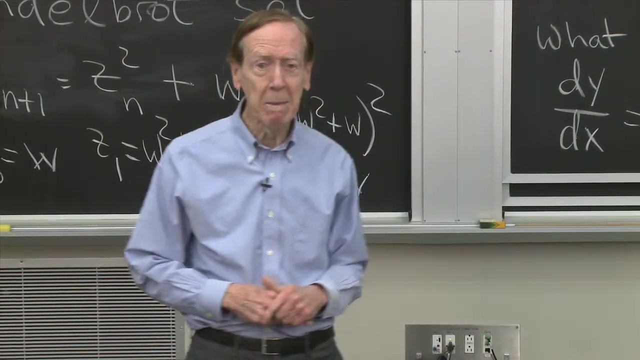 … … … …. Hi. Well, thank you for being part of this complex number presentation and your students. So I've been teaching at MIT for quite a while. Complex numbers come into it. Not everybody knows Euler's formula when they arrive at MIT. 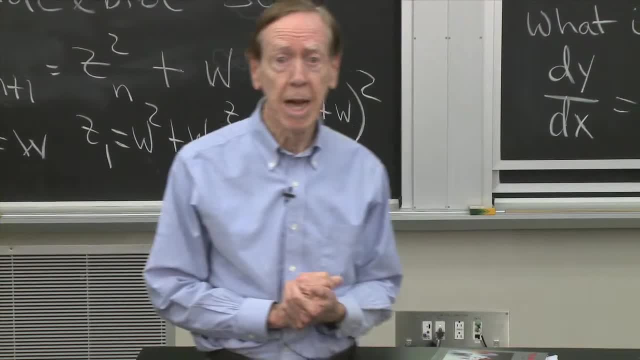 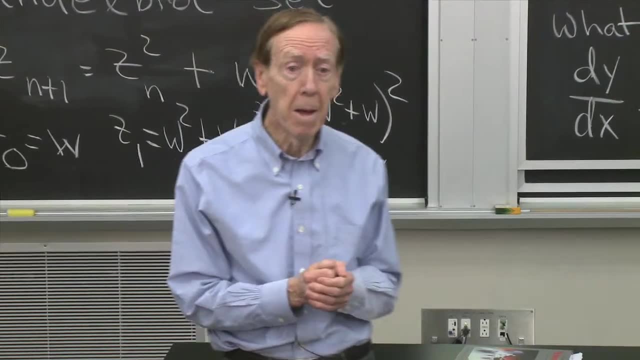 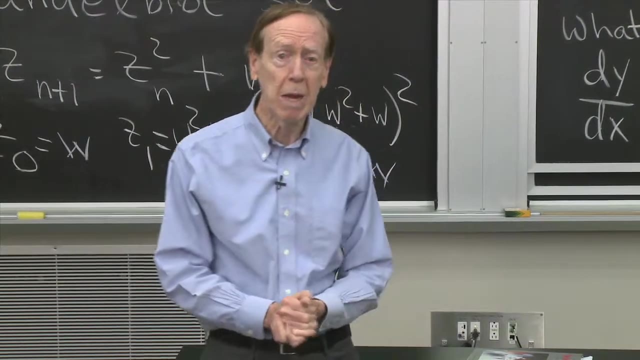 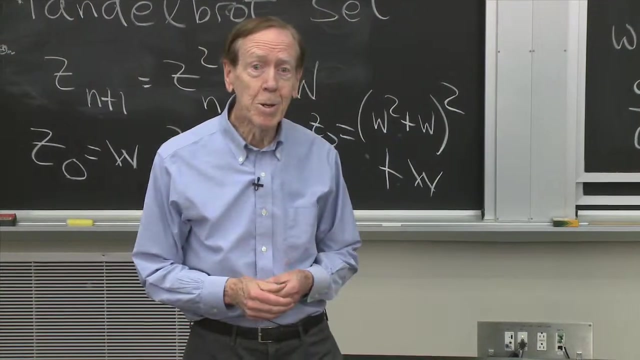 And then my part is more matrices and linear algebra, linear equations. So that's on OpenCourseWare. But the quadratic, The blossoms on the quadratic equation. I hope your students would like that. My objective in this blossom was to open up.